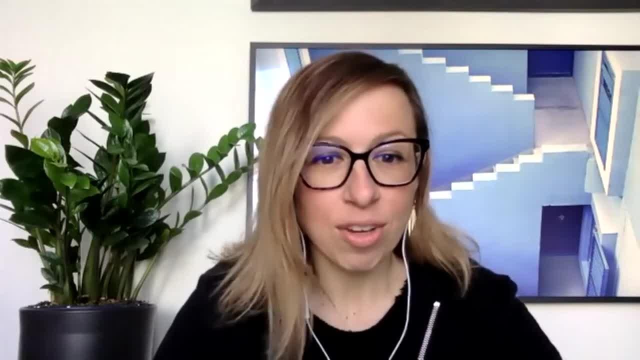 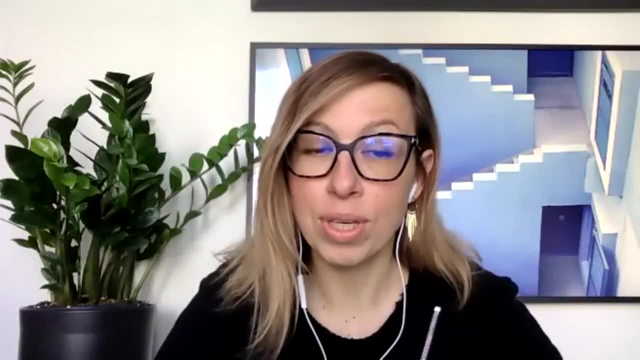 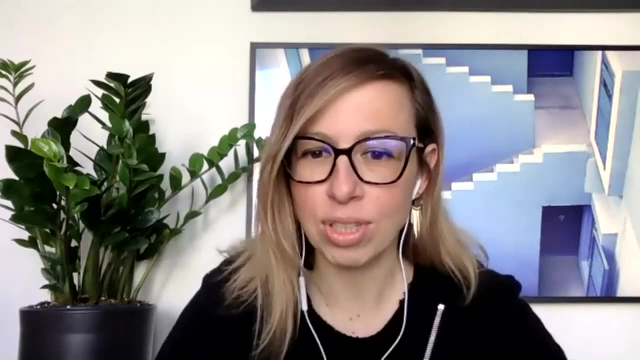 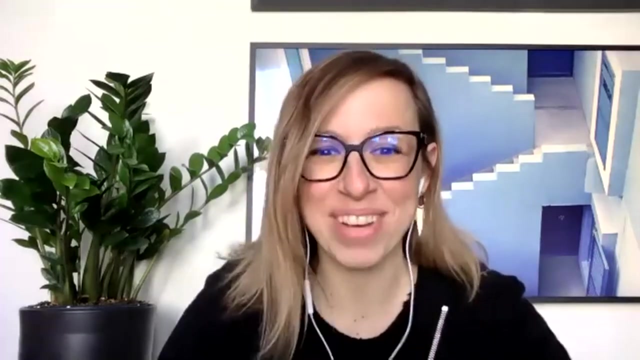 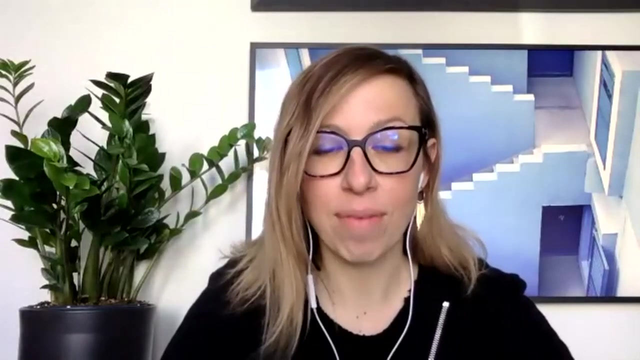 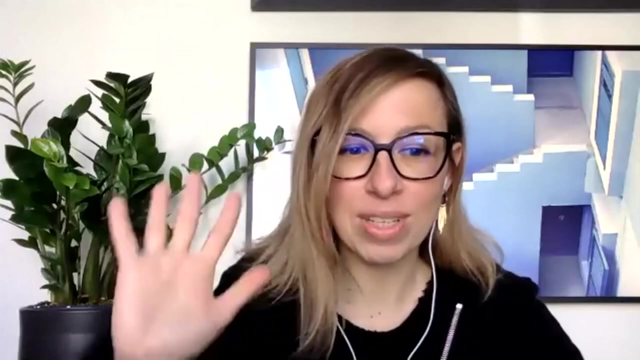 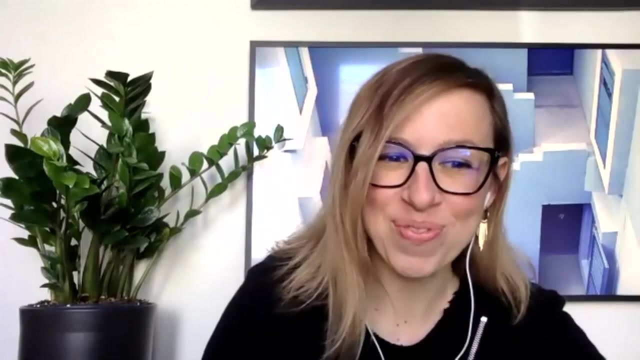 If you have questions, please pop them into the chat. That's probably the easiest way to get started. If you're a texter or the Q&A box proper, that would be great. Or if you feel so inclined, you are welcome to raise your little virtual hand and we can unmute you so you can ask your question with voice. On that note, I'm passing things over to Rebecca. Over to you. 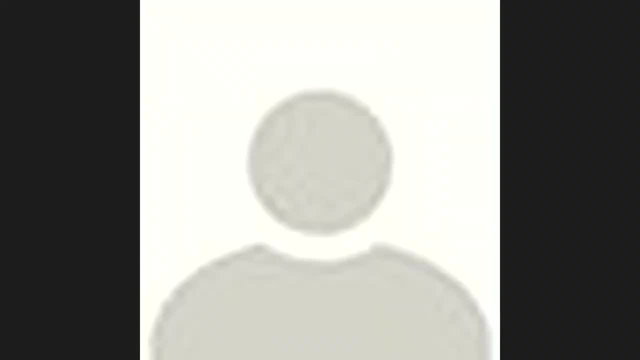 Hi everybody, Thanks for joining us today. On behalf of the Loyola Sustainability Research Center and the Loyola College for Diversity and Sustainability, I'd like to start by thanking Anna and Doug and the whole team at 4Space for hosting us today. 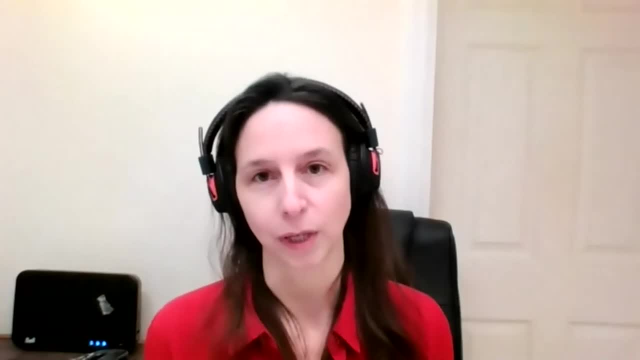 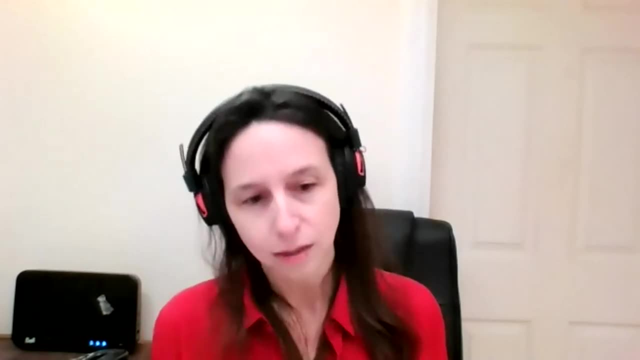 And also start with an acknowledgment that we are coming live from today, from Tiohtiagé, as Anna said, which is otherwise known as Montreal. This is unceded land of the Kanankahaga of the Haudenosaunee Confederacy. 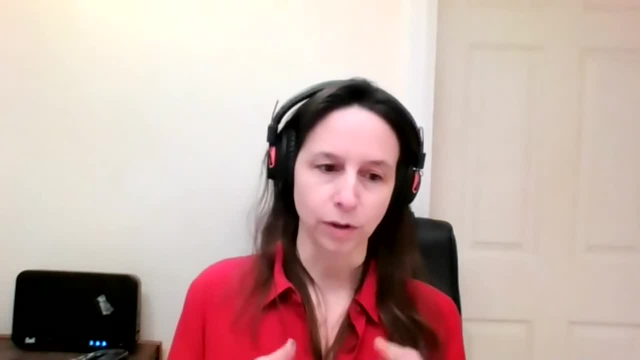 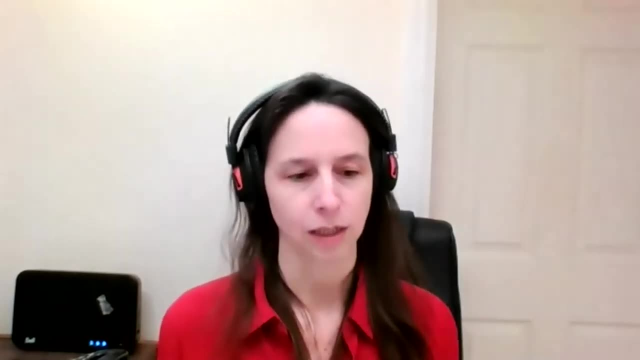 Tiohtiagé means where the two-part ways- and this is a reference to the two communities of Kahnawake and Kanasatake- that are still strong to this day in the area. Tiohtiagé is a place that is still strong to this day in the area, despite genocidal conditions. 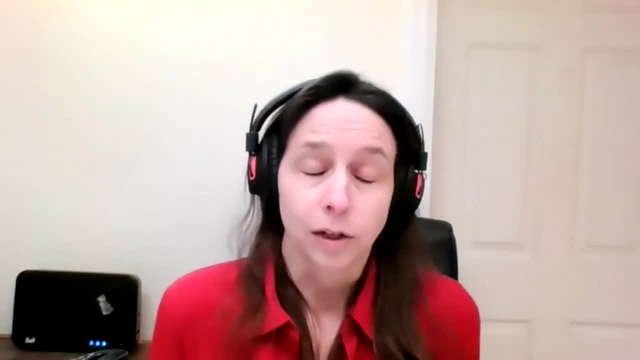 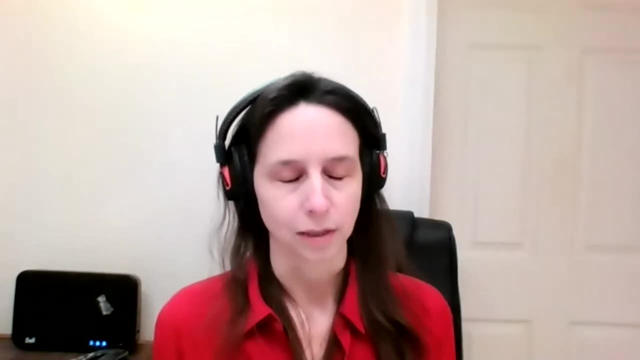 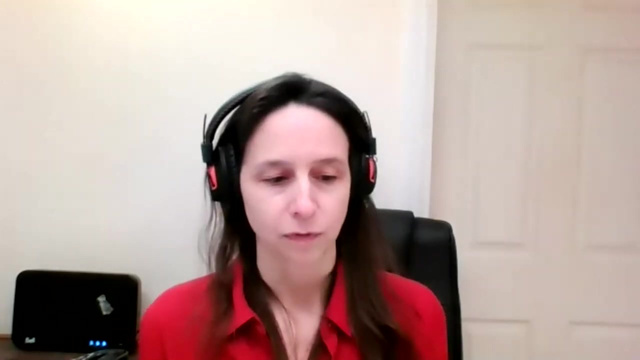 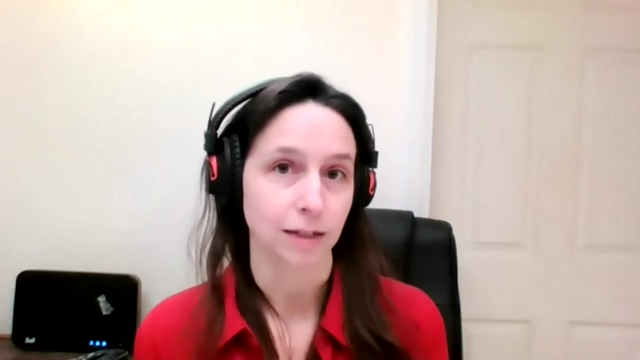 Tiohtiagé is a place that is still strong to this day in the area, despite genocidal conditions, And we recognize the resilience of these peoples and are grateful for their generosity. Tiohtiagé remains a place for those of many nations and viewpoints to meet, and that is a little bit the point of this week's series of events on sustainability in the climate crisis, which is a cross-disciplinary conversation. 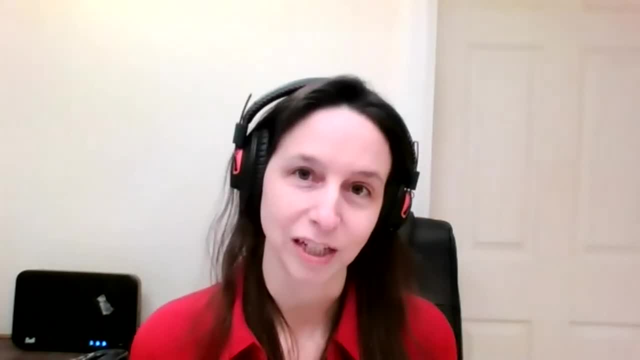 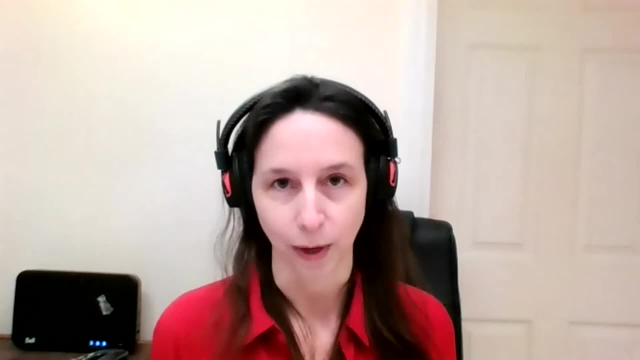 a cross-disciplinary conversation. So with that, I would like to briefly introduce our three speakers today. We will begin with Emma Desplains, who is a professor in the Department of Biology here at Concordia University. She will talk about some of her work on insects. 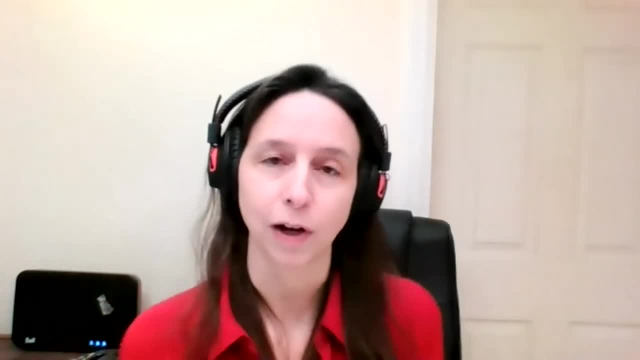 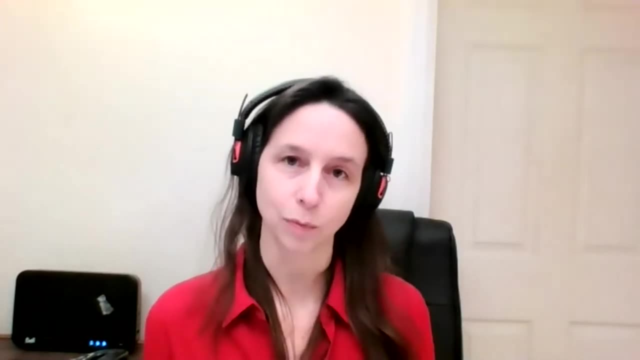 Javier Ibara Isasi will then follow her. Javier is doing a PhD under the supervision of Jean-Philippe Lessard here in biology as well, And then Pamela Yataka will present some of her MSc research, where she is also a professor at the Reception Science Center. And then Pamela Yataka will present some of her MSc research, where she is also a professor at the Reception Science Center. Javier Ibara Isasi will then follow her. Javier is doing a PhD under the supervision of Jean-Philippe Lessard here in biology as well. 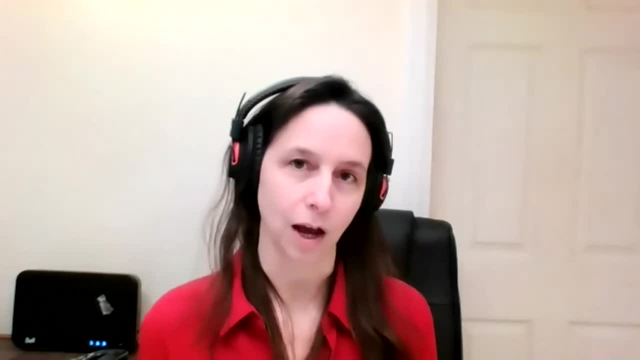 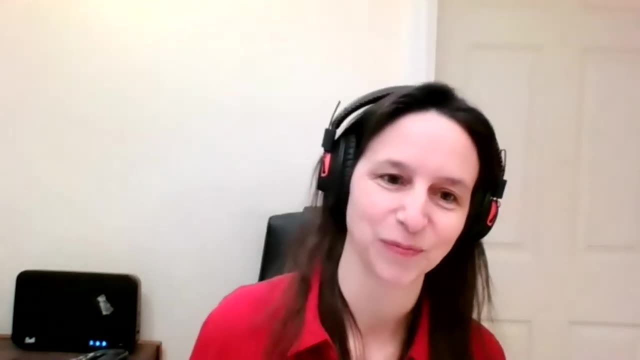 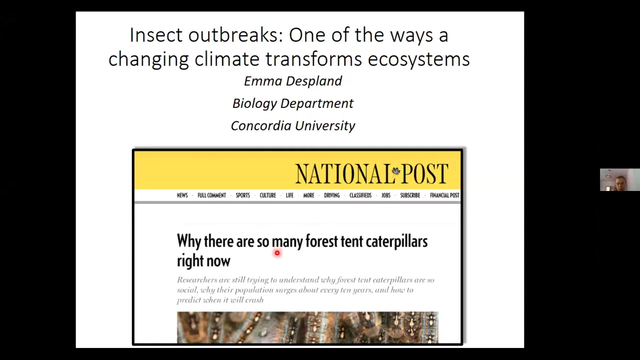 she is working again here at Concordia under the supervision of Professor Emma Des Plaines. So with that, Emma, I invite you to take the stage. Thank you, Okay. so people might have noticed that there have been a relatively large number of 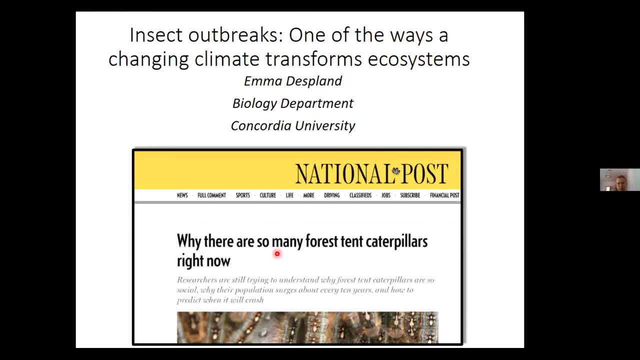 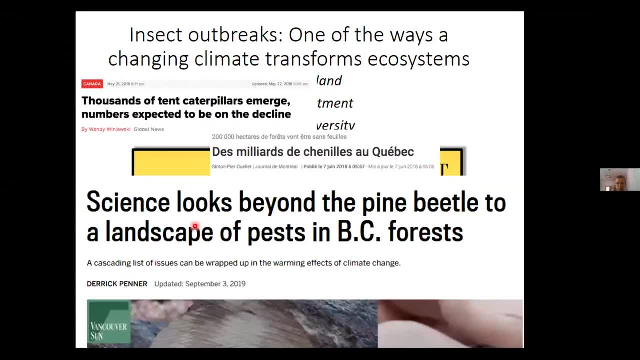 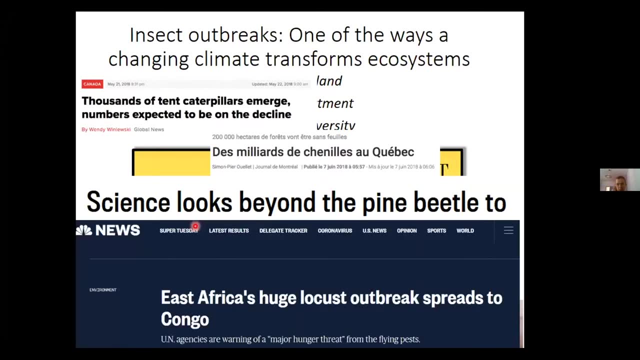 insect outbreaks that have been hitting the news. So in eastern Canada it's mostly been the forest tent caterpillar We've got. in western Canada it's been more the mountain pine beetle and in this case the link with climate change is pretty strong. And internationally there's also been large 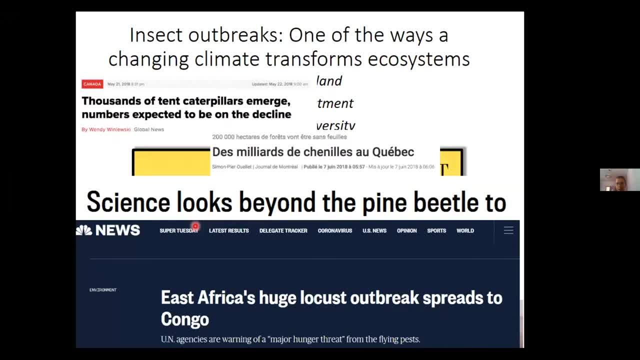 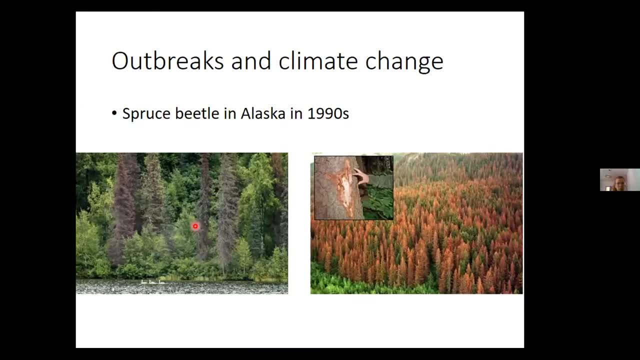 locust outbreaks in East Africa, And so what I want to look at today is some of the relationships that these events have got with climate change. I'll do that through a series of examples. Okay, so the first example I want to look at is the spruce beetle. 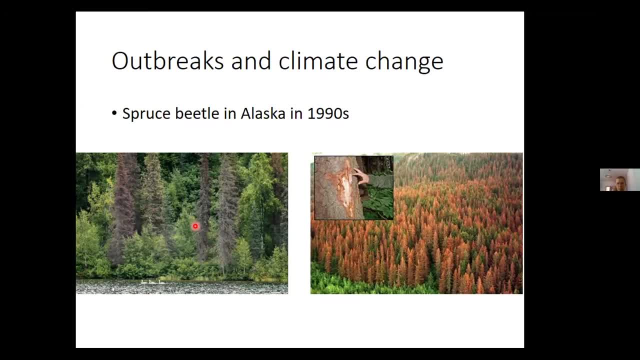 which really was. spruce beetle outbreaks in the 1990s was really, I think, the first indication that an outbreak was happening. that was different, And it was different because of a warmer climate. Now the spruce beetle is an insect that's native to Alaska, so it's always been there And what it. 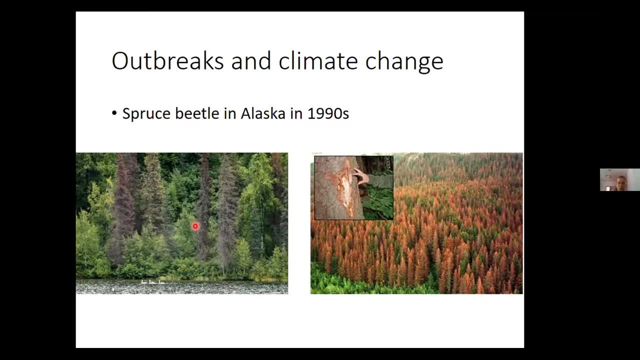 does is that the adult lays the eggs underneath part of the tree and then the developing larvae eat the soft under layer of the bark. So it causes damage like this on individual trees. But traditionally spruce beetle outbreaks are not as common as spruce beetle outbreaks. So spruce beetle 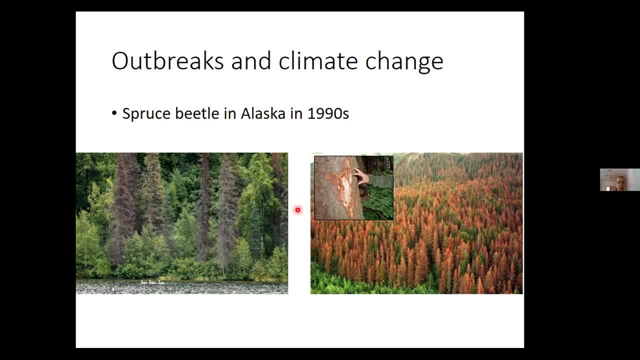 outbreaks are not as common as spruce beetle outbreaks, But traditionally what has happened is they'd only been able to attack trees that were already weak or dying in a bad state, So you'd get a situation like this, where most of the forest was still green. 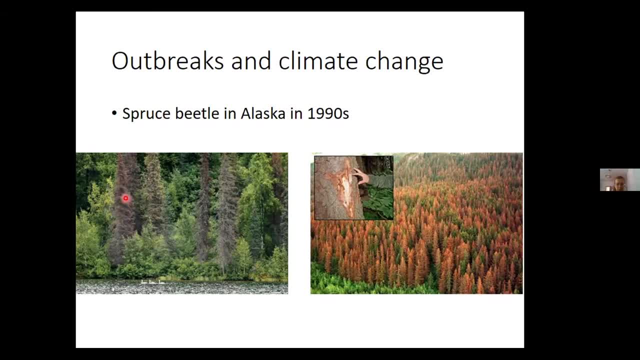 and you had a few individual trees, like this one here, that were killed by the spruce beetle. What happened in the 1990s is that you got scenes like this, where entire forests were being destroyed by spruce beetles, And this, of course, was very concerning to forest scientists. 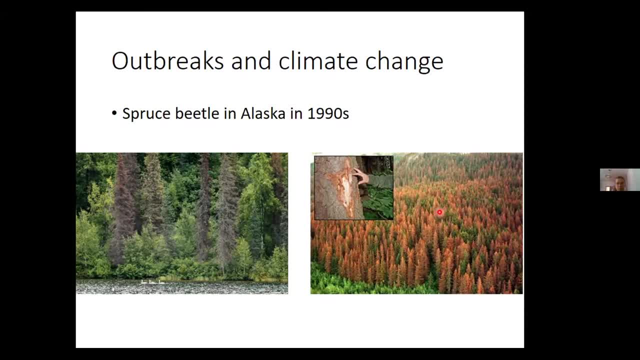 and they worked out that essentially, this was happening because the climate was warmer, And so when you had three warm years in a row, you got explosions of beetle populations, And so you did have this devastating outbreak. Less than about 10 years, it eventually 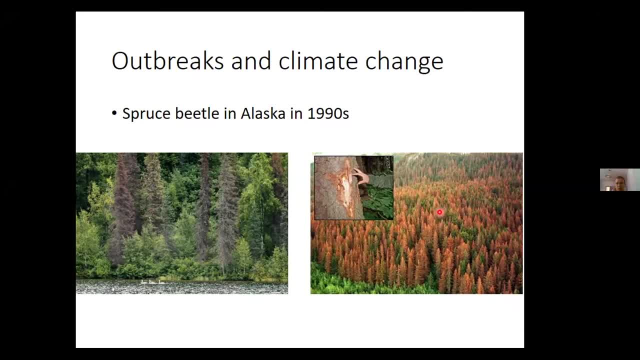 collapsed around sort of the year 2000,. because all of the mature spruce trees were dead, And so what had been a spruce-dominated forest got changed into a mostly birch and poplar, so hardwoods-dominated forest with young spruce trees growing underneath. We then fast-forwarded. 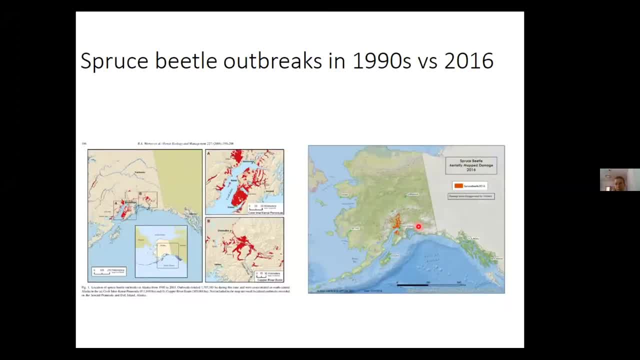 about 15 years, and now those young spruce trees have gotten big, so they've become big enough to be susceptible to the beetle. And as soon as you got those three warm years in a row- this happened in 2016,- you got another outbreak. But if you compare these two outbreaks, this was the 1990s. 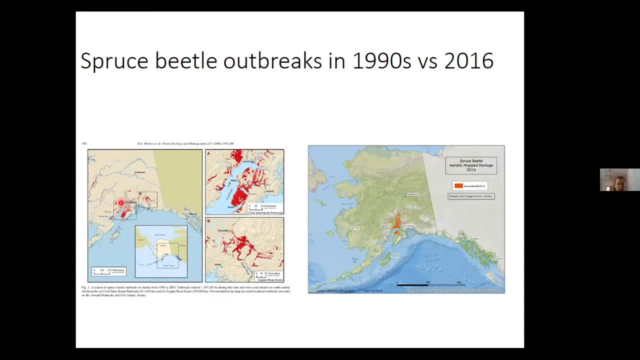 outbreak, so it was mostly on the Kenai Peninsula here and a little bit on the mainland. The 2016 outbreak touched some of those same areas, but also moved farther north, And so this is the reason why I'm suggesting two things. One, that maybe this region's spruce forest is no longer 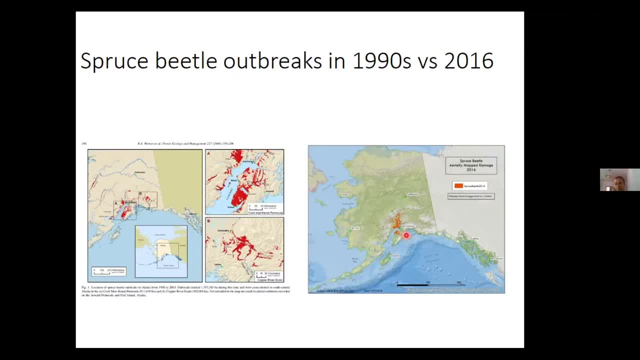 adapted to the climate they have now, because as soon as you get these three warm years in a row and you have a mature spruce forest boom, the mature spruce forest is gone. But also that if this is moving farther north, you know the climate is getting warmer and warmer. 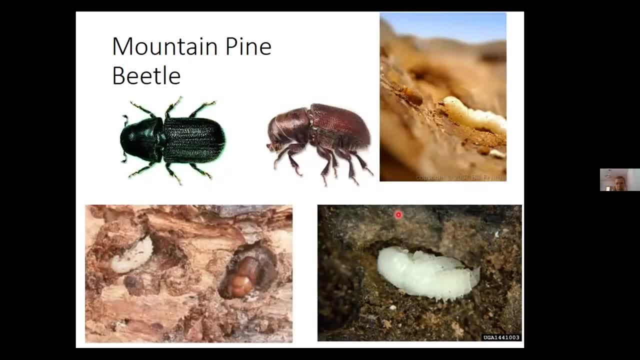 Okay if you move a little closer to home. the mountain pine beetle is maybe familiar to some people. I think it's familiar to pretty much everybody in British Columbia and Alberta. I agree, Going off here this other outbreak is- it's another bark beetle. So these are the adults. 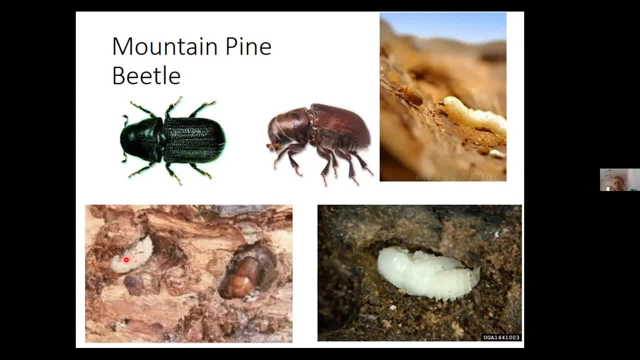 and here to the adult lays the eggs on the bark of the tree. Those eggs then develop into larvae. You've got an adult here and a larva here. These are the larvae in the adult in situ, so that larva is feeding on the underlayer of bark of that tree. And then, of course, if all the bark gets cut all the way around the trunk, the tree will die. but it's always been present in forests of northern British Columbia, But it's always been on his Brock iris himself And as direct supply along the south coast, up north, in terms of tree species and the tree we have been facing, there's four parts. 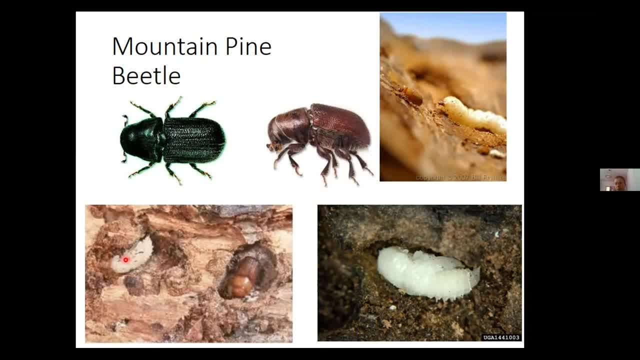 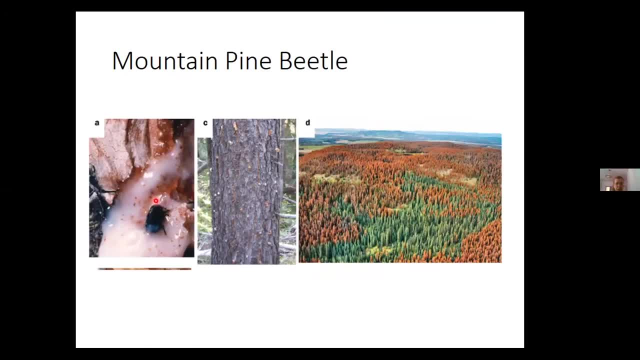 present at relatively low levels, and healthy trees have usually been able to fight them off. So trees can fight off bark beetles like this. They can actually pitch out the beetle. So you've got a drowning beetle here and all this is resin that is being pitched out or, you know, extruded. 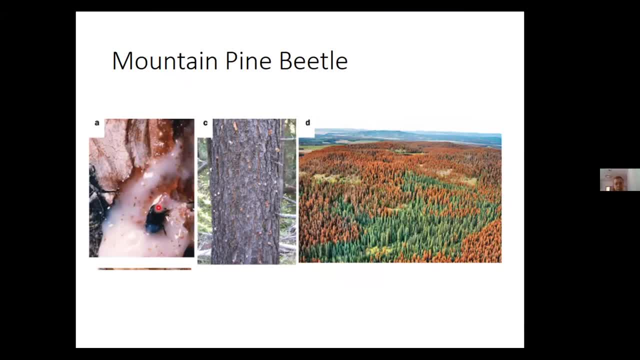 from the bark. from the bark of the tree, The tree is defending itself. It's drowned, this beetle. So traditionally mountain pine beetle has only affected trees that were already stressed or dying for some reason. What you got happening now is again: the populations are much, much larger than 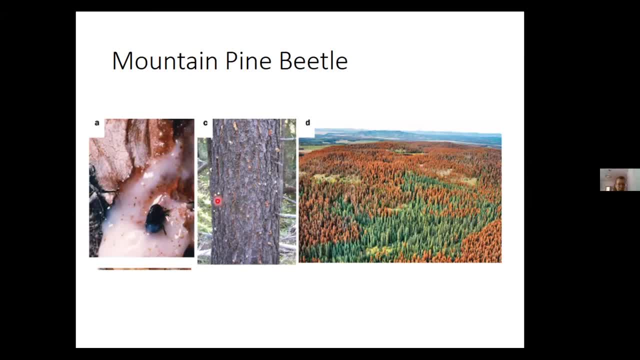 they ever were before This tree. every one of these little pale dots is pitching out, happening, But each one of these pale dots is a beetle that has affected this tree. The tree has been defending itself and pitching them out, but, you know, eventually it's going to be too much for. 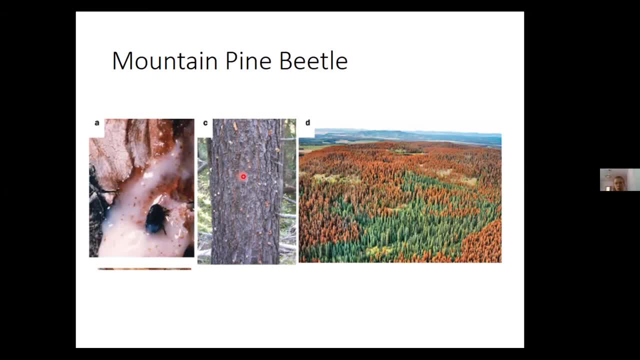 that, and this tree is probably going to die, And so what you saw increasingly happening in the lodgepole pine forest in the Rockies was landscapes like this, Where you had huge numbers of trees dying because of mountain pine beetles, And in this case it seems to have been linked to warming of winter temperatures. 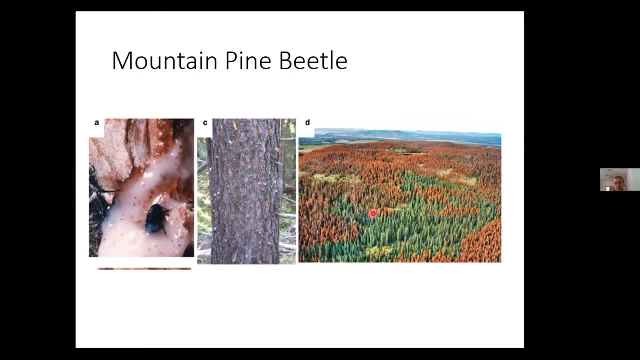 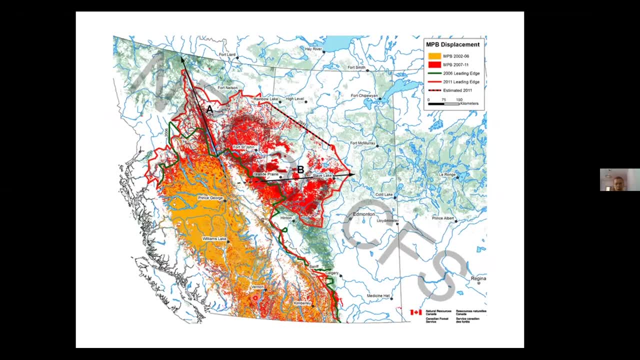 That winters are no longer cold enough to kill large numbers of these beetles, So they all survive and the populations get bigger and bigger. Okay, if we look at what this looks like on a map, The regions in yellow here are where the forests were destroyed by the mountain pine beetle between 2002 and 2006.. Beetle hasn't come back because of 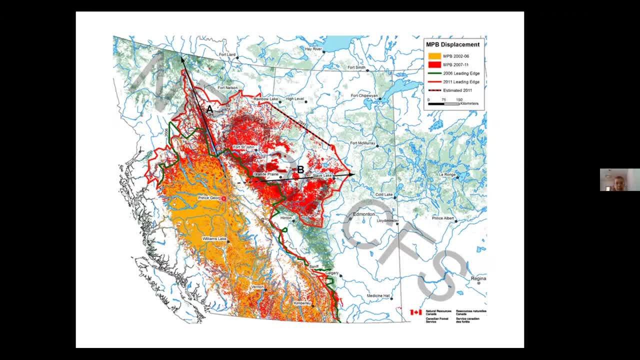 most of the trees that have been affected. The trees that have been affected have been destroyed and the trees that could have been susceptible are dead. And then it's moved farther north. It's also moved up the Rockies, across the Rockies and now attacking lodgepole pines in Alberta. 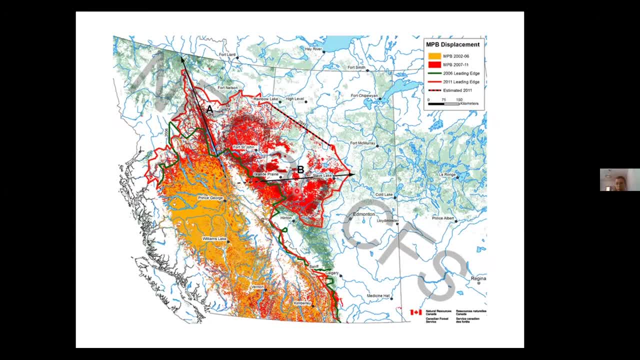 So this, of course, is raising questions as to whether lodgepole pine is now the forest type that's suitable for this ecosystem, Or maybe this ecosystem is now going to change into something else, because the mountain pine beetle is certainly having a level of effect that it didn't have. 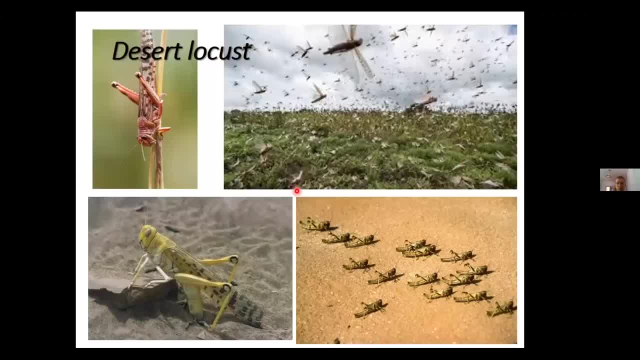 previously, If we move farther afield, the desert locust. So this is the locust I mentioned in the Bible. So it's also a native species to North Africa and Middle East, to those desert regions. Outbreaks happen every now and then and this is normal part of how that ecosystem functions. 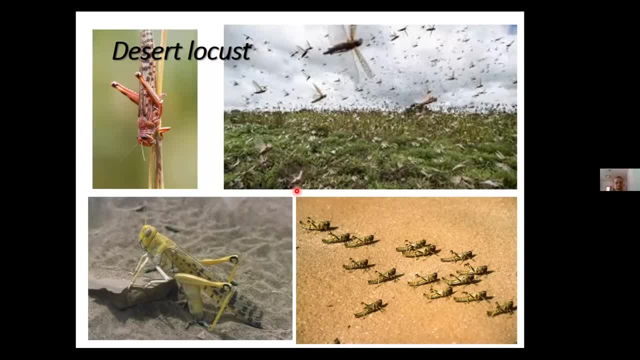 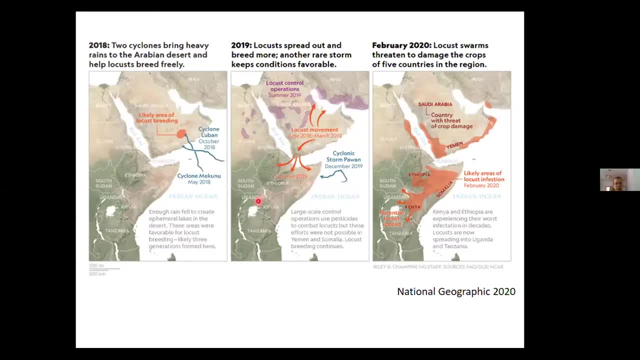 As I said, it's recorded, you know, for thousands of years, But there has been an outcast outbreak recently that has been again different, And so this started in 2008.. Linked basically to these two cyclones here that made unusually heavy levels of rainfall. 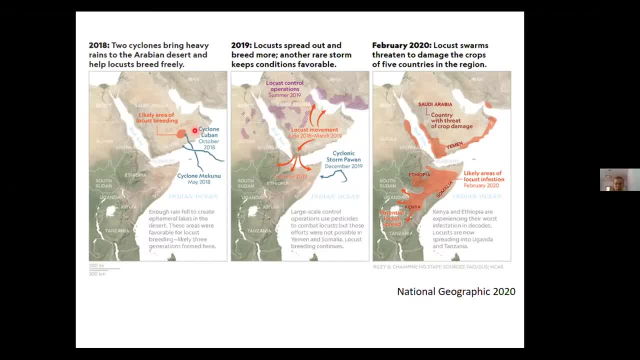 occurring here in the southern part of the Arabian Peninsula Now. this is linked to the fact that warming sea temperatures means more dramatic hurricanes and cyclones. I think we know this in the North Atlantic, that the hurricane seasons now that start in the Caribbean and move north to the United States and sometimes all the way up to us. 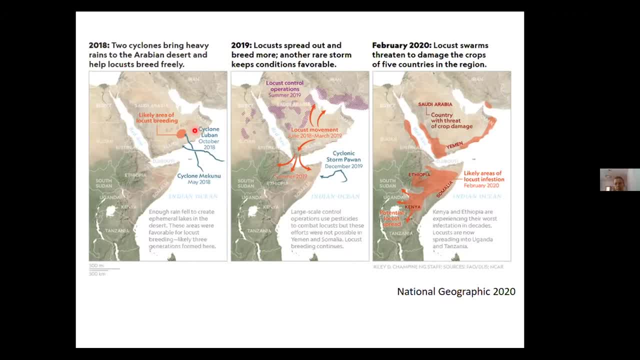 Those hurricanes are stronger and more severe and more frequent. Same thing happens in other oceans, except they get called cyclones instead of hurricanes. You had these extremely strong storms that made landfall here, Large, heavy storms. making landfall means huge amounts of rainfall. You might think huge amounts. 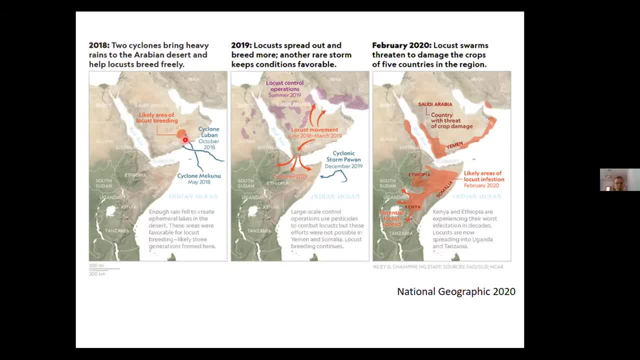 of rainfall in the desert is a good thing, but it's also a good thing for locusts. So locusts were able to breed in this vegetation, and because it's not a cold climate like we had to have here, you can have multiple generations per year, So a locust can go from egg to sexually. 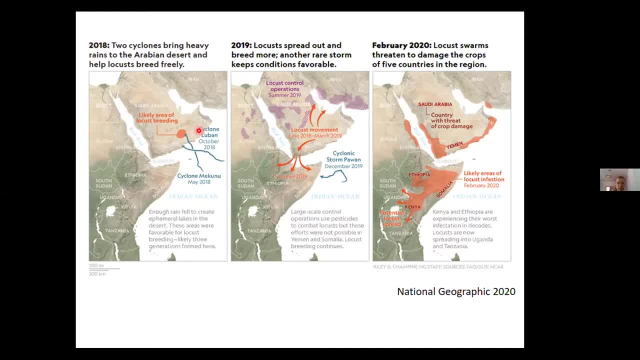 mature adult in about two months, And what often happens is that after two months- because this is a very dry, desert kind of climate- quite often all the vegetation is gone, It's dried out, And so those adults have to migrate and go elsewhere and try to find vegetation elsewhere. What happened? 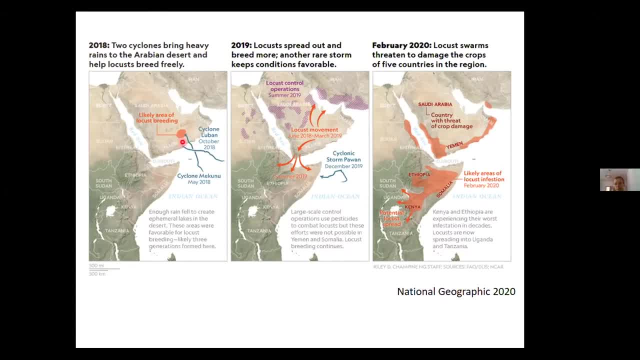 in 2018 is there had been so much rain that when those you know eggs that were laid became adults, it was still green, So they laid their eggs. And when those eggs became adults, it was still green. So you got a third generation and three generations growing here, And each female can lay several. 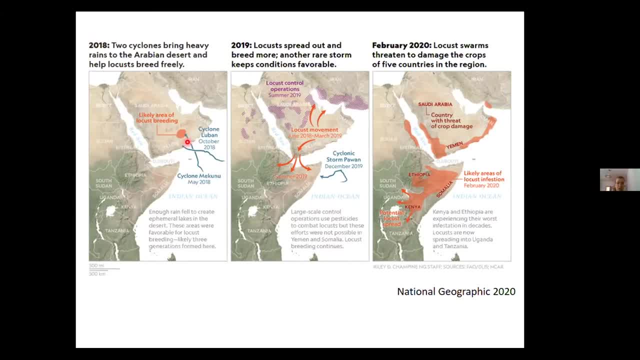 hundred eggs. So even if most of them get destroyed by predators, that still means, you know, a huge rate of population growth. So populations here basically exploded After three generations. the vegetation was gone, So then they migrated westward. here to the Horn of Africa, We have this: 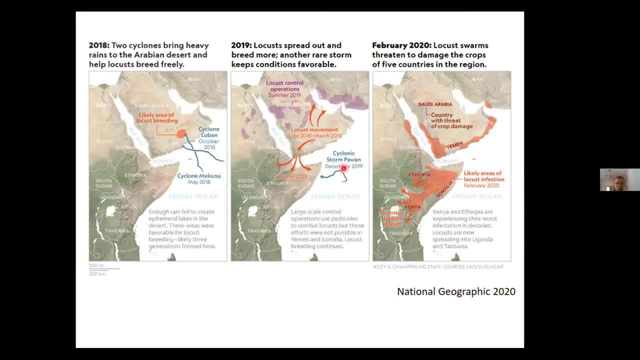 happening here And then I guess, luckily for the locusts or unluckily for us- there was another dramatic ocean storm happening that meant huge amounts of rainfall occurring here in the Horn of Africa just when those locusts were moving in. So you get another mass breeding effect. 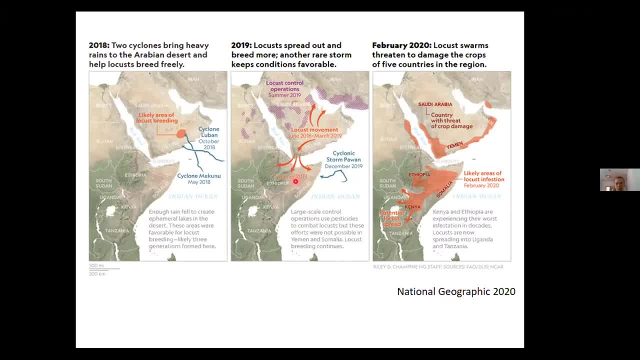 And I think it's worth mentioning that. you know departments of agriculture in these countries are not naive, So they know this happens and they usually have locust control programs. Unfortunately, Yemen, Somalia, in you know, 2018, 2019,. 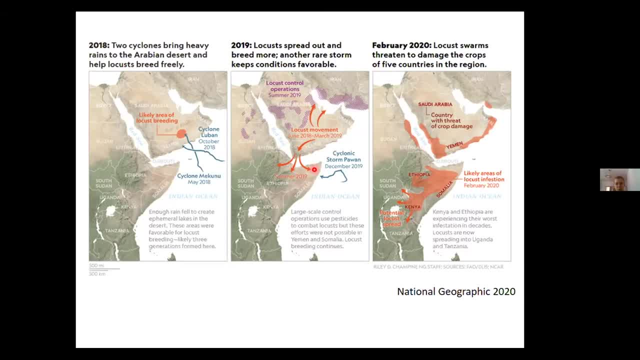 were not able to do that, And so they were able to do that, And so they were able to do that really in a situation where they could afford to invest very much in locust control. So that didn't happen. Populations exploded with this additional rainfall And then 2020, they then spread to. 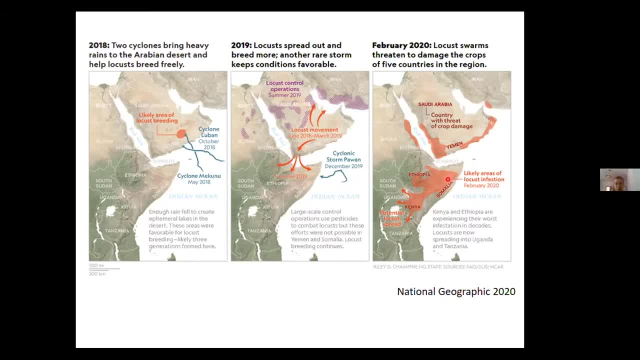 multiple different neighboring countries. Now I think it's worth mentioning that. you know, environmentally this is not so much of a problem, in that desert vegetation is by nature very ephemeral and they're adapted to. you know the upper, the above ground part of the vegetation. 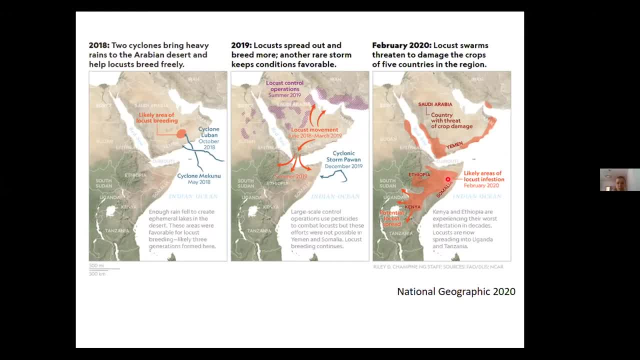 is destroyed. where they can survive And when rain comes back, either from seeds or roots, they regrow. So it's not so much changing the ecosystem, But the problem part is that much of what these locusts feed on are crops And so obviously you know massive crop destruction is. 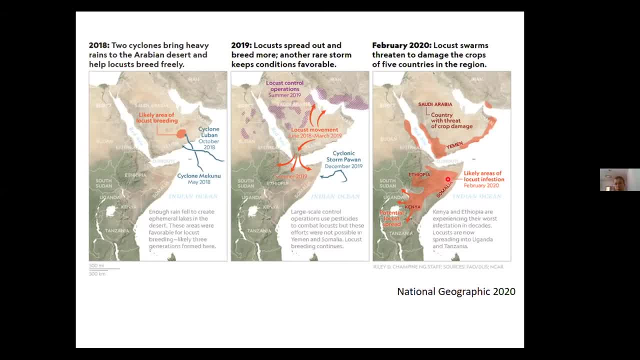 loss of income from farmers, loss of livelihood for farmers and, in some cases, food security, And so that really is the concern with locusts. Are these outbreaks going to become worse, linked to these more severe ocean storms? We're not sure, But that's maybe where we're going. 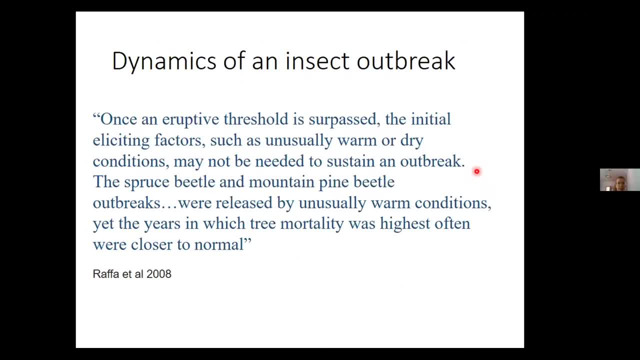 Okay, so there seems to be a sort of pattern here of outbreaks becoming worse as the climate changes. This has been studied And here are some of those generalizations that seem to be able to come out of these examples. So one is the idea of this eruptive threshold. 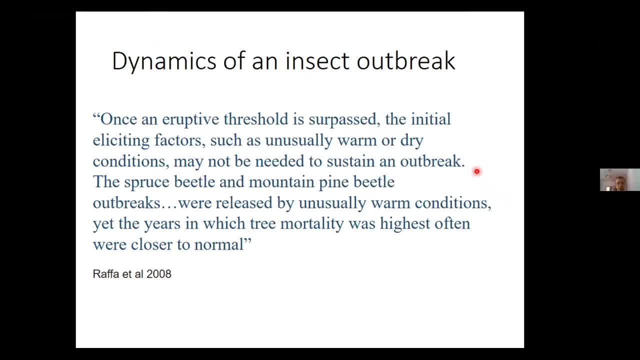 What's that threshold is surpassed, The initial eliciting factors, like particularly warm or dry conditions or in the case of locusts, are going to be worse, linked to these more severe ocean storms, Or as particularly high rainfall might not be needed to sustain the outbreak. 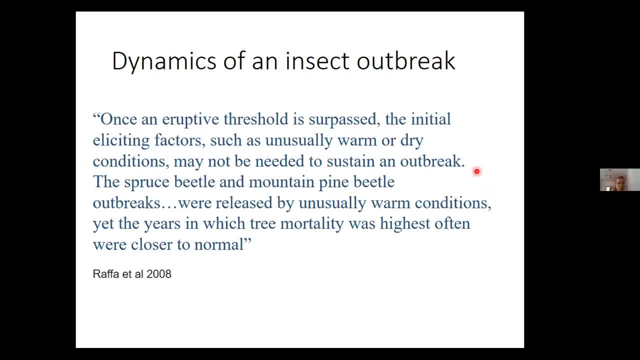 So, for instance, the spruceissimo, the mountain pine, beetle outbreaks were released or they were begun by unusually warm conditions, But the years in which the tree mortality was highest were often kind of normal years, And so this means that the climate signal is difficult to read. doesn't mean 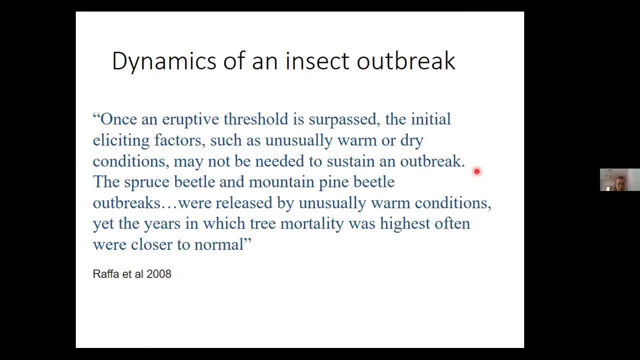 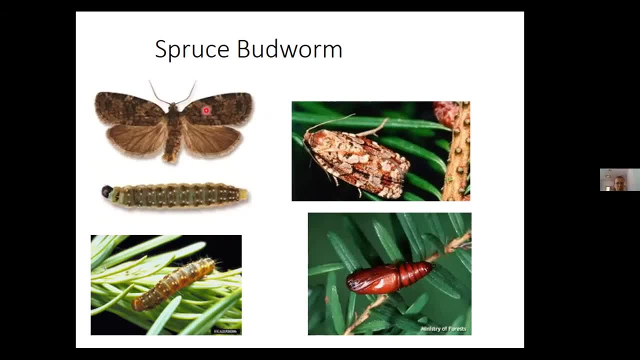 it's not there, it means it's harder to detect. I have a final example here that's closer to home, which is a spruceissimo budworm. So this is a moth. This is the adult. This is another picture of an adult: The life cycle. 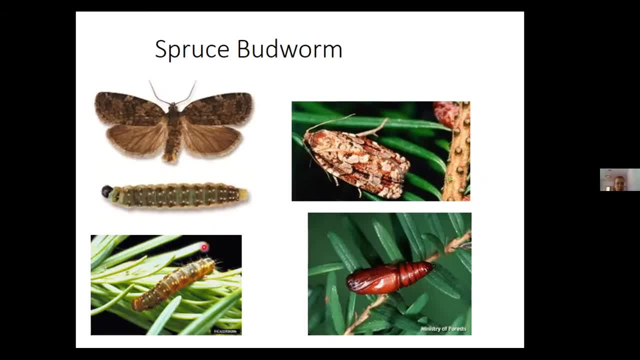 stage that actually causes a problem is the larva, the caterpillar. So there's one here. There's one here feeding on what it feeds on- spruce buds, And then this is a pupa. So the spruce budworm, again, is a native insect to eastern Canada. It's always been here, There was. 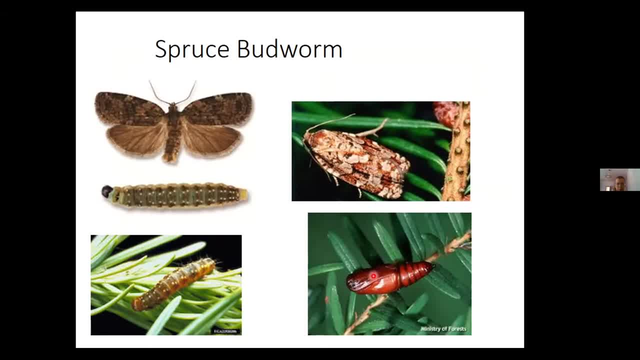 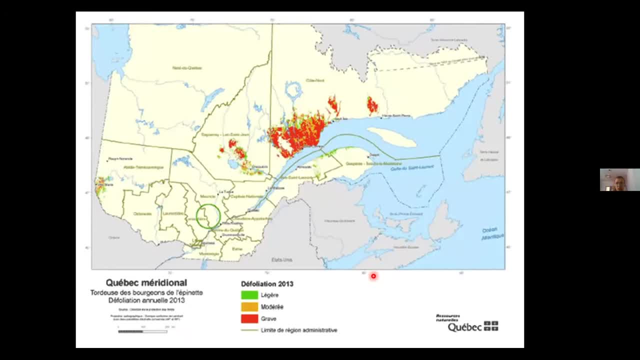 another major outbreak in the 1970s, some people might remember. We have an outbreak that started about 10 years ago and Quebec does keep track of defoliation. So basically these are people who drive around with trucks and they look at the trees and see how much dead foliage is on the trees. 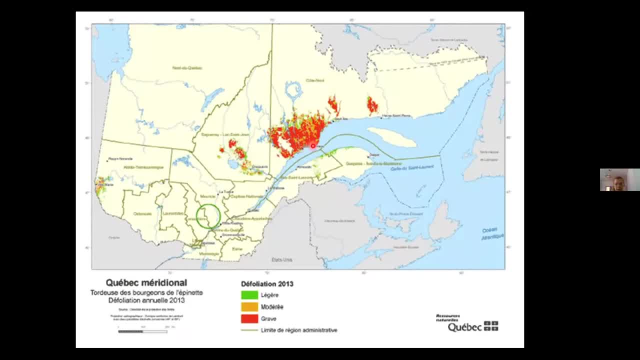 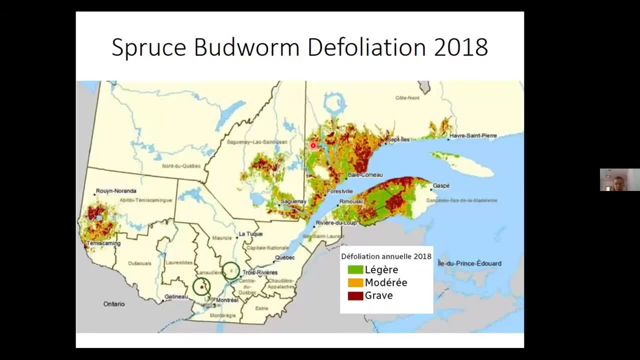 This is the status in 2013.. So everywhere is red is severe defoliation. 2014 spread: 2018.. So there you've got huge spread northwards, almost to the Manicouagan here, and southwards through most of 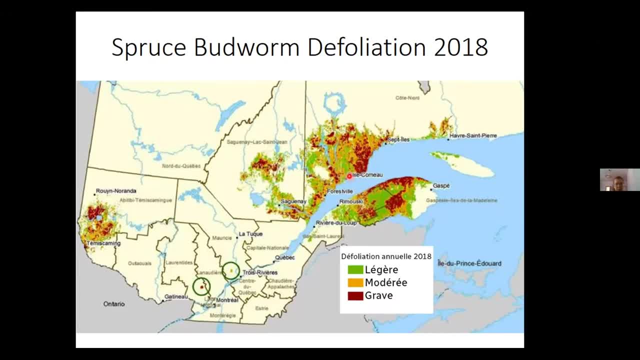 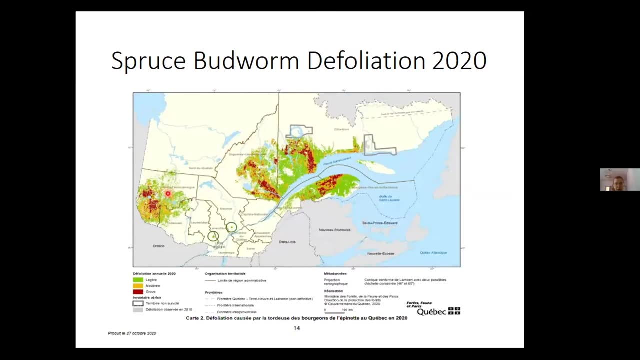 Gaspésie. It's worth mentioning that by this point, much of the light defoliation areas around Bay Como. here they're light because most of the trees are already dead, So there's nothing left to defoliate. And then, finally, 2020.. So we've got, you know, massive northward spread and the beginning of 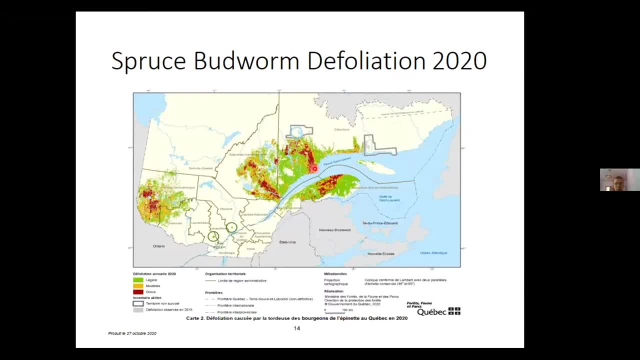 a second phocos here in Abitibi. And what's a particular concern is the spread farther north. So the previous outbreak that we know about was in the 1970s, was in New Brunswick, in Cape Breton. So that's, you know, much farther south, Spruce budworm seems to be far. 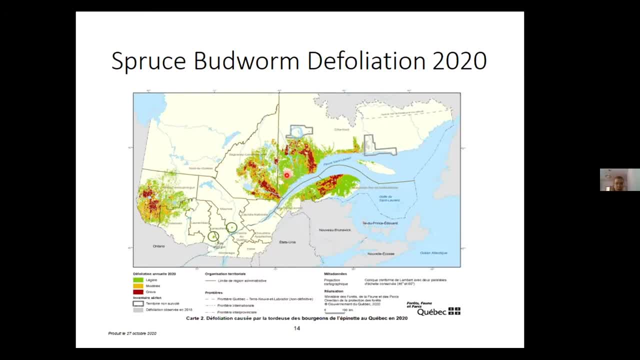 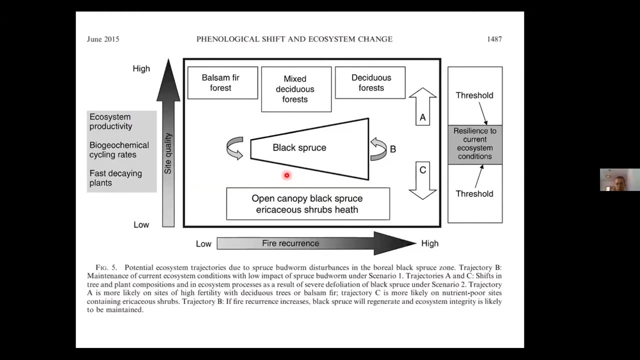 moving north, and as it's moving north, it's moving into the more boreal black spruce stands, And so there's concern as to what will happen to these black spruce stands under heavy spruce budworm defoliation. So people have to model this to try and find out scenarios of what do we think. 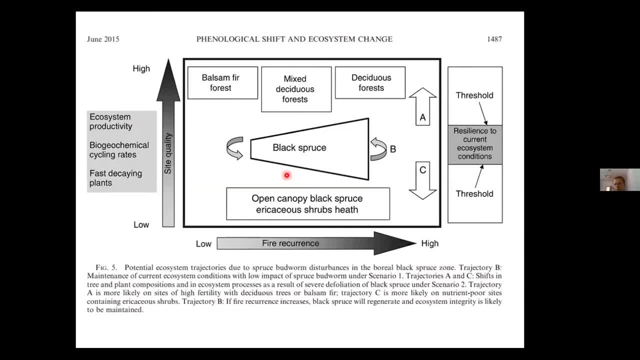 will happen to the black spruce forest, And this is because the black spruce forest is extremely economically important And there's three scenarios, which are A, B and C here, So we'll start with B, And B is the kind of things. go on as usual. 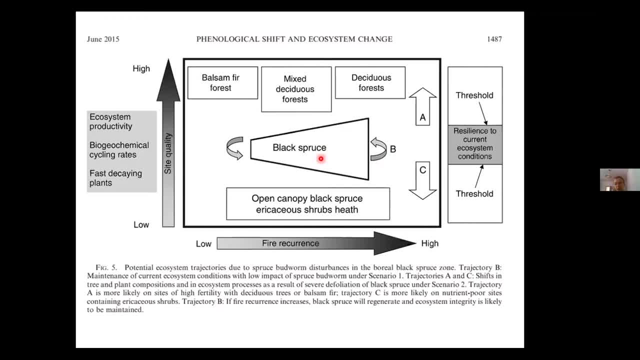 So B scenario means that, okay, individual black spruce trees die, whether it's because of, you know, spruce budworm or flooding, or heat or fire, But the forest grows back as black spruce, And so individuals die, but the forest stays the same, And so this here is in the zone, here that gets. 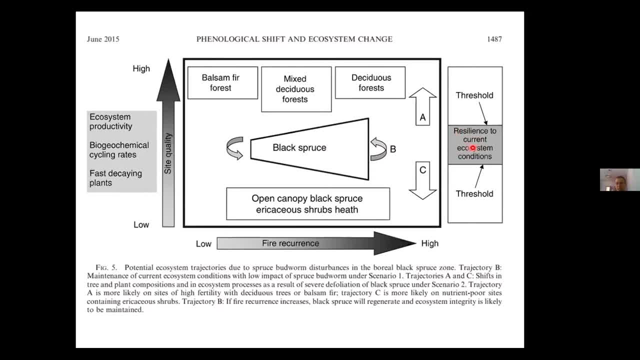 called the resilient zone. So the black spruce forest is resilient. It continues being the same thing. If, however, you pass a threshold, So if you pass this threshold here, you move into A scenario and this black spruce forest will become either a balsam fir forest, 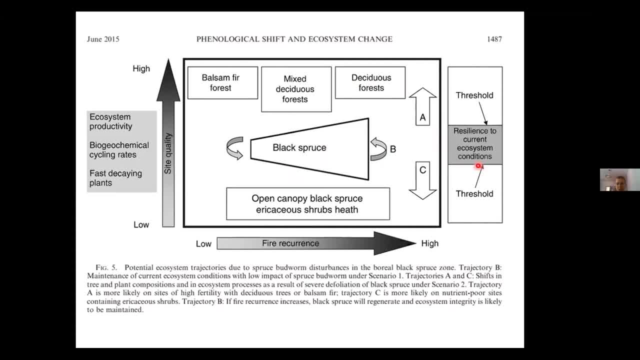 or deciduous forest. Similarly, you pass this threshold here. you're moving to the C scenario and the black spruce forest is changing to an open canopy heath, And whether we get you know A or C depends on other factors like fire recurrence or ecosystem productivity, both of which also depend on climate. 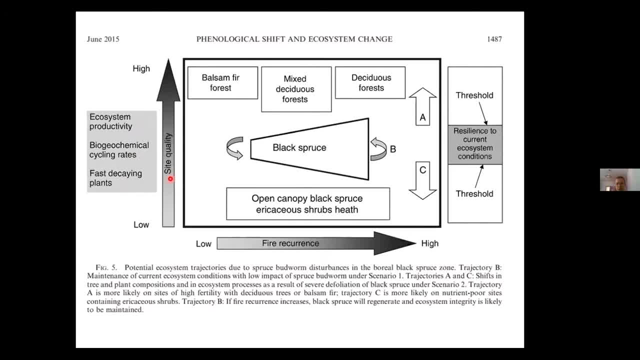 And so that's kind of the question that we have now for black spruce forests in Quebec: Are we going to stay with B scenario, which means it stays the same as it's always been, Or are we looking at A or C, where it shifts to something different? Just to give you visually what this looks like. 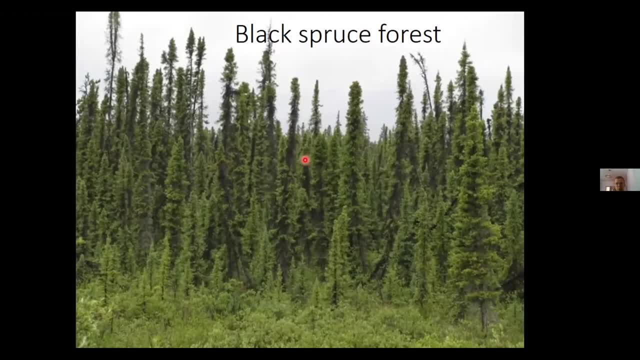 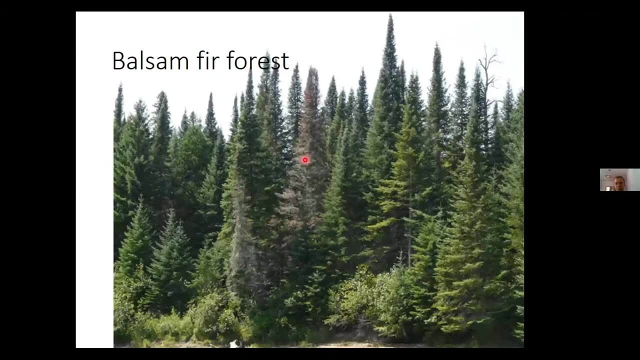 This is what a black spruce forest looks like, And this is what covers much of the boreal region in Quebec and supports a lot of our timber industry. A balsam fir forest looks like This. that might look pretty good, but from the industry perspective, balsam fir wood is really. 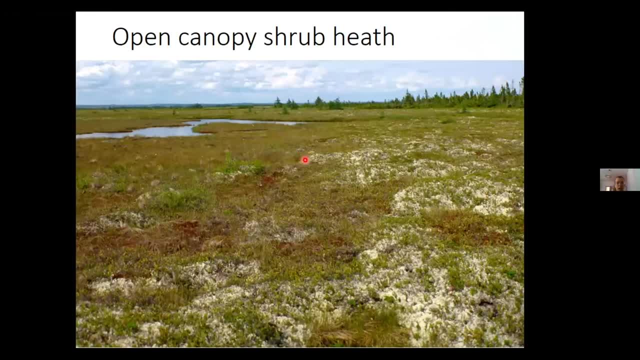 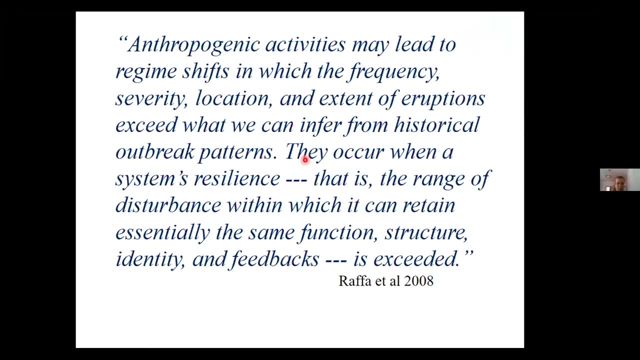 not very good quality, And then an open canopy shrub heath looks like that. Okay, so here too, if we look at it a bit, from a bit of a more theoretical perspective, we're getting to the generalization that anthropogenic activity, so human activities, 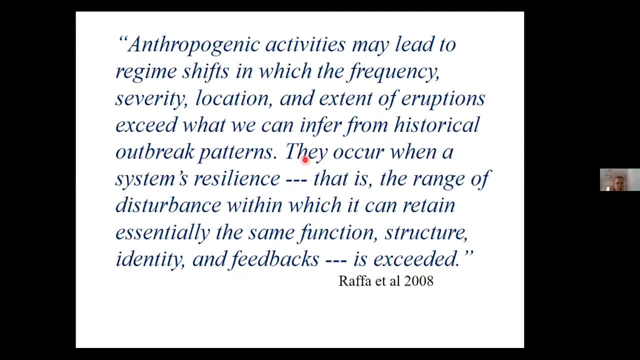 may lead to regime shifts where the frequency, the severity, the location or the extent of eruptions or outbreaks exceed what we can infer from the history. So they occur when a system's resilience- and the resilience is the range of disturbance within which the system can retain the same function- structure, identity. 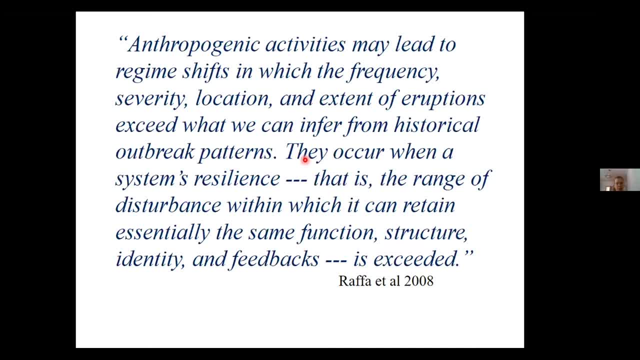 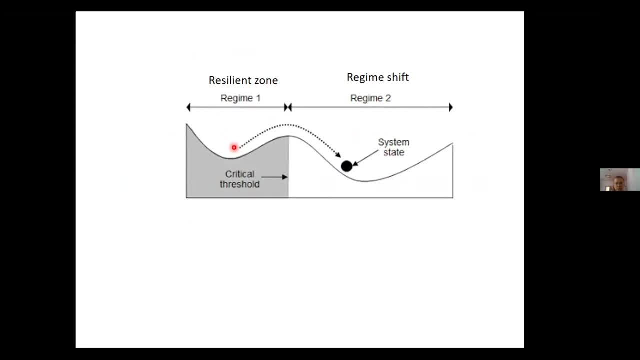 And these shifts occur when resilience is exceeded. Now, maybe that's a lot of words. This is the same thing kind of graphically. So the idea here is, if you look at my cursor here, the red dot, this is our system, This is our forest And things. typically they change from year to year. So maybe you know: one year you have a a wire outbreak, then you have a terrible heat waves, it oscillates, Or maybe you have a near freezing winter. In another example, one year a storm surge comes. 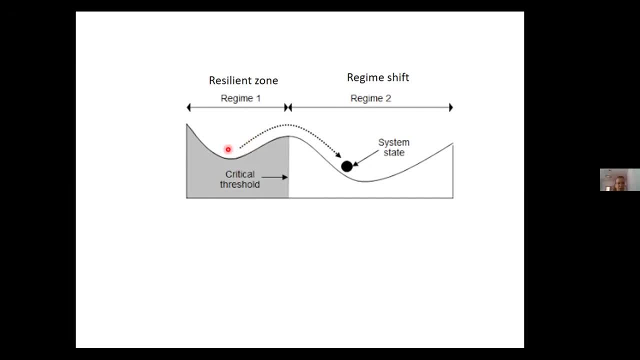 so that forest kind of changes. it goes from young trees to old trees, but it stays within regime one, It stays within the resilience zone of the same forest type. Then let's say you have climate forcing And so you have a warmer climate. and when it goes here, as you push it out the mud, there's more, então a warmer climate pushes it to here, and then you move it to this. then let's say you have climate explicitly, And so you have a warmer climate, and when it goes here, the warmer climate pushes it to here. 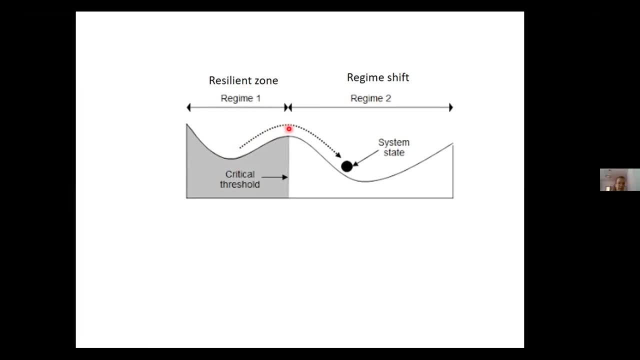 and when it goes here, the warmer climate pushes it to here, and then you push it back to there, pushes it to here, and then, once it's here, it no longer falls back. it goes over that hump and drops into regime two, and then it starts oscillating here, and so you've had a shift. 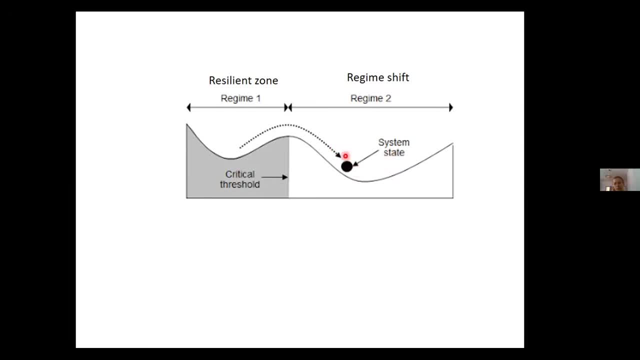 from regime one to regime two and your forest type has changed from what it's always been to something else. So if we look at the examples with the mountain pine beetle, you know we had lodgepole pine forest with climate forcing well a lot. so climate forcing and the mountain pine, 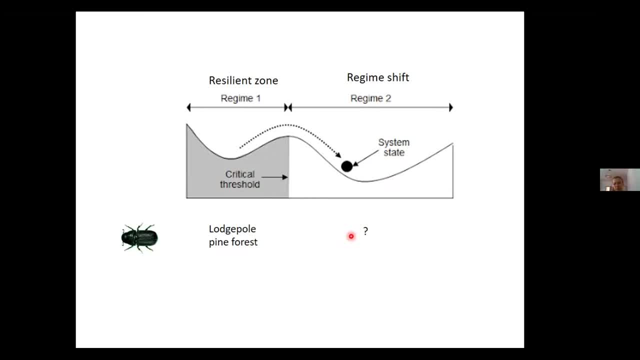 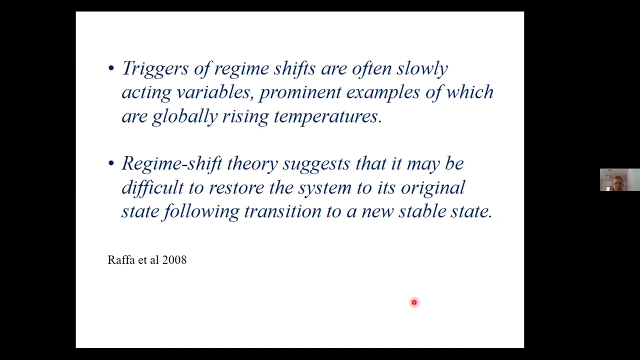 beetle have changed lodgepole pine forest to something else. If we look at the spruce budworm climate forcing with the spruce budworm is changing the black spruce forest possibly into something else, possibly into one of these open canopy shrub roots. So a couple things that are worthy of note about these regime shifts is that the triggers are often 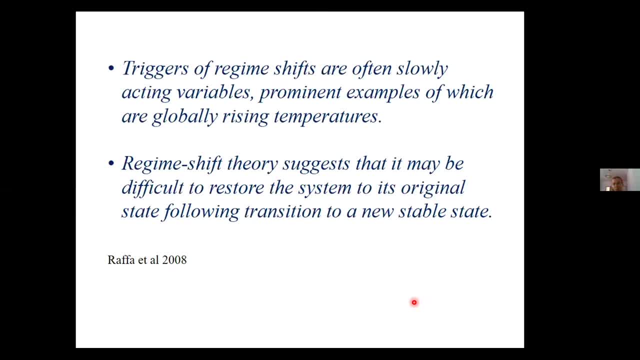 very slowly acting variables, things like globally rising temperatures, And so these very slowly acting variables are things you don't really notice because they're kind of hidden in the noise, but they do still give that additional shove to move the regime, the system, from one regime to another. And then the theory suggests that once that shove has, 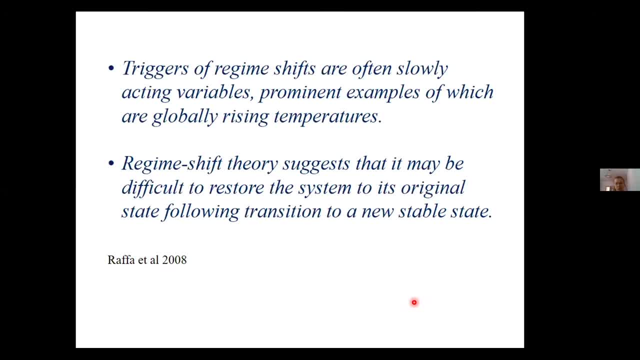 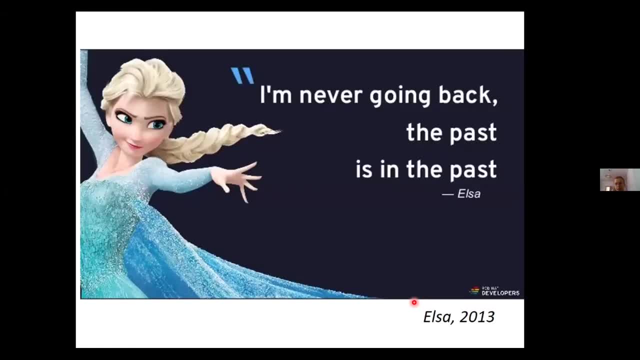 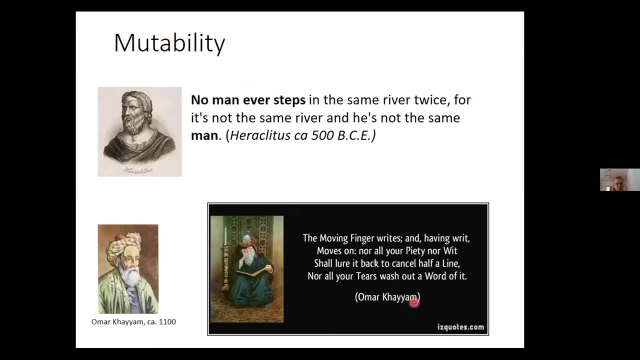 happened and you fold over into a different regime, it's very, very difficult to restore the system to its original state. Another way of saying this is that we don't go back past is in the past. Now that maybe seems a little superficial, but we've got some more serious philosophers saying the. 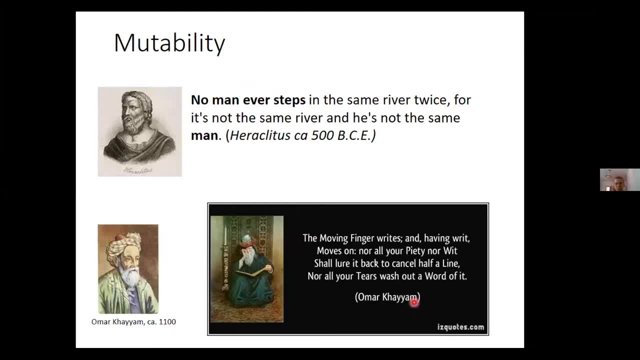 same thing, and this is an idea that's called called mutability. Mutability is that change happens and we have to live with change, And I think these people were talking about change more. you know changes that are lost. So I mean, in Elsa's case, change was liberating. It isn't always. Sometimes, 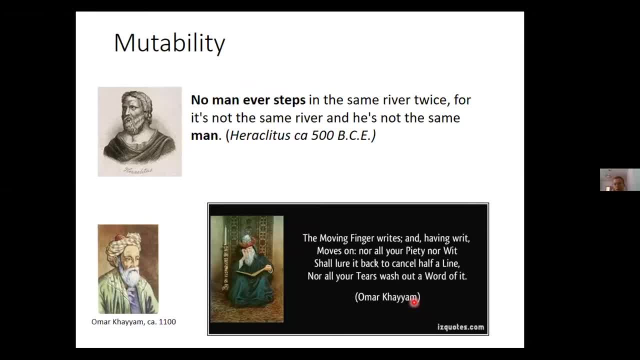 change is lost. I think we know this, particularly with the pandemic. you know we're not going to go back to the pre-COVID world. All the people who have died are not coming back into the world. So where do we go from there? We do still need to move on, but we need to move on from where we are. 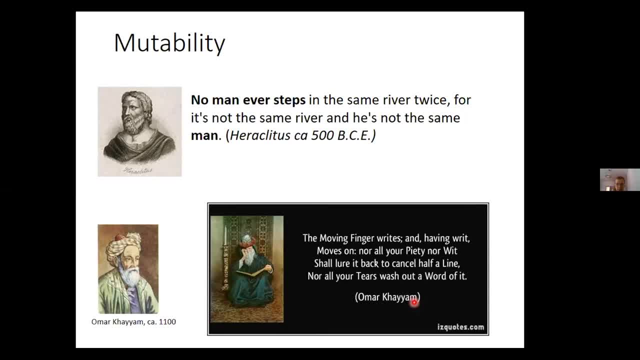 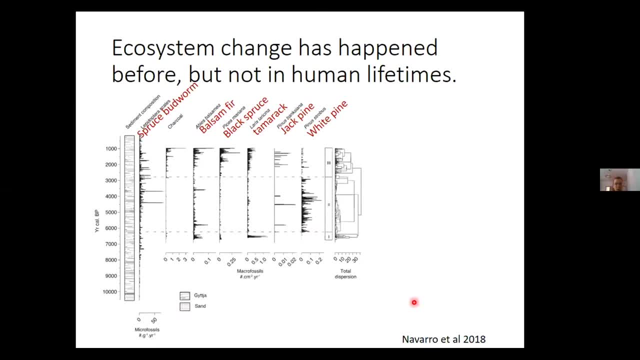 now and not regret where we were in the past. So what does this mean in terms of forests and insect outbreaks? I think one thing that's worth mentioning is, if we look very far in the past, ecosystem change has happened before, Just not in our lifetimes or anybody's life. 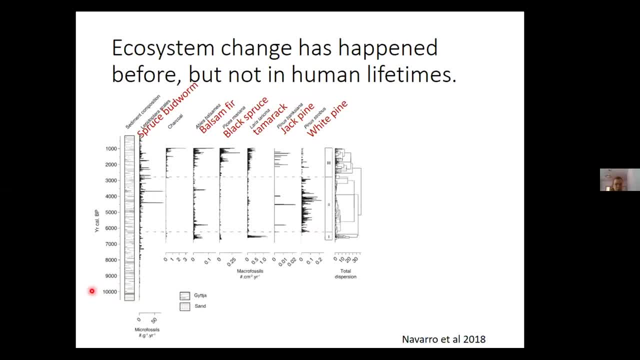 So this is paleoecological reconstruction of forests around the Chicoutimi area, So northern Quebec, what is now black spruce forest, And this is over the past 10,000 years. So that's really, you know, since the last dice age. 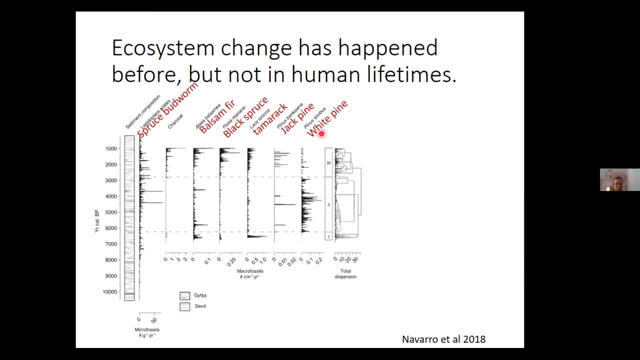 And here they've got a range of different kinds of indicators. So here I've put the trees. These are pollen from different trees, and I put the three species names in English under the Latin ones. Charcoal is an indicator of fire and this is spruce budworm wing scales. Now I'm 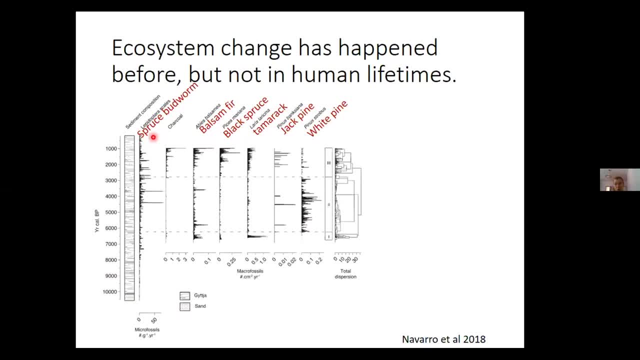 incredibly impressed by anybody who can dig out moth wing scales from 8,000 year old mud. But people apparently can do this, and that amazes me. But what it shows us is that, for instance, the fire frequency indicated by charcoal fires have been more frequent recently, relatively recently. 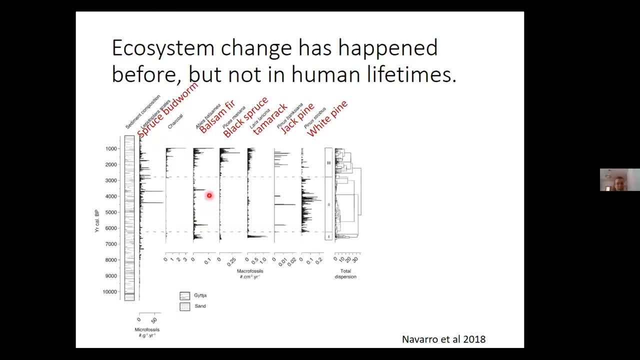 than they were, you know, thousands of years ago. Composition of the forest, in terms of trees, has changed. So white pine, you know, doesn't really grow around Chicoutimi now. 5,000 years ago it was dominant Black spruce, which is dominant now. 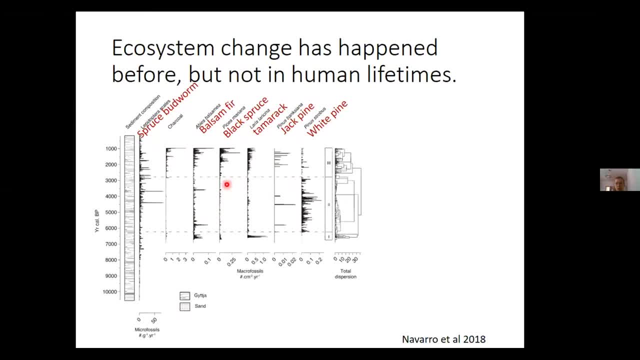 wasn't that important. years ago It was there but it wasn't dominant. Spruce budworm has been around and there have been outbreaks over the past 10,000 years, So we can't say that outbreaks per se are new. Whether outbreaks happened in the boreal and changed erratically changed. 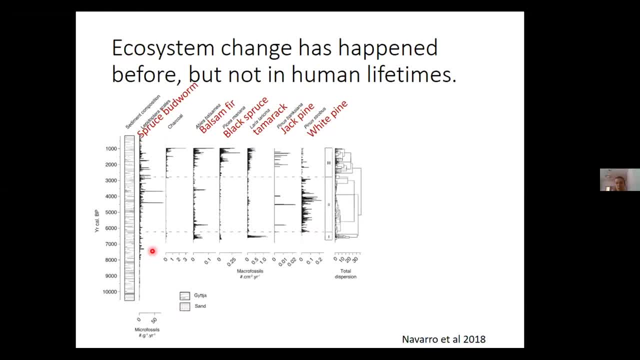 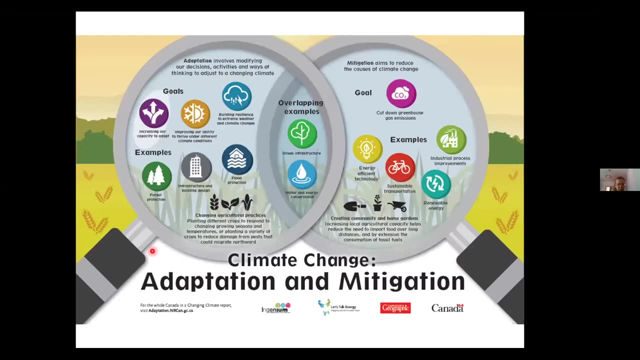 black spruce forests? we don't really know, But so what we're seeing now is unprecedented times. It doesn't necessarily mean it's unprecedented in geological terms. In practice, what does that mean for us? I think there's two concepts here, which are climate change. 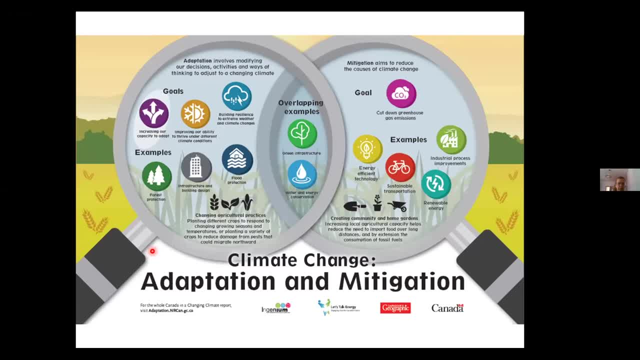 Really, it should be the other way around. It should be mitigation first and adaptation second. So mitigation is really reducing the causes of climate change. You know, we know climate change is causing bad things, so let's try and slow it down, And this is something that is. 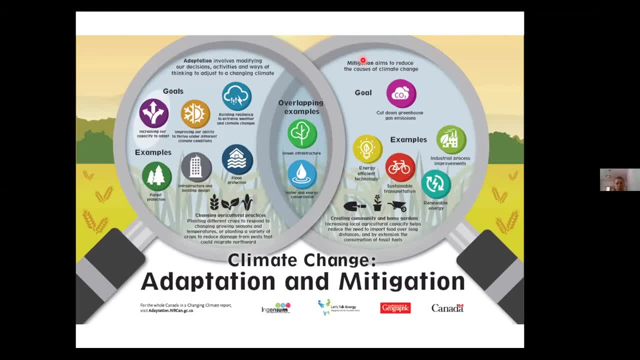 really for the collectivity It's, for society in general to address. Adaptation is recognizing that climate change is happening and that we need to change the way that we behave in order to live with that. In our case, we're talking about forest protection. 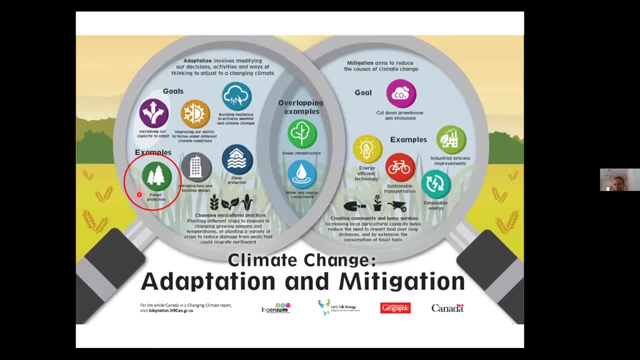 What this means is that if you're a forest manager, maybe recognize that what you learned 20 years ago is not true, because the forest that you have now is not the forest that you know, your professors knew, And that you need to be more creative and more adaptable to manage the forest that we have. 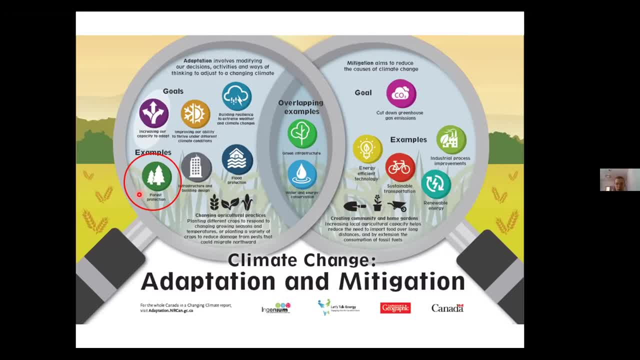 now, under the conditions we have now. Thank you, Thank you, Emma. I remind the audience that we have time only for a couple of points of clarification after this talk and then we will take more general questions at the end of the talks. So I do have a question from Carly Zeder For your first example, for your final example. 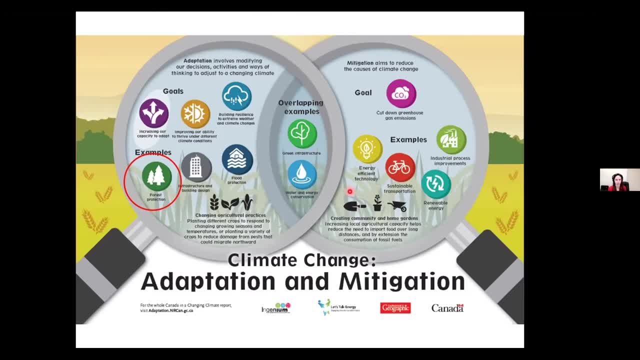 how well are we able to predict whether we're close to these thresholds? For example, are there early warning signals that can tell us whether we may be approaching a regime shift? and even if we know it's coming, are there any management strategies we can use in the forest? 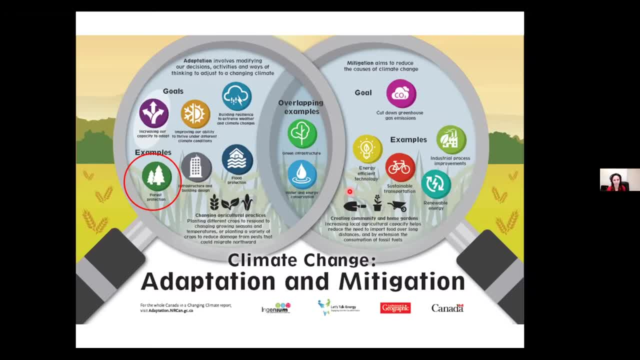 systems or is the shift inevitable? Great question, Yeah, I mean. I think it's, that's extremely system dependent. So, for example, the spruce budworm. you know, the reason why there was that paper showing those three scenarios was an attempt to say we think we might be getting close to a regime shift. 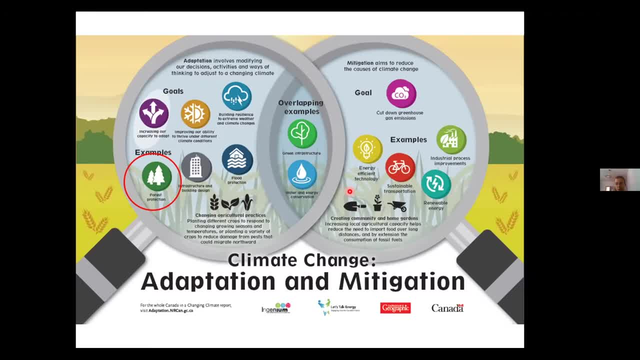 If we are. here are the possible scenarios and let's think about how we can adapt to that. But what's true for the spruce budworm? you know, the mountain pine beetle is not the only one, it's the other. But what's true for the spruce budworm, the mountain pine? 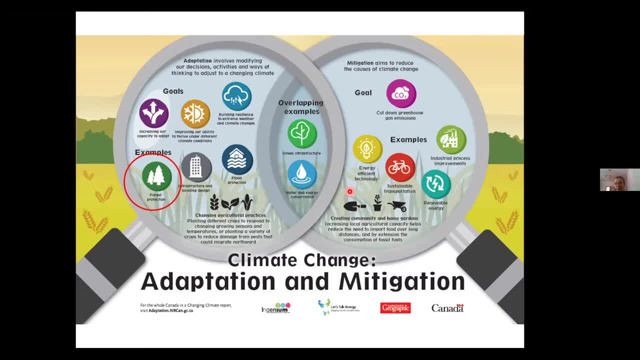 beetle is a different system. I'm not aware of any general answer to that. That would be too easy. Another question: any comments as to where we are at regarding the gypsy moths? Are we close to a shift? OK, One thing that's worth mentioning. 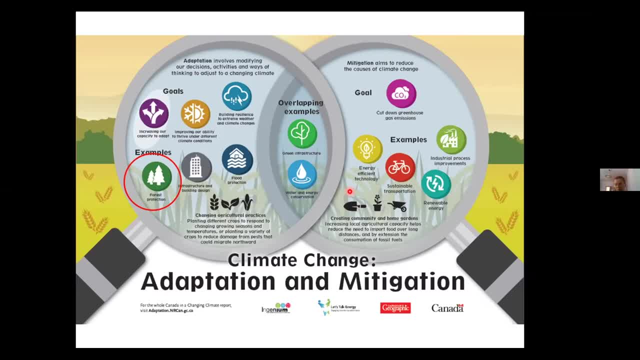 is. the European gypsy moth has been in Quebec and eastern North America for about 40 years. It's kind of resurging. So it's a novel system. The Asian gypsy moth has not arrived in North America yet And there's a lot of concern that it. 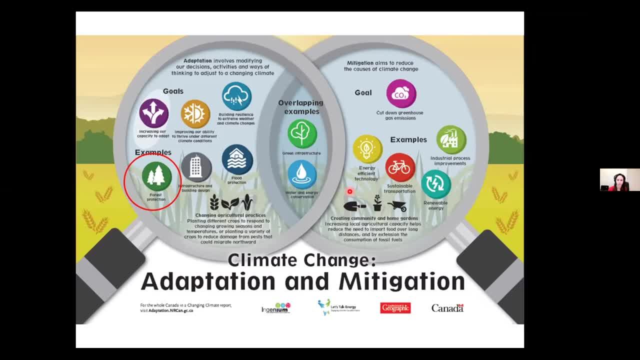 will get here at some point, But it's not there yet. So there is sometimes confusion. when we say gypsy moth, Do we mean the European one or the Asian one? I think the European one. there was concern that it would be completely destroying the forests. 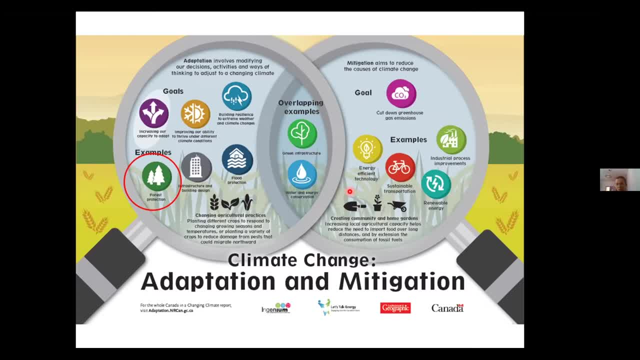 I think it was in the 1980s and then a pathogen got introduced and it kind of went down. It's kind of on its way back up, but I'm not aware of it being close to shifting yet. But I think that's one thing. that's hard with outbreaks. 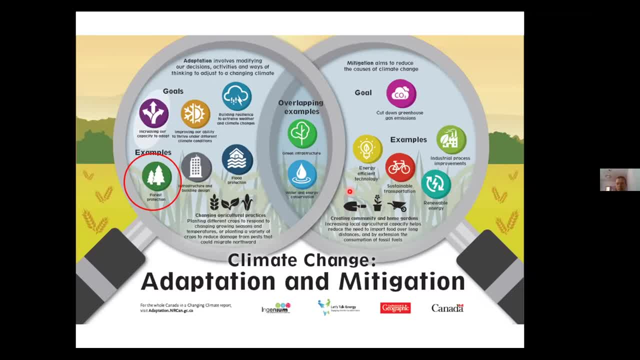 is that locally they're devastated, But maybe that's normal. So how do you tell between normal devastation and something new, especially with things like the budworm, where the cycle is 40 years? So the last one, The last one was in the 70s. 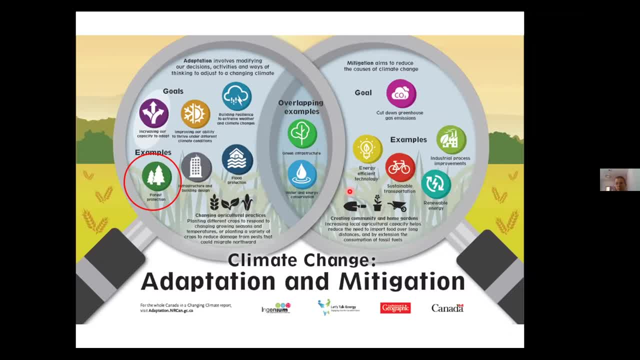 We know something about it. Some of those professionals are still around. The one before that was the 1930s. The one before that we don't really know anything about. So we have like an N of three, which is not a lot. 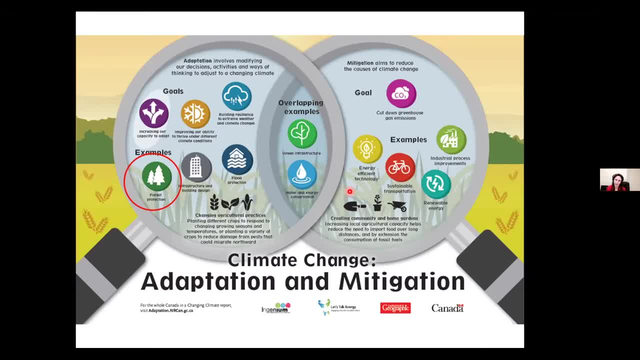 Right, OK, I'm going to take one more question and then we'll move on to Javier. So a question from Jochen Yeager: How many insect populations are declining due to climate change and chemical pollution now? So some are increasing and others are declining. 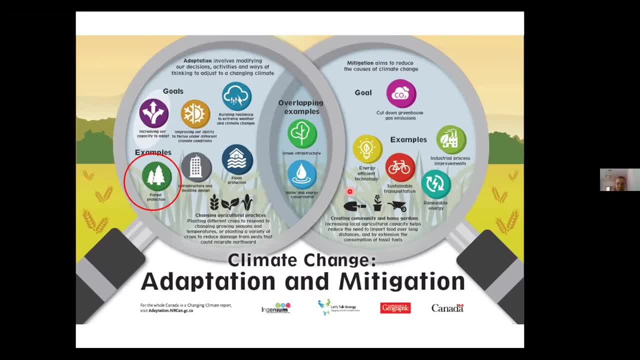 Yeah, Yes. So I think there tends to be a sort of- and I think the decline will be spoken to by the next speakers, But in general we do kind of see a homogenization that the few species who do well are becoming. 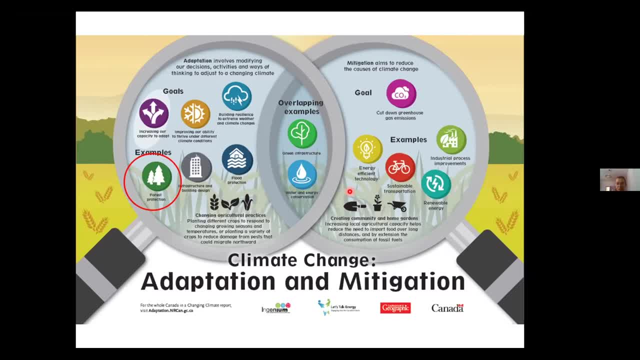 there's more and more of them, And then the broad diversity of species that maybe don't do so well under these new conditions. they're the ones who are declining. So we might have large numbers, but we probably have lower diversity. Thank you, Emma. 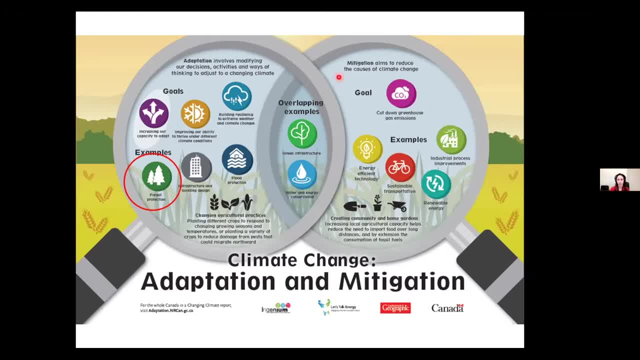 I'll invite our audience to please hold on to your questions, or you can put them in the Q&A and save them for at the end of the presentations, But in the meantime I'd like to invite Javier Nibarra-Essazi. 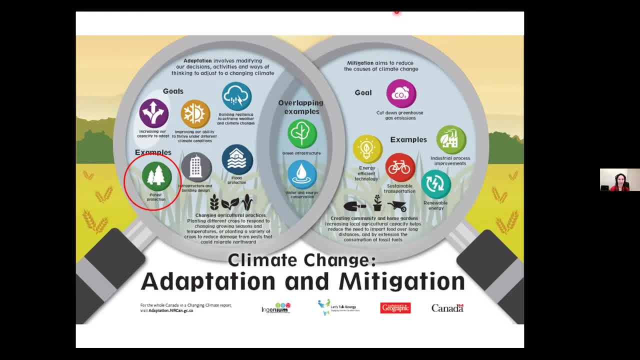 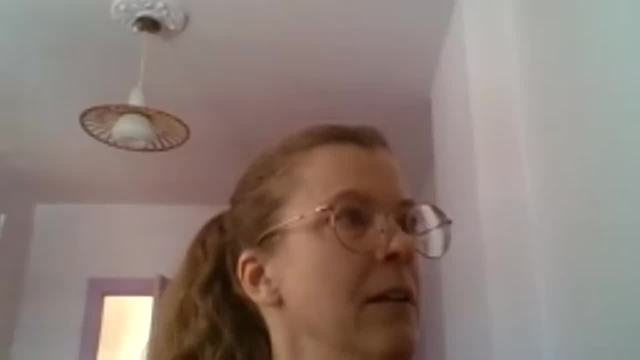 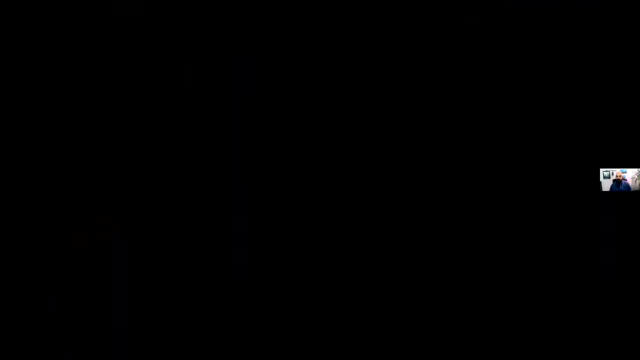 to speak to us about his PhD research. Thank you, Emma. I'm trying to stop sharing and I think somebody's got to do it for me. OK, Thank you. Let me share my screen. Here we go, All right. 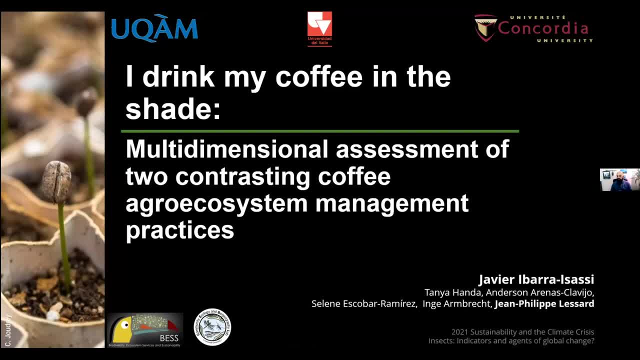 Well. thank you, Dr Duplant, for such an interesting talk. Hello everyone, I'm Javier. I'm a PhD student at Concordia, working under the supervision of Dr Jean-Philippe Lessard from Concordia University and Dr Tania Handa from UCAM. 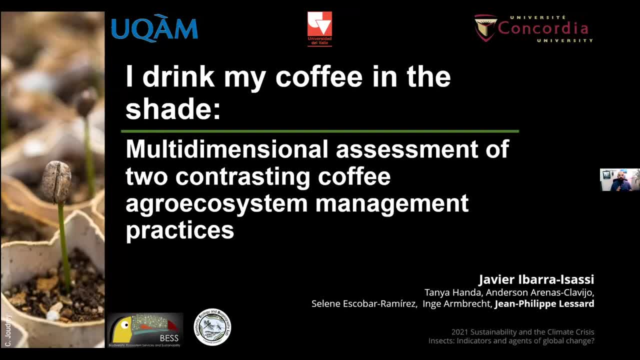 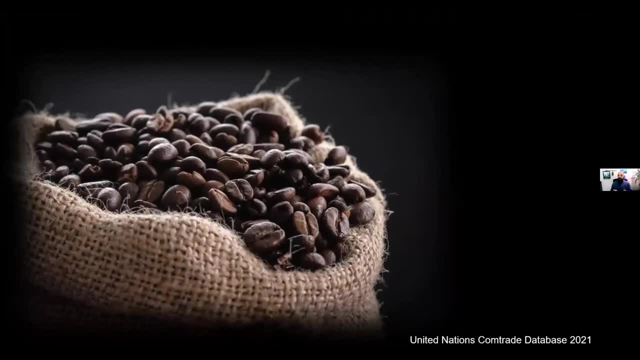 Now it's my turn to tell you a little bit of what I've learned while studying the impacts of two contrasting agroecological management strategies across multiple biodiversity dimensions. So coffee: we all know what it smells like, right? Most of us know how it looks like, and some of us 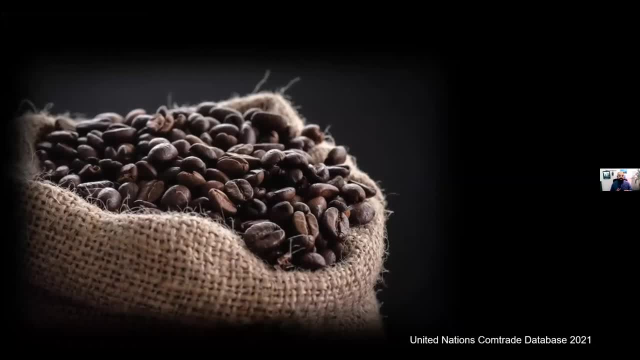 know how it tastes like, And actually some of us need it a little bit more than we would like to admit. But coffee is actually a really big deal. Next to oil, it's the second most commonly treated product in the world. In fact, Canada is one of the largest importers of coffee. 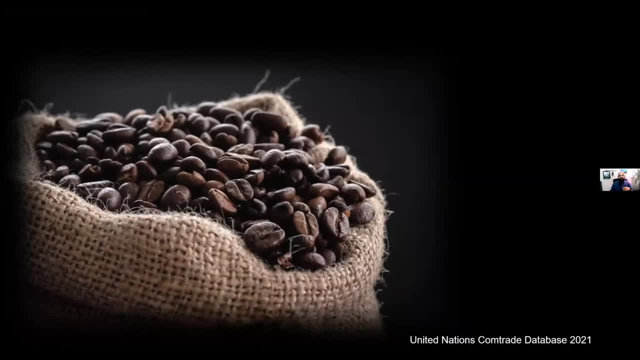 accounting for around 4% of total coffee imports In 2019.. So all of these coffee means big business for coffee-growing countries like Colombia, And in fact, around 15% of the coffee consumed in Canada is imported from Colombia. But what is the impact of coffee production on biodiversity? 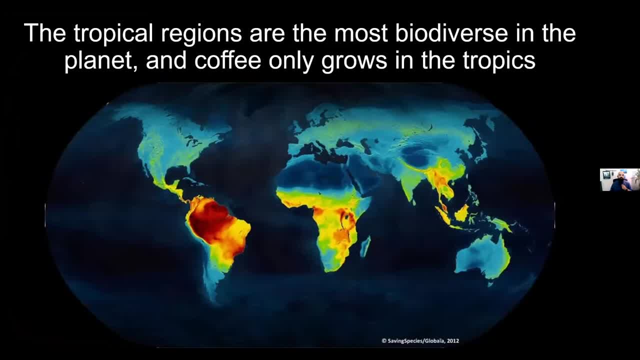 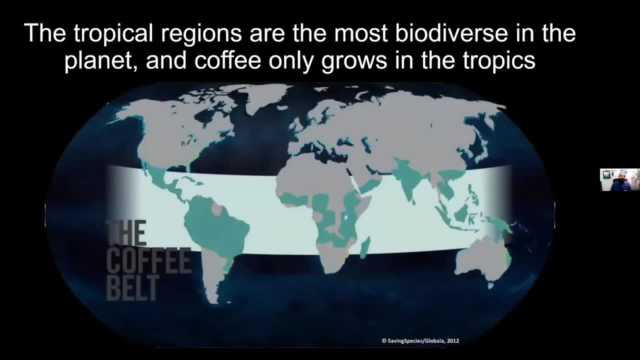 So first, we need to know that coffee can only grow in tropical regions, where we can find some of the most biodiverse habitats, And additionally, it is estimated that the yearly increase of coffee land reaches about 1,000 square kilometers, which may not sound like much. 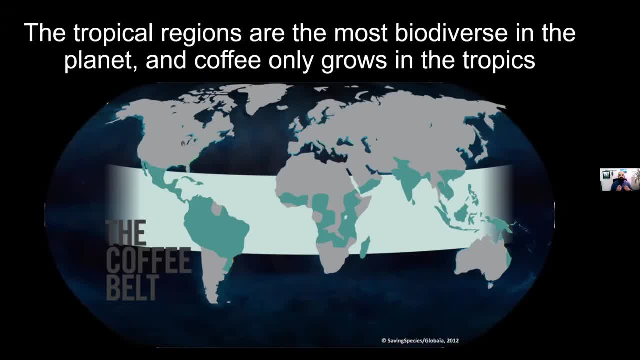 But it's actually about the size of the city of Rome or roughly the size of the island of Montreal. And this actually points at a critical issue that needs to be addressed: the habitat destruction and its associated losses, The loss of the diversity through the forest conversion. 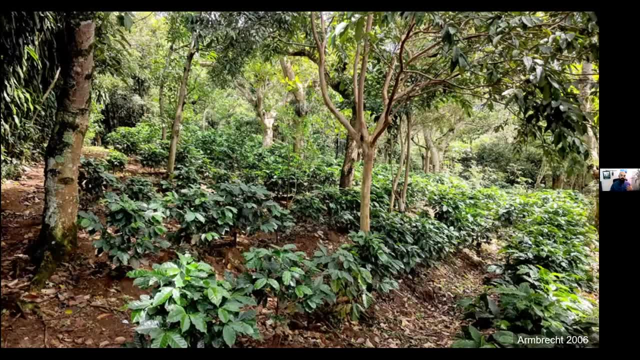 to coffee plantations. So coffee bushes naturally grow in the forest floor under the shade of tall trees, And farmers who follow traditional practices try to mimic this environment by planting coffee bushes interspersed with other trees that provide shade to coffee plants, including fruits and vegetables. 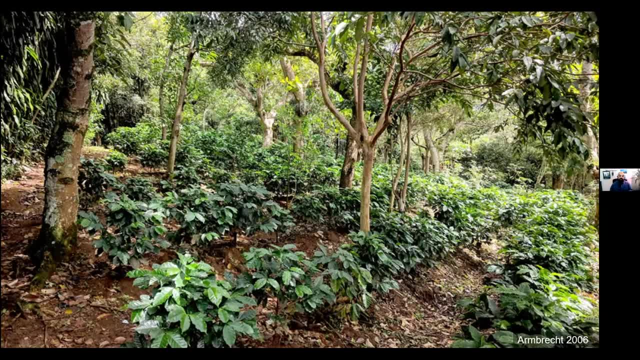 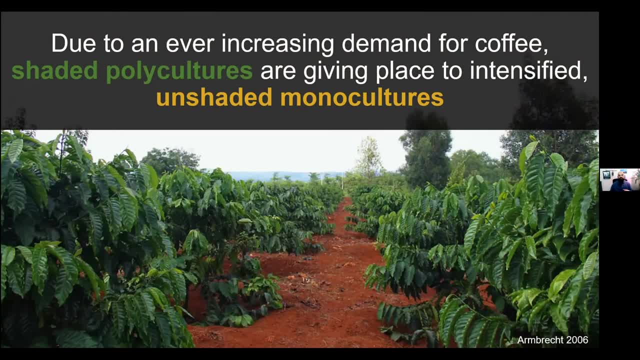 that farmers often can use to supplement their incomes. However, due to an ever increasing demand for coffee, traditional agricultural practices are giving place to more intensive practices. While traditional agricultural practices simulate the natural conditions where coffee bushes grow, intense practices do not use accompanying trees. 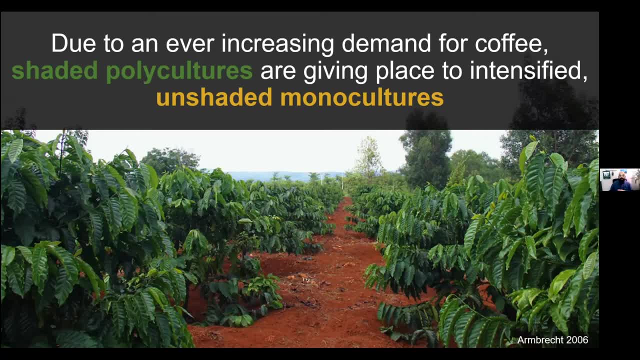 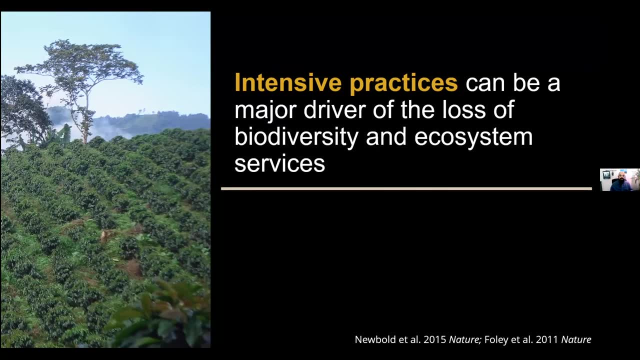 leaving bushes to grow under the full sun, providing an increased yield of coffee, but of lower quality. Also, intensive practices create different environmental conditions and have been shown to be a major driver of biodiversity and ecosystem service loss when compared to traditional practices, And this is due to this strategy of intensive practices. 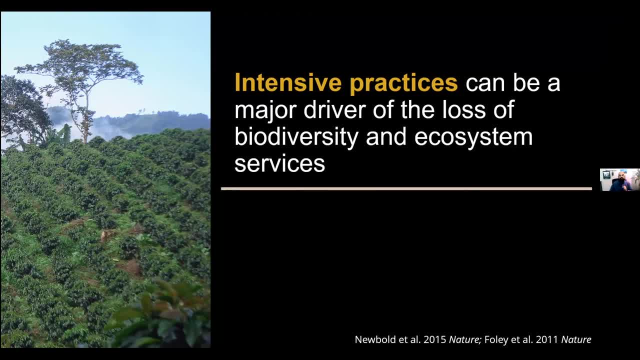 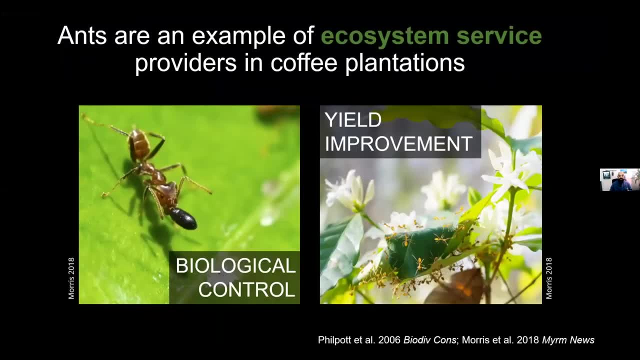 mainly focusing on the coffee bushes themselves and not other potentially important accompanying taxes such as, for example, ants- And actually ants have been demonstrated to play important roles in coffee plantations and provide important ecosystem services, So, for example, ants can act as biological control pests. 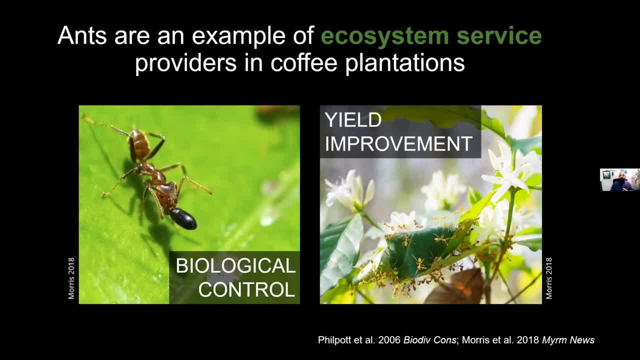 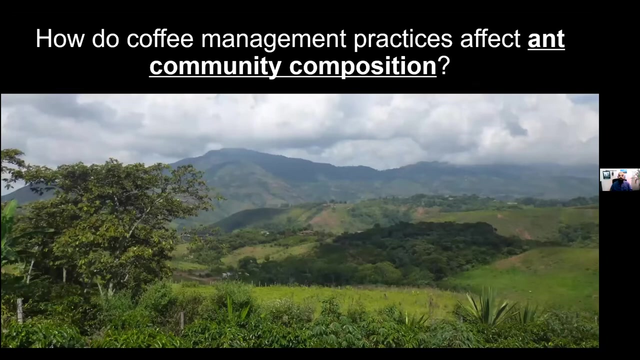 because they eat the adults of one of the most harmful pests to coffee crops, the beetle known as the coffee berry borer. So this fact can also trickle down to the improvement of yield in coffee. Now, given that different management practices change environmental conditions of the farms, 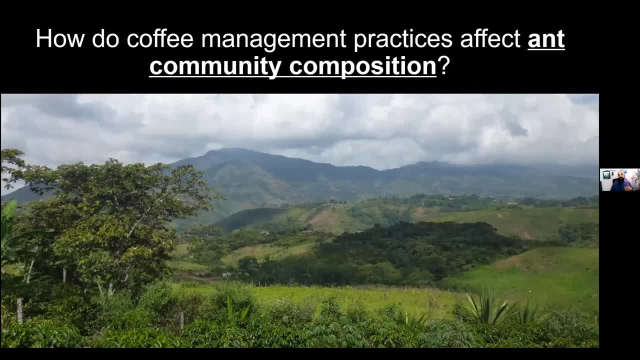 there's a natural question that arises And that is: how do coffee management practices affect the ant community composition? And we hypothesize that the ant communities and plantations that use the shade trees to grow coffee have a different composition from plantations that grow coffee under the full sun. 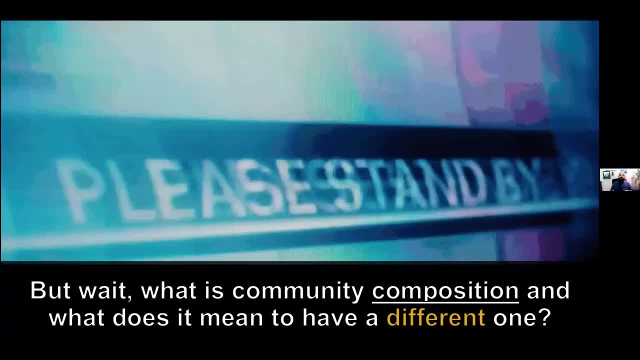 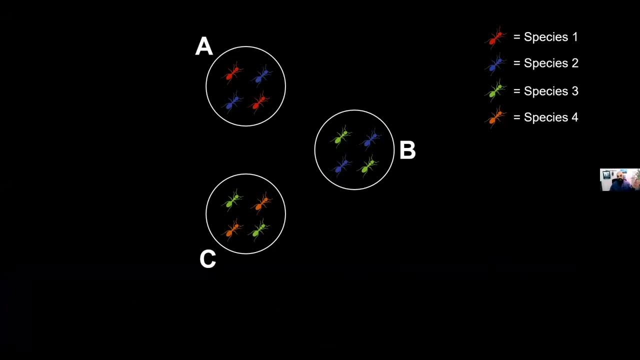 OK, But wait, what is species composition And what does it mean to have a different composition? And first picture three sites, A, B and C, with two species each, And which species are in each site is the composition of the community at each site? 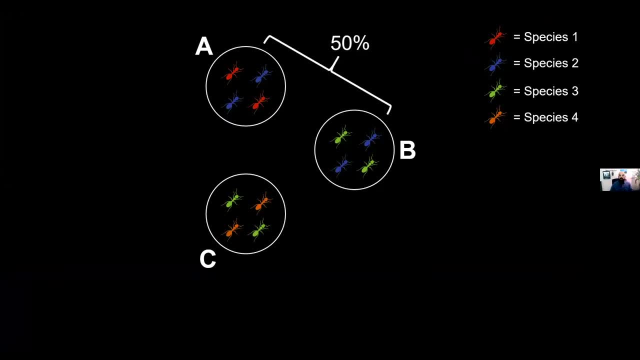 So when we compare sites A and B, we see that they have one species in common, or that they, in other words, we can say that they also differ in one species. On the other hand, if we compare sites B and C, 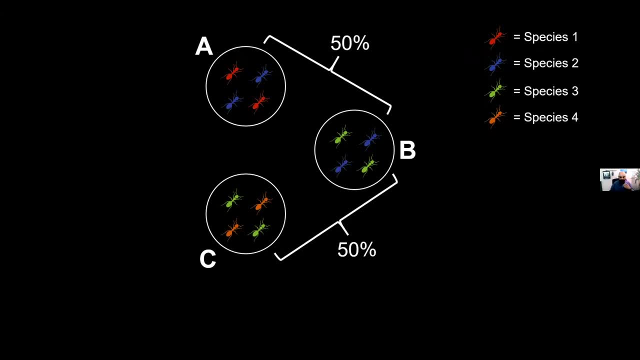 they also share one species. But now, when we examine A and C, we see that they are 100% different, that they share no species at all, And so we can evaluate how different variables can affect these composition differences. And after this brief information, 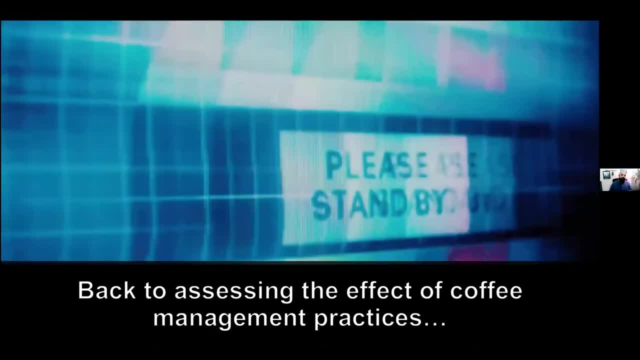 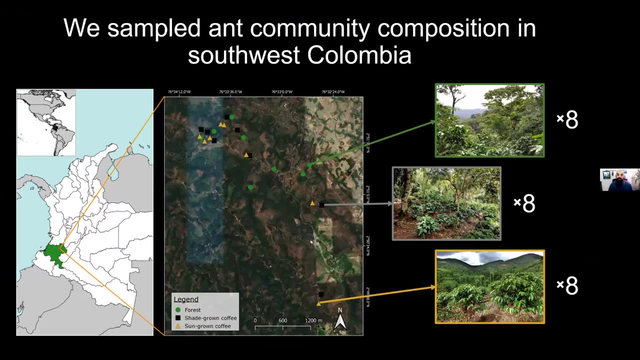 let's get back to assessing the effect of coffee management practices. All right, So to answer our question of how do coffee management practices affect ant community composition, we sampled ant communities in southwest Colombia And so to contrast the management practices, we sampled ants and several environmental variables. 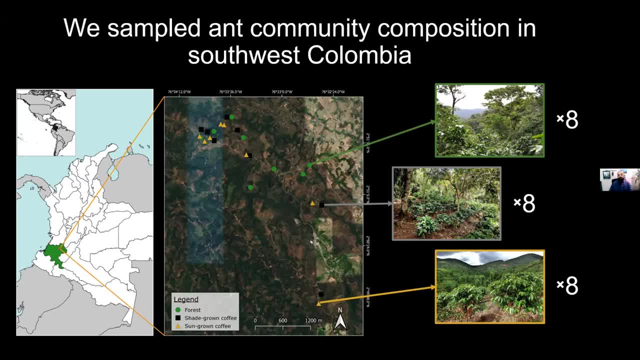 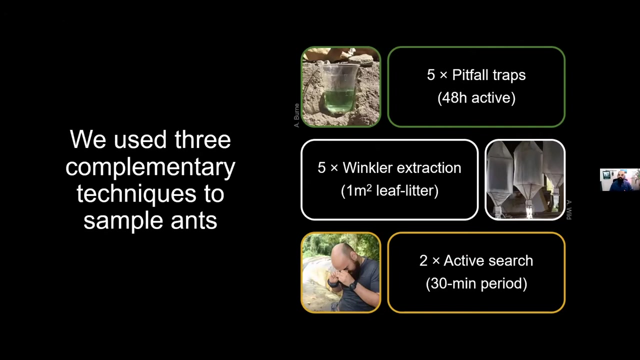 like soil temperature and humidity, in eight shade-grown coffee plantations and eight sun-grown coffee plantations that otherwise followed similar management styles. And to establish a comparison point to more natural communities, we sampled eight forest patches in the nearby area. So to collect ants we used three complementary sampling. 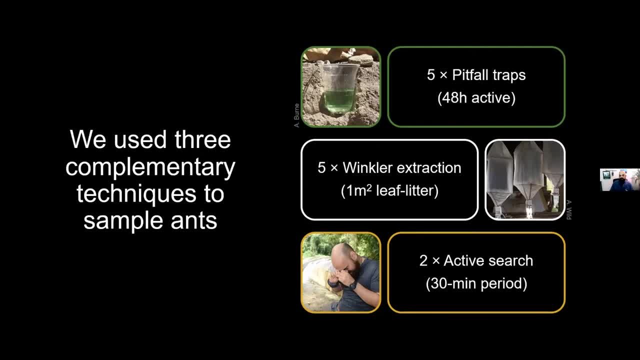 techniques that have been shown to capture most ant species present in a particular site. So we used five pitfall traps that were active for 48 hours, five one-square-meter leaf litter wrinkler extractions and 30 minutes of active search. so basically active looking. 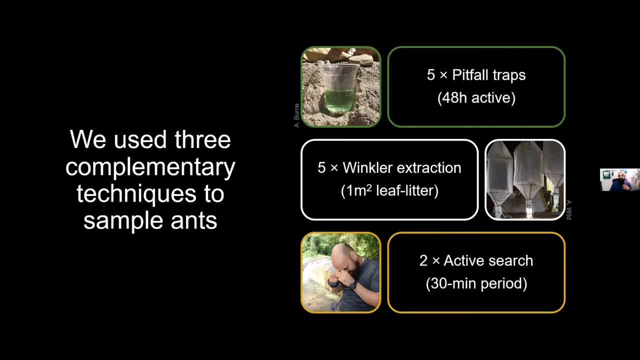 and then we collected the data, And so we sampled twice, once in August 2015, and then once between December 2015 and January 2016- on each of the sites, And, after processing our samples and identifying and counting all the ants that we collected, we 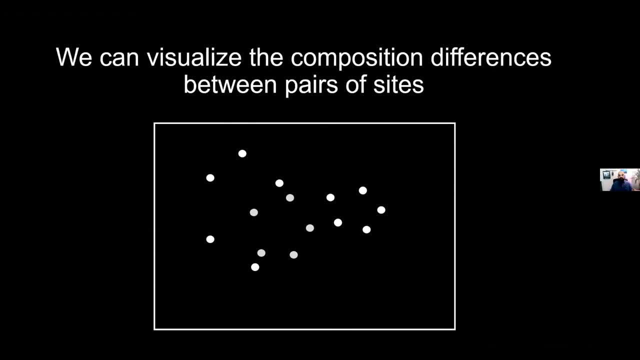 had to visualize differences between each pair of sites based on how strong the differences are between them. So here each point is a site and the difference and the position of it in the plot is determined by how similar or dissimilar the relation they are in relation to other sites. 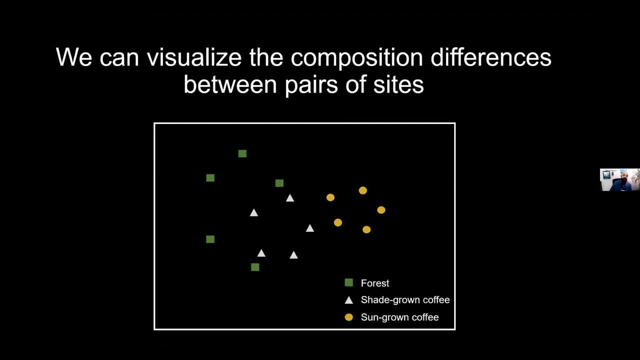 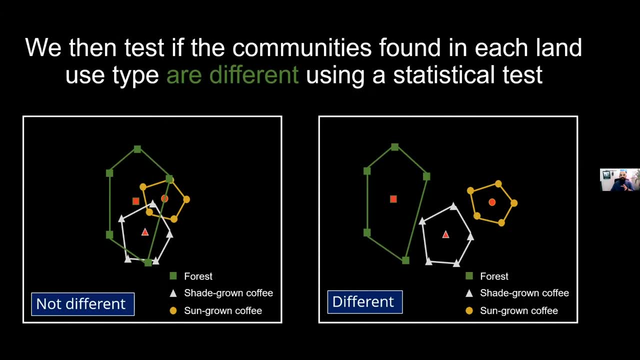 And we can identify each plot per land use to make it easier to interpret, using different shapes and or colors, And we can then test if these communities found in these plots are different using statistical tests that evaluates if species composition is equivalent between all land use types, meaning that we would expect. 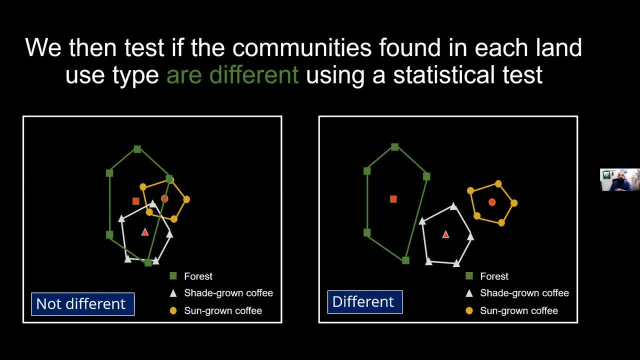 to find the same ant species composition regardless of the land use type. So we would see the pattern on the left when the species composition per land use is the same and the pattern on the right when they are different. We also tested how homogeneous these communities. 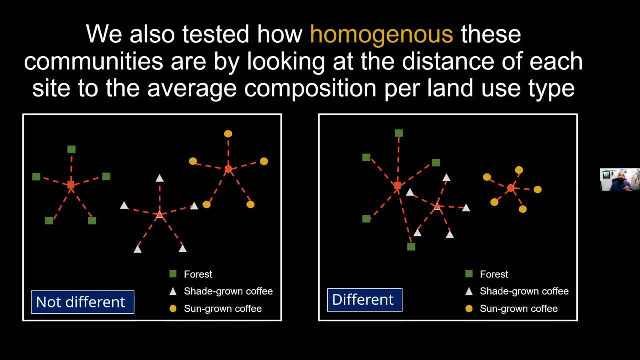 are by examining the distance of each plot to the community composition average per land use type. So if communities are homogeneous, then this means that in practice it would mean that if we were to walk from one site to another in the same land use type, 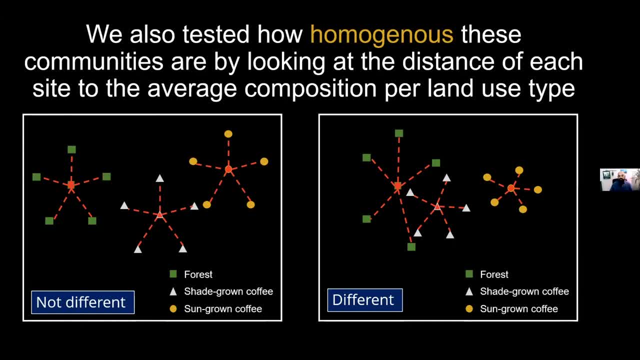 there's a high chance that we will find the same species composition. So, like before, we would see the pattern on the left when the species composition homogeneity within each land use type is the same, and the pattern on the right when they are different. 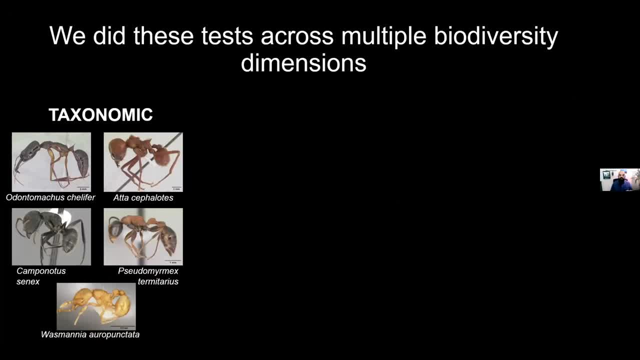 And so, to get a comprehensive idea of how these contrasting agroecological management strategies affect biodiversity, we examined the effect across multiple biodiversity dimensions, And the first one is the taxonomic dimension, or basically the identity of the species found in each site. 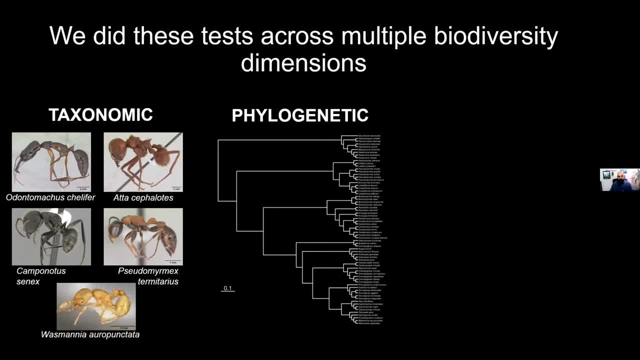 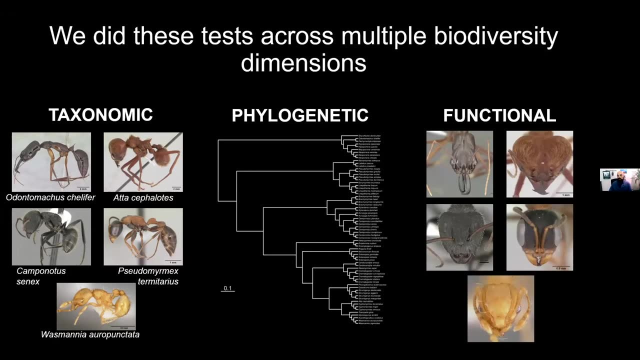 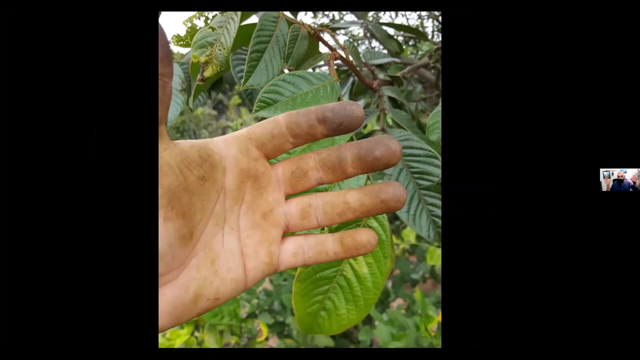 We also evaluated in the functional phylogenetic dimension, which means that we examined the evolutionary relationships among the species found in each site and also the functional dimension, or basically the different potential responses and roles that species have in each site. Now, after getting our hands dirty and our brain wheels, 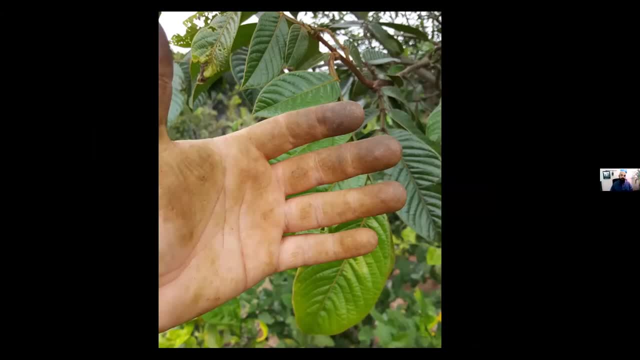 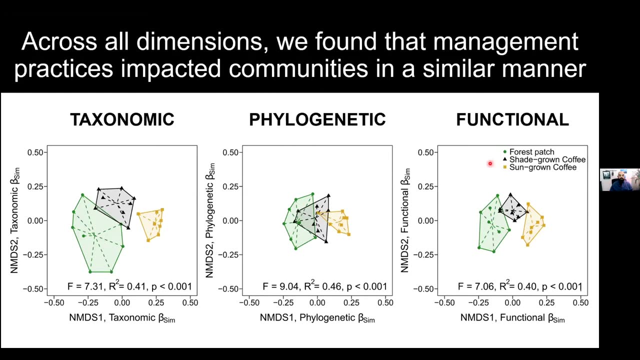 turning. here are the results of our analysis And here you can see the visualization of the community composition differences across the three dimensions. And each plot is identified per land use type. where you see green circles are forest patches, black triangles are shade-grown plantations. 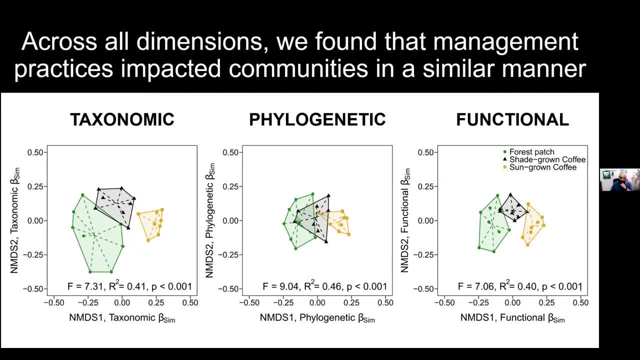 and yellow squares are sun-grown plantations, And so when we analyzed differences in species composition across all dimensions, we found that land communities found in shade-grown coffee plantations are more similar to those found in forests than to those found in sun-grown coffee plantations. 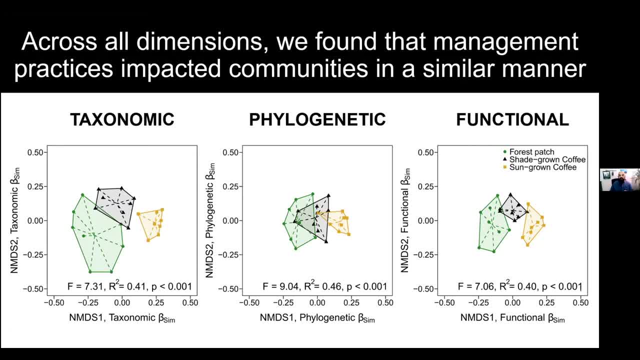 Also, When we analyzed how homogenous they were, we found that the communities that occur in sun-grown coffee farms are more homogenous than those found in shade-grown farms and or forests. In other words, remember that homogeneity means that if we were to walk and sample ants, 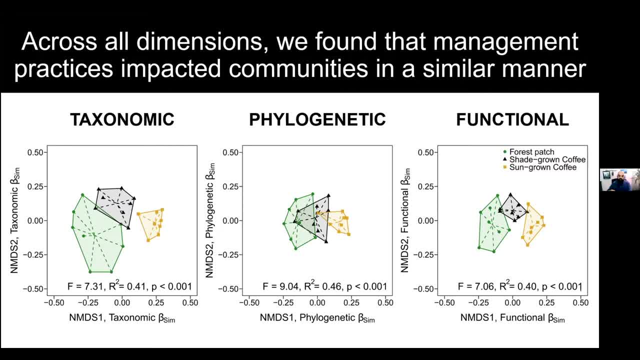 from one sun-grown coffee farm to another sun-grown coffee farm, it is more likely that we will find the same ant species with the same evolution, And so we found that, in the same way that we were able to find the same ant species with the same evolution. 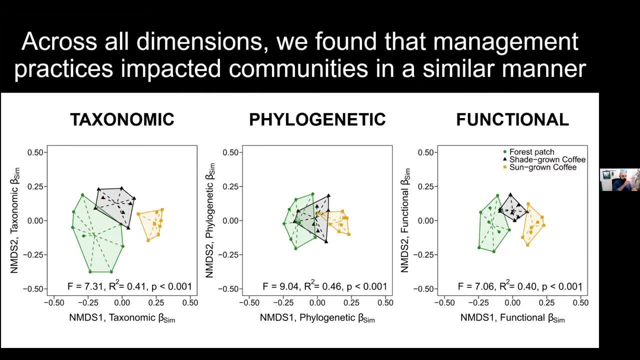 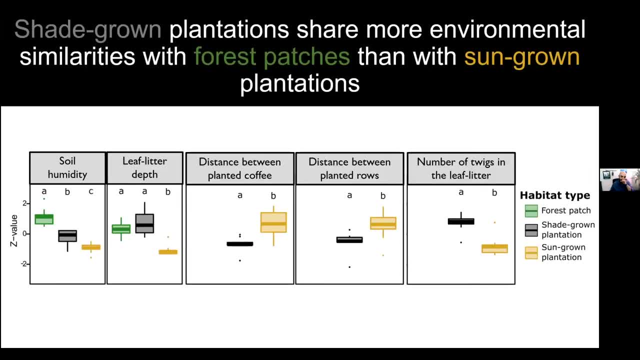 in the same way that we would if we were to walk and sample ants from one forest to another forest or from one shade-grown coffee farm to another shade-grown coffee farm. And to better understand what was driving these compositional differences, we analyzed how some environmental variables were different. 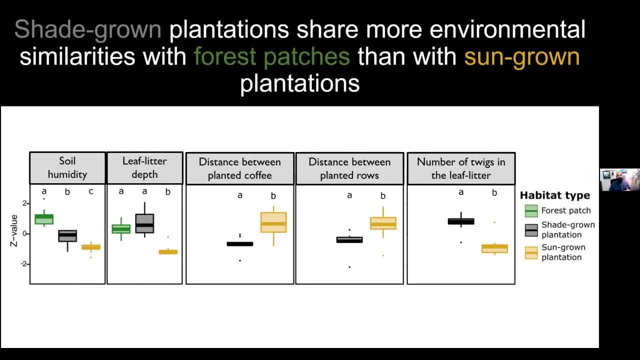 between the different land use types, And so, after doing this, we found that shade-grown plantations, for example, share more environmental similarities with forest patches than with sun-grown plantations. So, besides having trees, providing shade to the forest floor, 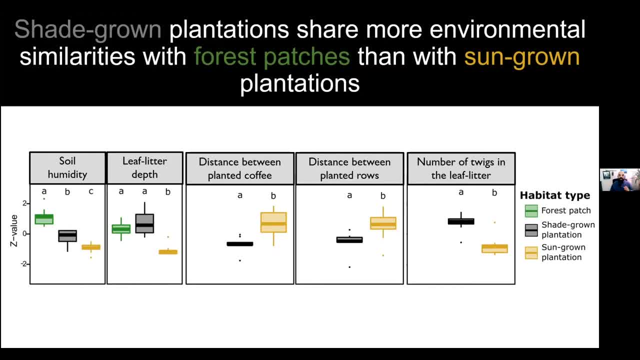 forest patches and shade-grown plantations have similarly deep and humid leaf litter relative to sun-grown plantations. Also, shade-grown plantations had higher crop density and the number of twigs in the leaf litter. These differences in the soil and soil 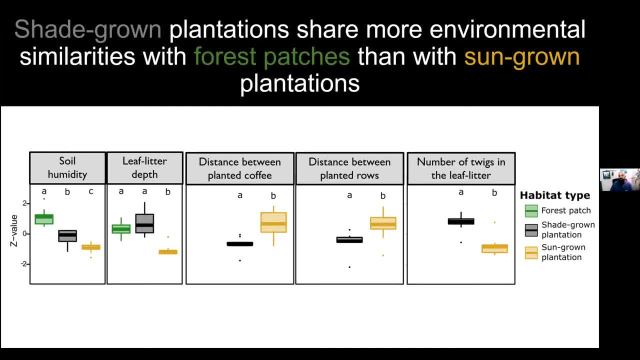 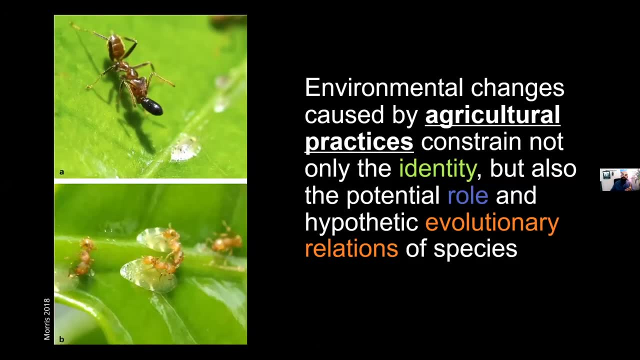 and management characteristics are the ones that are driving the compositional differences between the habitat types, And this actually corroborates the results found in previous studies in the region. Now, to conclude, our results suggest that the environmental changes used or caused by agricultural practices constrain not only the identity 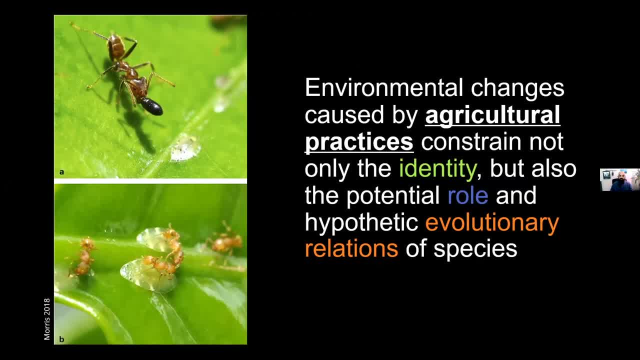 but also the potential role in hypothetical evolutionary relationships of species. Thank you, Thank you. And this is evidenced by the fact that coffee farms, regardless of management practices, they harbor and communities that are taxonomically, phylogenetically and functionally different. 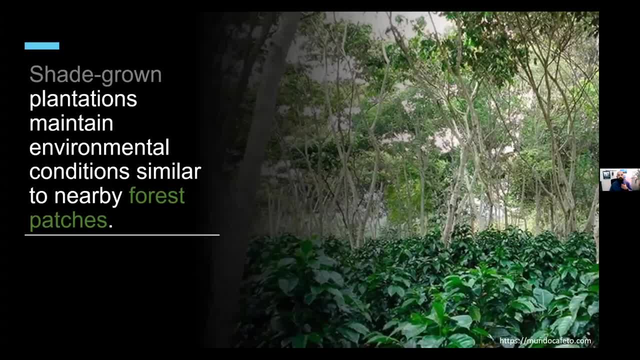 than those of forest patches, And also our environmental analysis allowed us to identify that shade-grown plantations maintain environmental conditions that are similar to forest patches, which would lessen the impact of habitat loss in coffee plantations. So Farm managers should try to mimic these forest-like leaf litter. 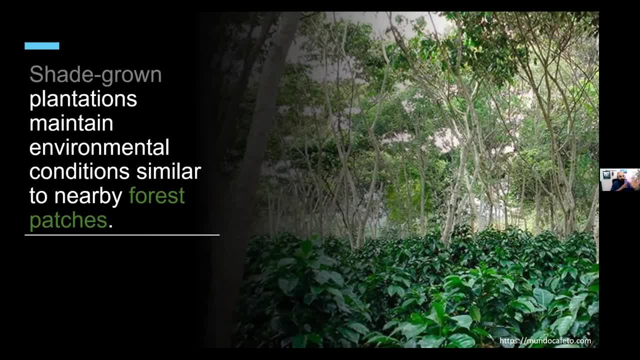 conditions to help mitigate the loss across multiple biodiversity dimensions. So, maintaining or increasing leaf litter depth and twig number below the coffee bushes could be used as a strategy to conserve and predation services, because these conditions can favor the persistence of the specialized ant predators that could act as pest biologists. 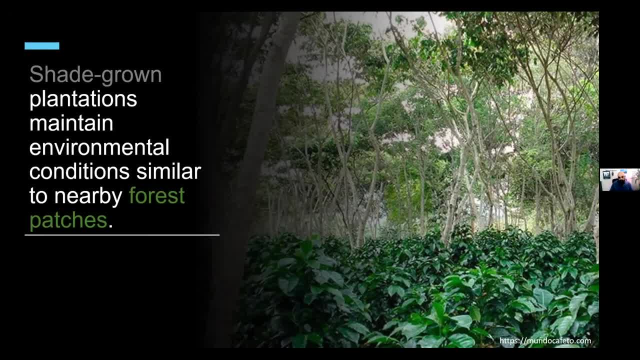 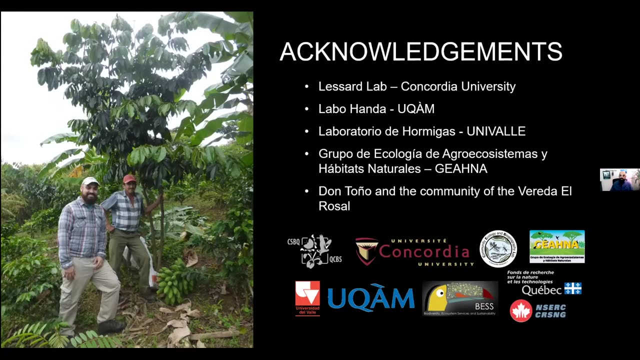 And finally, these practices would not only benefit ant diversity, but numerous additional benefits may come in directly from ant conservation-oriented practices, And with that I would like to thank all of our collaborators and funding agencies that made this research possible, And a special mention to Antonio, who 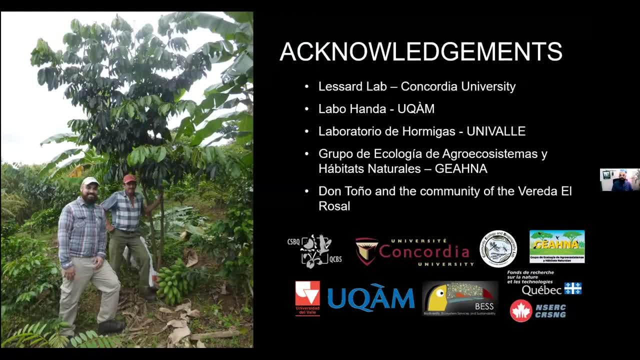 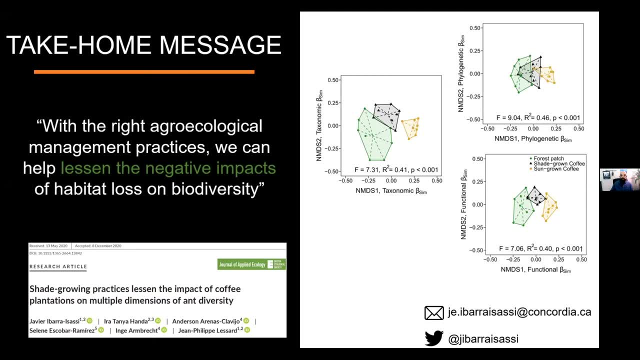 is a person who tirelessly works taking care of these coffee plantations and is very eager to learn and help during these type of activities. Thank you, And, of course, thank you for your attention, And I would just like to leave you with one key message that we learned from our study. 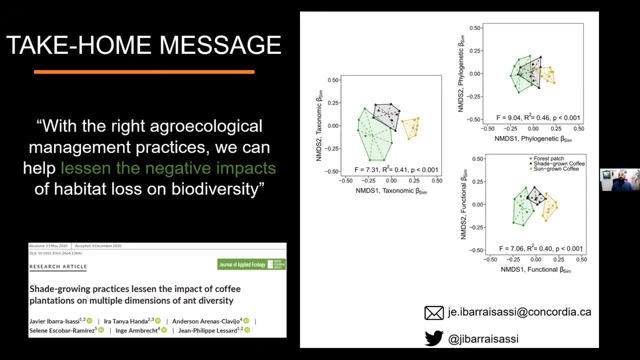 that, with the right agroecological management practices, we can help lessen negative impacts of habitat loss on biodiversity. And if you want to read more about this study, we recently published it in the Journal of Applied Ecology. And so, finally, if you have any other questions, 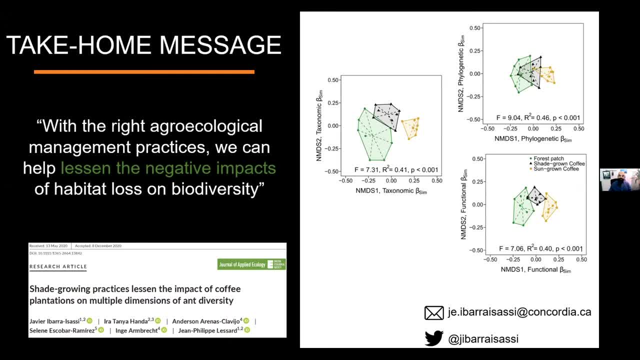 feel free to send me an email or contact me through Twitter, Thank you. Thanks so much, Javier. Does anybody have any questions? before we move on, Just quick points of clarification. at this point, We do have a question from Carly, who says great talk. 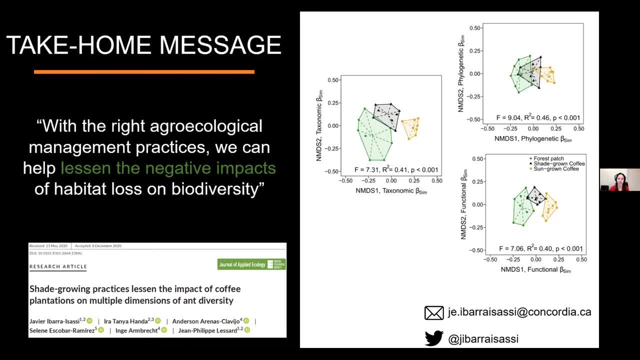 I'm glad I buy shake-grown coffee. I have a question of: oh, I can save this one for the end. Sorry, I just caught the second part of that question, So we'll save it for the end. Maybe it's a question that would be better asked to everybody. 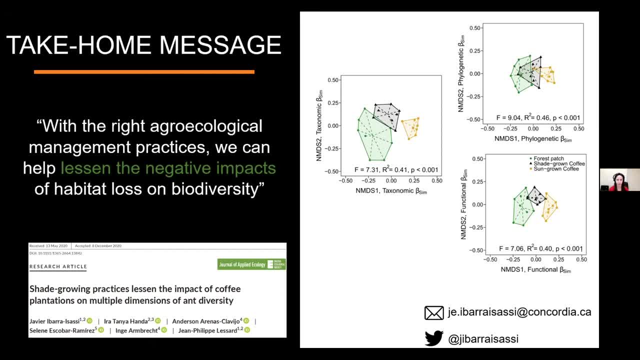 So if anybody has a question, that would be just a point of clarification for Javier at this point. How much of the problem are the consequences just fine or really a concern? So the consequences of not having shake-grown coffee, how serious is this? 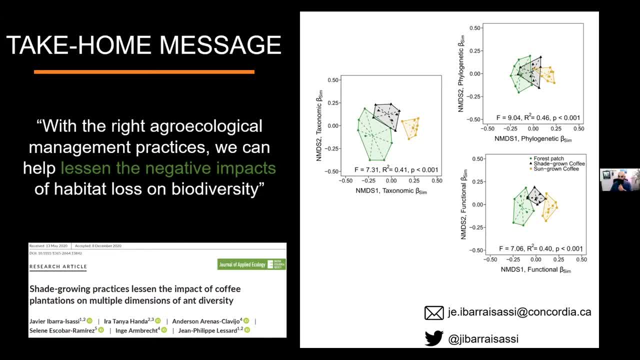 I think that's what's meant by this question, Right. So right now it's definitely a concern, for sure, But it can become a real problem, Right, Because we're seeing that communities or diversity in general, we're losing a lot of diversity. 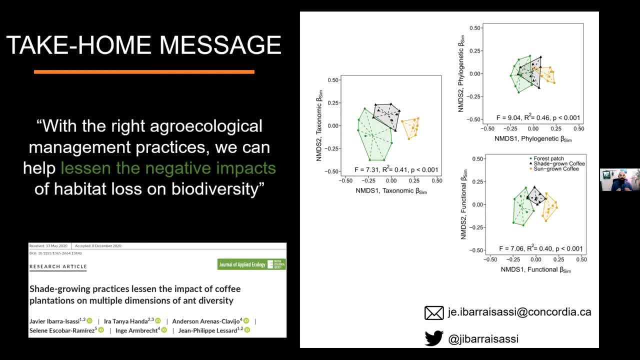 And what's important here is that we're seeing that we're not only losing species, We're also losing a little bit of the evolutionary history that those species have and also the potential roles that these species might have in these ecosystems. So it's very important that we keep doing. 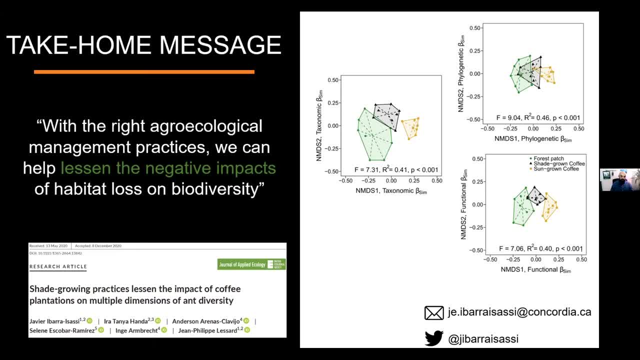 keep monitoring these biodiversity laws caused by intensive practices And we potentially can start adapting or mitigating these laws by introducing or integrating these different biodiversity dimensions into the management strategies. I'm sorry I've been on mute. Thank you, Javi. I have another question from the audience. 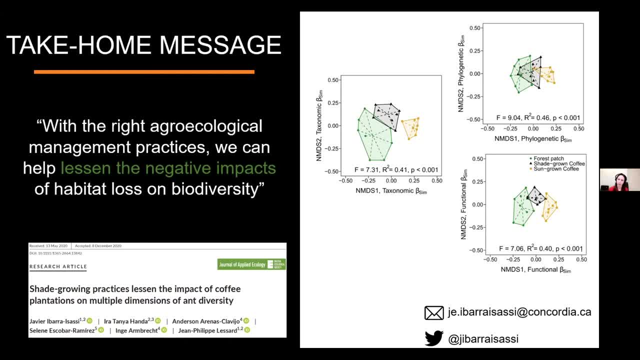 from Kim Gomery, who asks: beyond coffee plantations, what lessons can city dwellers and gardeners draw from the ant experiment? That is an excellent question, And what we can do is definitely be aware of what type of coffee we can. 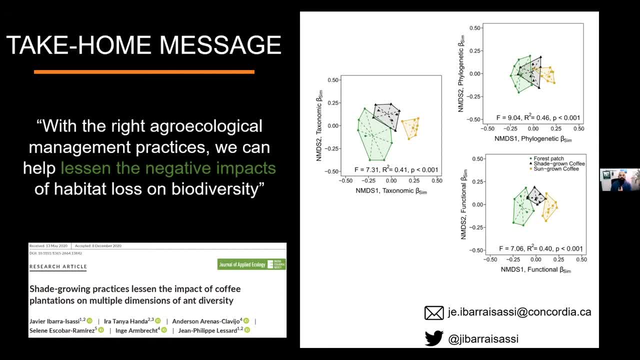 consume or what type of food we consume. If we are a bit more aware of this, we can buy things that come from sustainable sources. Or let's just take the coffee. to make it more precise, If you buy coffee that is grown under the shade, 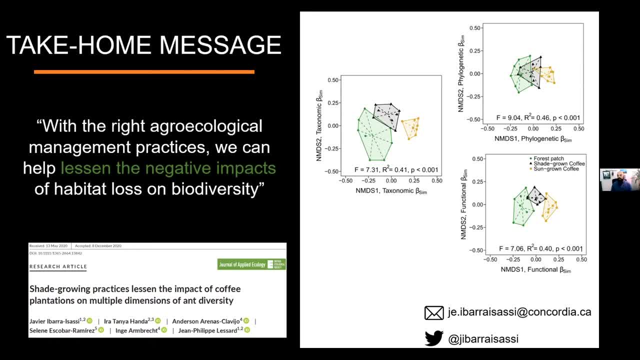 you are promoting these more sustainable practices, And so that's something that we can learn from this, And if you're a gardener, you can see that there's something that we have a bad image about ants, And so if we find ants in our garden, 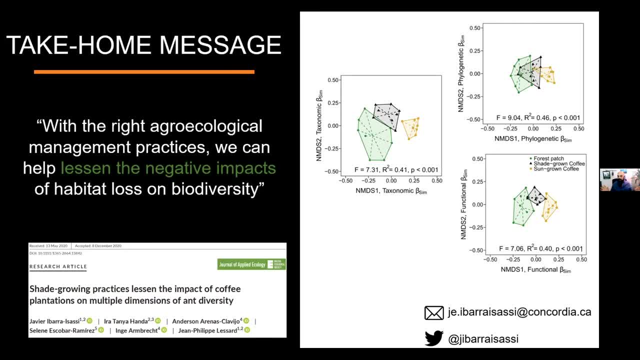 we immediately think, oh, it's a pest, Let's kill it, Let's get rid of it. But no, ants actually have many different important roles in nature that we are still trying to learn more on how we can perhaps use them to better take care of our ecosystem. 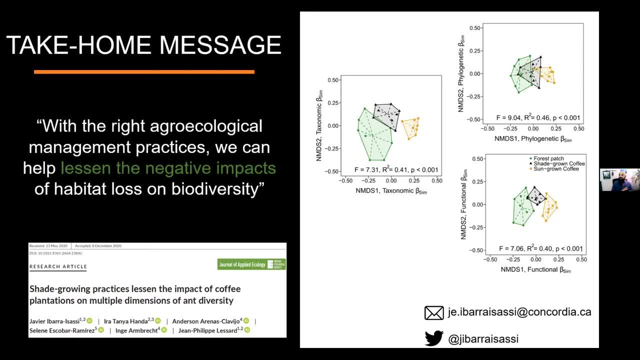 So maybe, as a gardener, you know, don't immediately consider ants as pests. Don't kill them, because they might be working in your favor. Great Thank you, Javier. There are more questions, but we do need to move along to make sure. 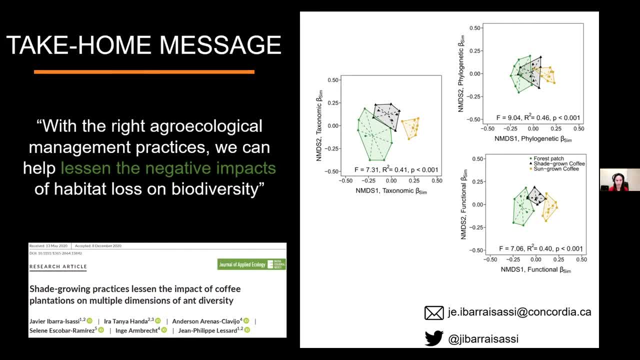 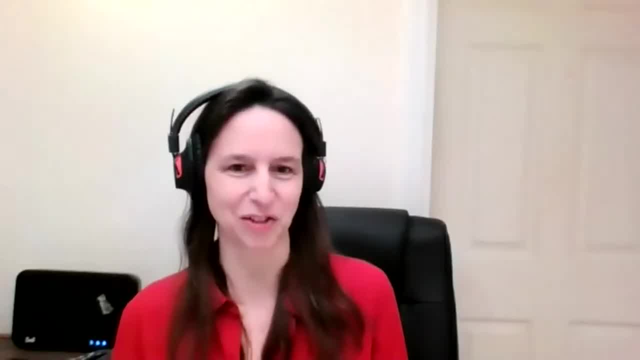 that Pamela has a chance to give her presentation as well, But we will take more questions at the end And if you have a question that's typed into the Q&A, it will stay there until we have addressed it. In the meantime, Javier, if you feel like you can address, 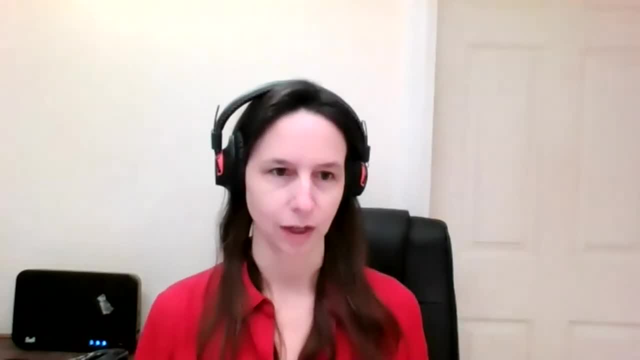 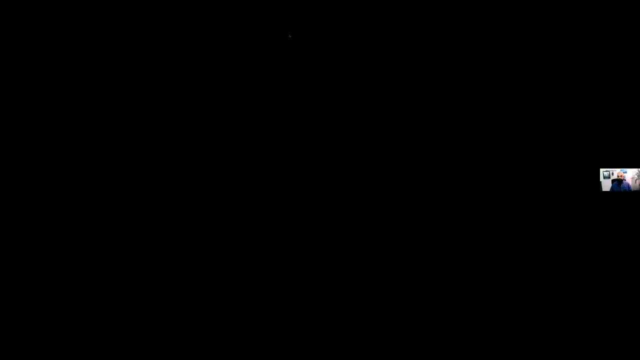 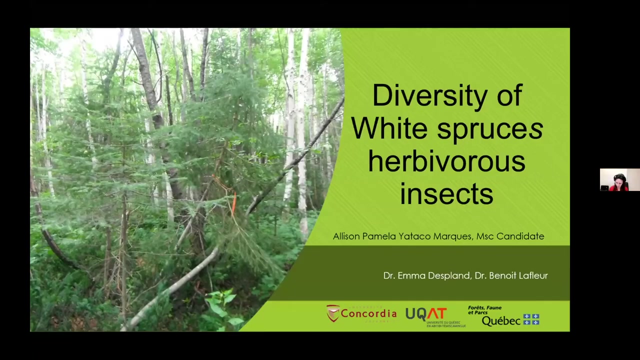 any of those questions in writing. you can do so At your leisure. Thank you so much for your presentation, And I'll invite Pamela now to share your screen and share your presentation. Yes, I'm on it, All right. All right, so I'll be presenting my thesis, that's. 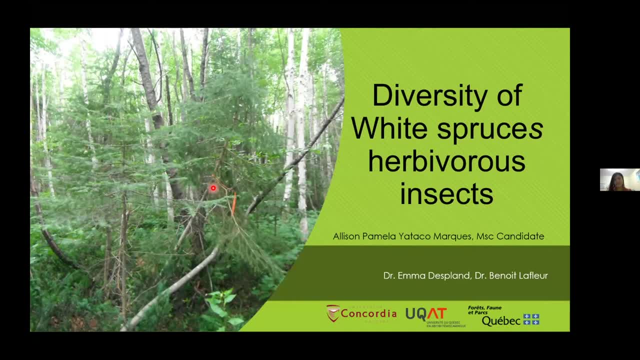 on insect herbivore diversity of white spruce plantations. So this is my master's Thesis. I'm working with Emma Deplan as a master's student. I'm also working with Benoit Lafleur, who is from UCAT. 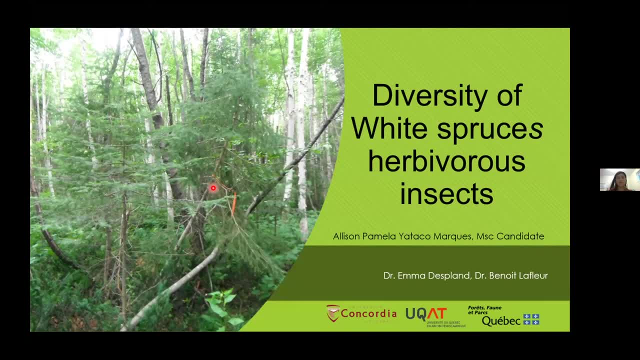 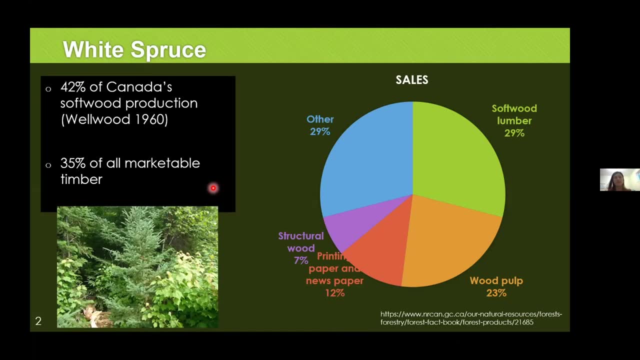 He's my co-supervisor and is being funded by the MFFP. So, first of all, why is white spruce important? So white spruce is an important source of production of softwoods. So softwoods being used for like sofas, for a lot of like, the production of like. 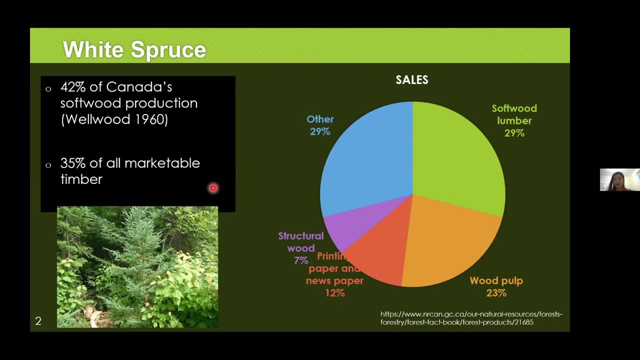 materials for Canada And it's also very important for the economy. It's 35% of the marketable timber And there is a lot of like- 29% of like. the whole wood production is softwood lumber, So these trees are being affected negatively, as I think Emma mentioned. 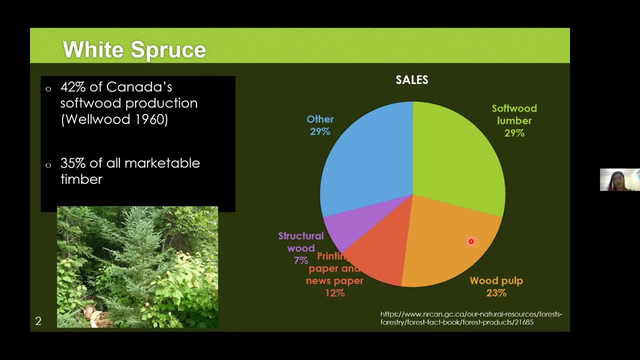 A lot of these pests, insects like out-breaking insects that like can come in. So in the region that I'm studying, Abitibi, there is like a probability that the spruce butt worm that was mentioned would infect this area. 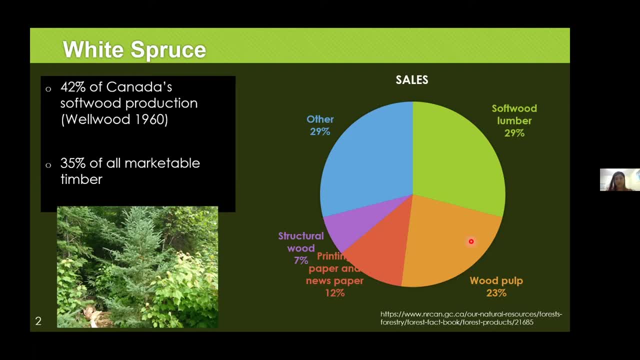 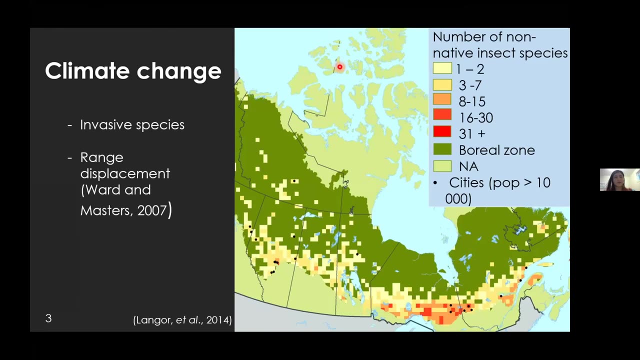 And it's like been affected before. So right now, what can we do to like manage these plantations in the future, with the climate change Kind of like happening over time? So one major concern is like, of course, invasive species. 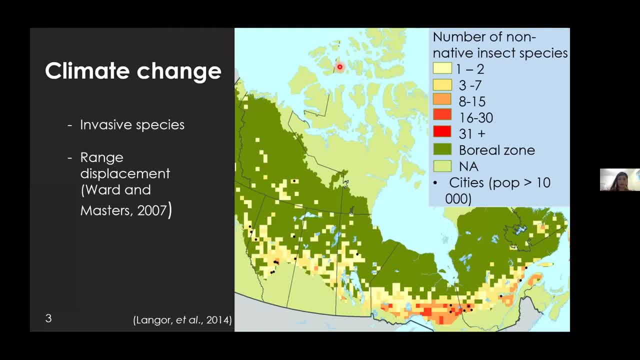 because warming of like the environment can cause a change in the range in which species can occur, especially non-native ones. Here we see kind of a spread of the non-native species currently, right now. So if, like, warming would actually really cause a lot of these to kind of move. 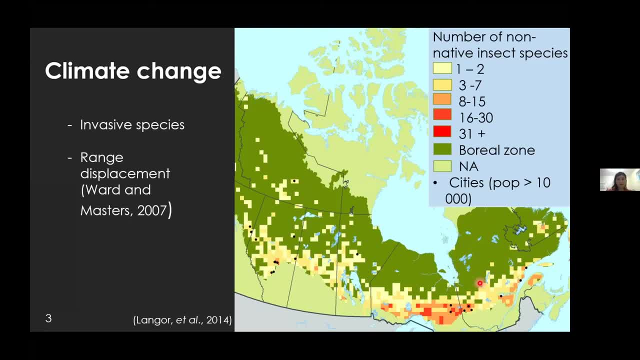 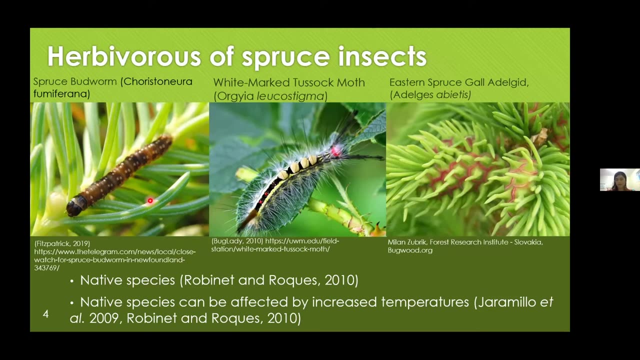 more towards the north. So we were wondering: OK, so we know that this can be a danger. How will climate change also affect native species? Because these guys are kind of an example of like the native species of the whites, like Canada. 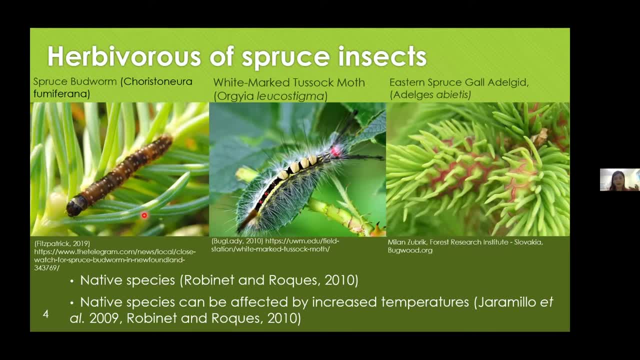 We know that already that spruce butt worms being affected by like climate change, like occurring, like more of these unstable like outbreaks. We don't know what's happening, But we'd like to know would this affect other like? 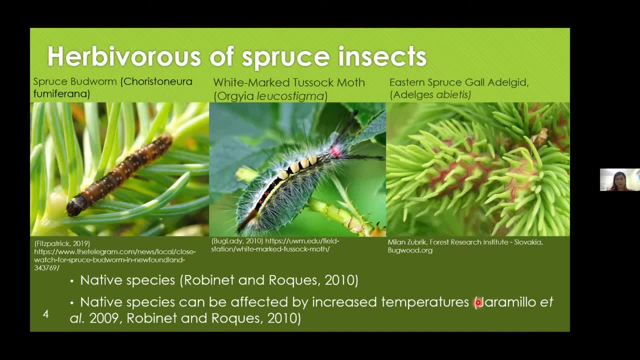 native species that might maybe not be so like obvious to us that could possibly be a threat. So that was my job. So why we are doing this is because, like there are studies that show that, like, for example, some groups of Lepidoptera like Nocturnidae- 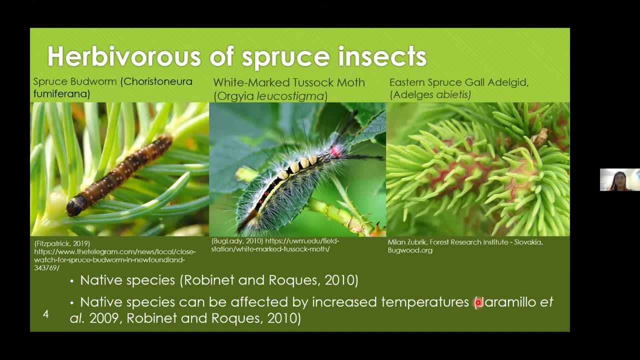 can do better in warmer climates and will reproduce more, And also warming of like of the northern region can weaken the trees and cause higher like levels of defoliation and, yeah, and damage from other insects. So because of this, we'd want to know like which species are. 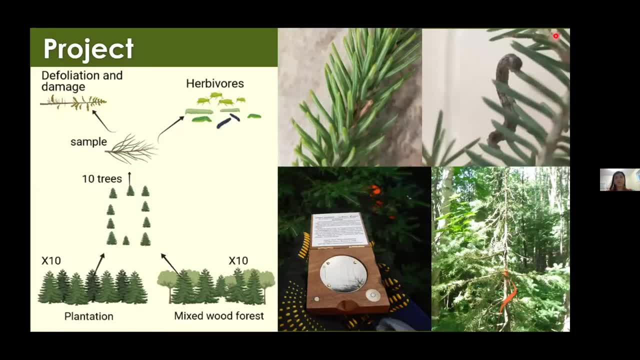 going to be The ones like affecting this in the future. So my project: we went out into Abitibi, the furled station, to sample plantations which are like this: They're just pure white spruce, They're kind of short. 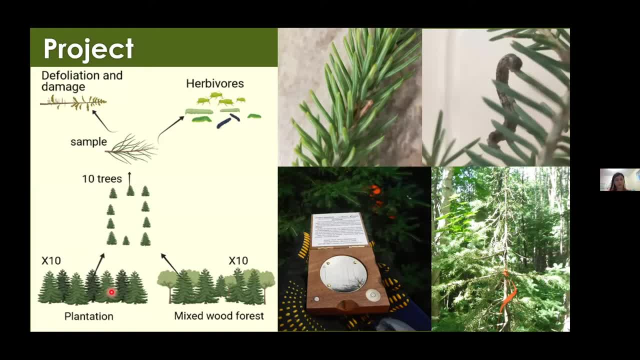 Like we sampled shorter trees around three meters. They have a very open canopy, lots of sun exposure. So, although it might not be completely like, maybe a predictor of how Like an insect will do also in warm environments. 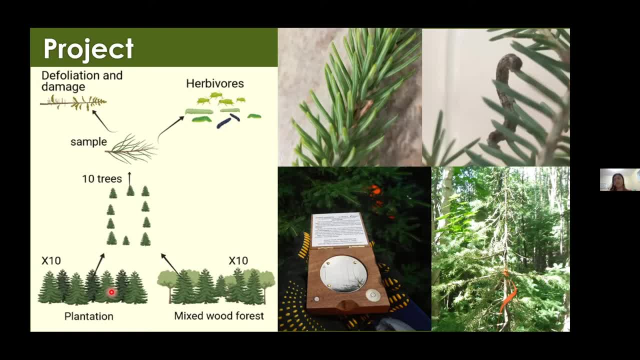 it's like higher temperatures and sun exposure is a factor that affects the populations there, And we also sampled those wild trees like this example here that are in mixed with forest, And these grow a bit slower in mixed with forest, So the age might not be exactly the same. 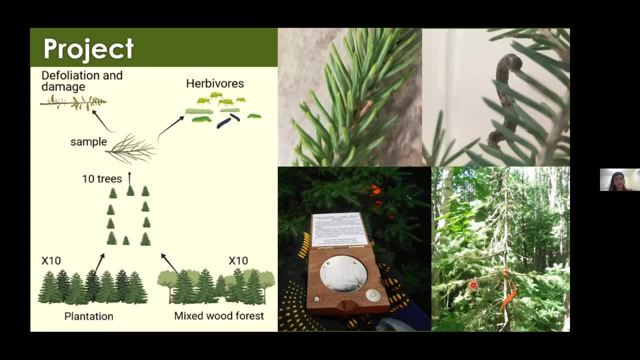 but we sampled around the same height And I chose 10 trees from each. I got one branch And from there I sampled herbivory diversity and foliation levels within like the branch. So we got the percentage of the foliation. 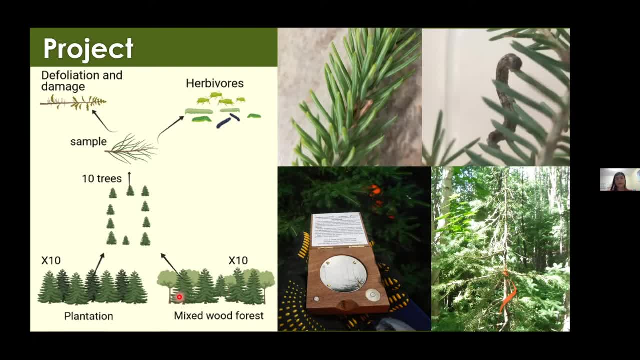 and like the different damages that we found as well. So this is kind of an example of a needle miner And this is an example of like a measure of the canopy openness that we did in these two areas to measure also. 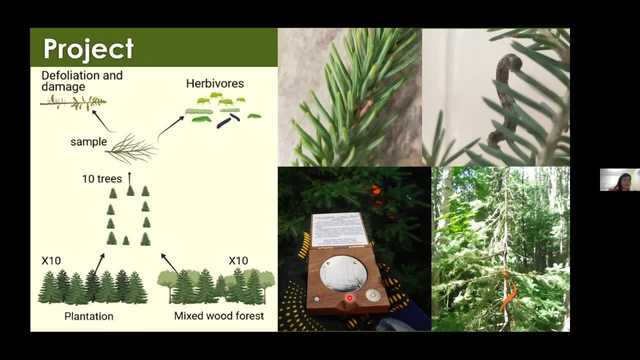 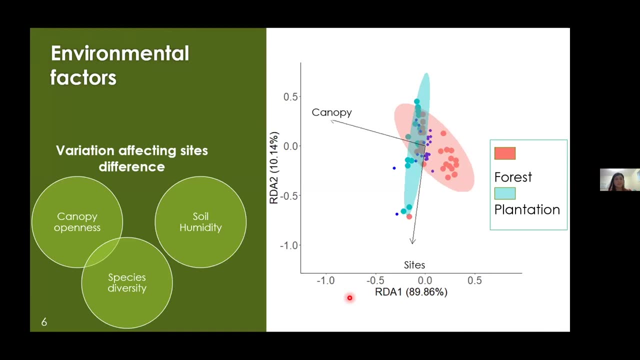 other environmental factors Such as canopy, openness, humidity of the soil and so on. From this like kind of population data that we got, we went on to do some analysis And this is a bit complicated. I tried to simplify the concept of kind of removing. 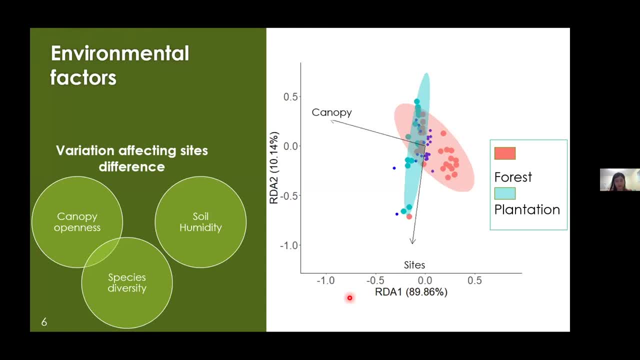 this environmental factors, from the diversity data by kind of this Venn diagram. So when you have like the like diversity set for one treatment, let's say like forest, it'll give you. I think also, as Shafi mentioned, 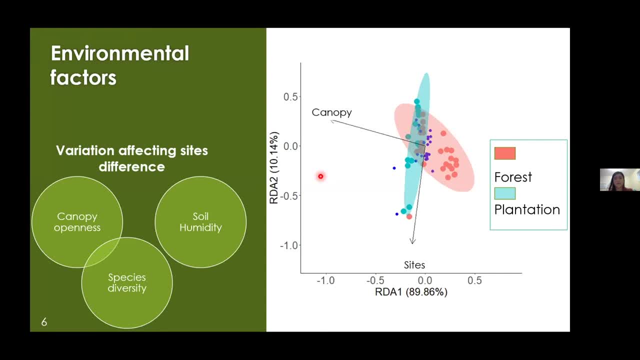 a point here within like statistical space And it kind of shows you how different each site is from one another, So you can kind of get the correlation. So we kind of tried to remove canopy openness. Soil humidity didn't really affect it in the end. 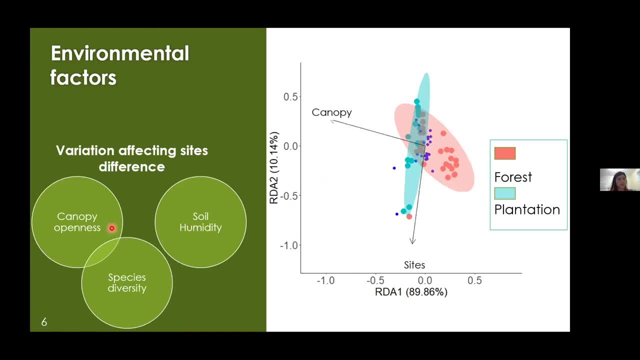 So It's not really needs to Education, Even though we tried to remove it Can. yeah, that was it. Yes, Alright it, and didn't really change the dispersion and in the end, this is what we got for: only herbivore. 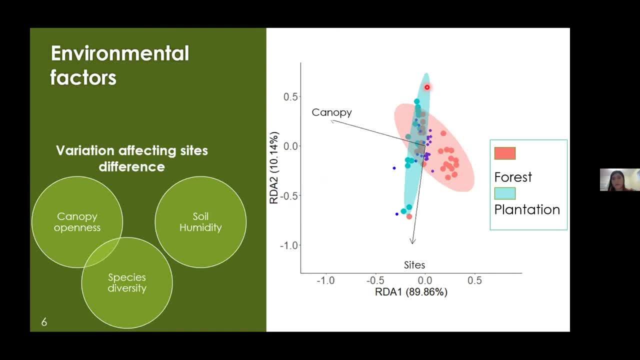 uh, diversity. so we saw that in plantations which are in blue, um, it's like, very like, there's a lot of like it varies a lot from forest site um, forest, uh like, yeah, sites, um, and this, with another analysis, was shown to be mostly driven by adult jits and aphids. uh, algis are. 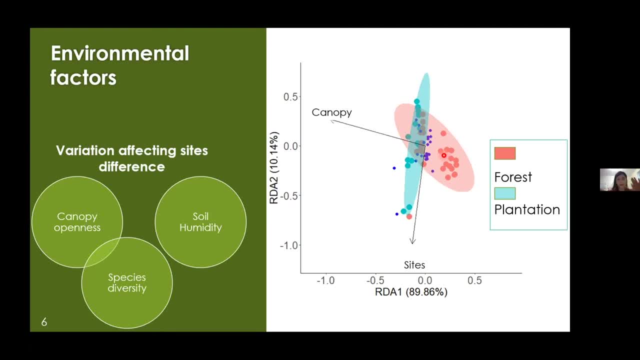 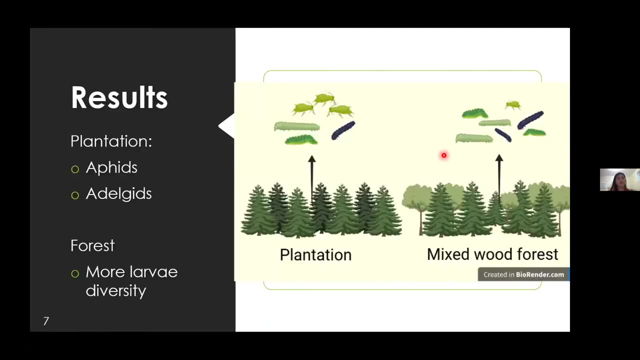 the little creatures that can form that pineapple shape that i showed earlier in the screen. so from like this is only for um herbivore diversity, for total diversity. it was another result and i'll i could talk about it later. so, um, we'll talk about the results. 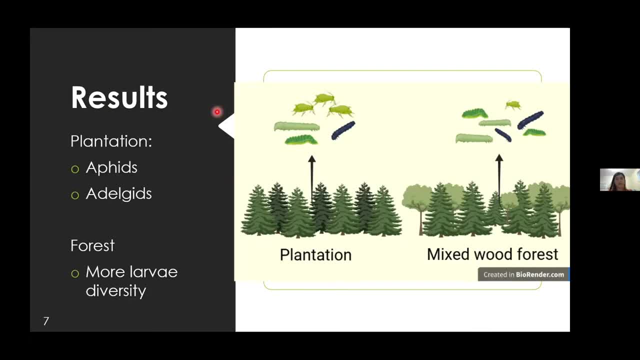 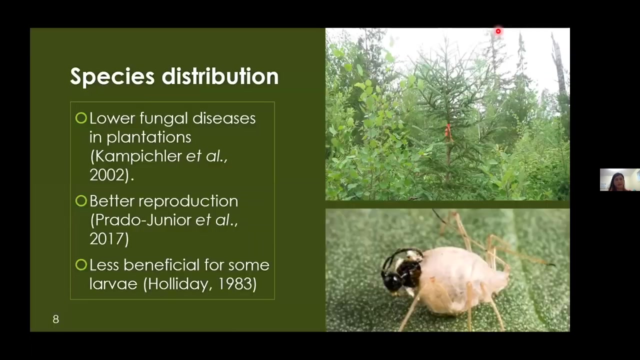 so for what again? um, we got more aphids and all jets within plantations and um less- well, actually more- larvae within mixed with forest. so what could this mean? um this, as i kind of like mentioned before, uh could be due well, because of um one of the different factors. so uh, studies have shown that uh between like um open areas. 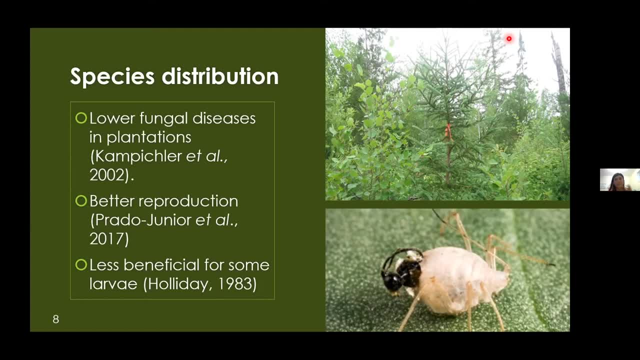 and forest areas. there is lower fungal diseases in these open areas for aphids, which could be a reason why they're in higher abundance. and there is also. they're like aphids are positively affected by heat. they tend to like have a better reproduction. they have several generations per year. 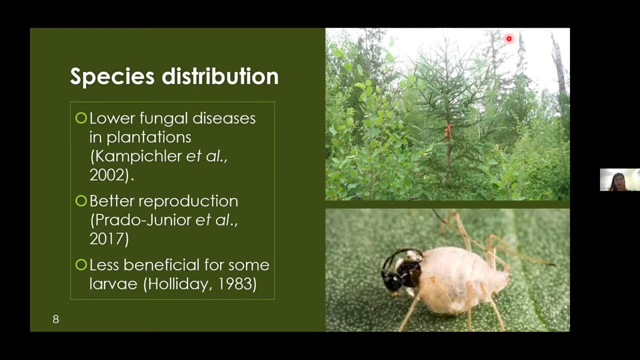 that's also a reason why they are increasing in these locations. however, for the larvae like, there's studies showing that geometridae are negatively affected, which is a group of larvae are negatively affected by like higher like temperatures overall. but there are other groups which are like, i'll just say, like nocturne, day uh, which are kind of like like the white mask. 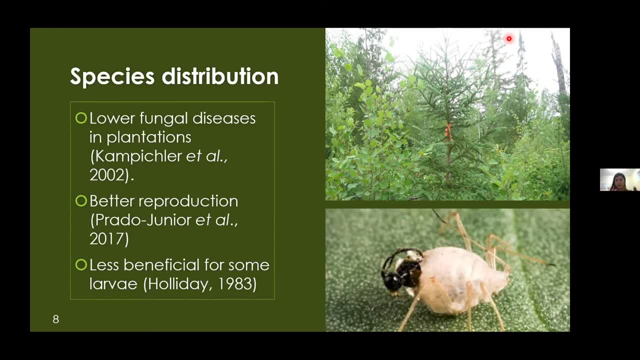 uh marked, uh tasok moth and the gypsy moth are kind of in that group also that seem to do better in warmer climates. so there's still a lot of like debate, uh, for this, the like, um, like what, whether or not, like each specific, how each specific level will react. but it seems a bit like. 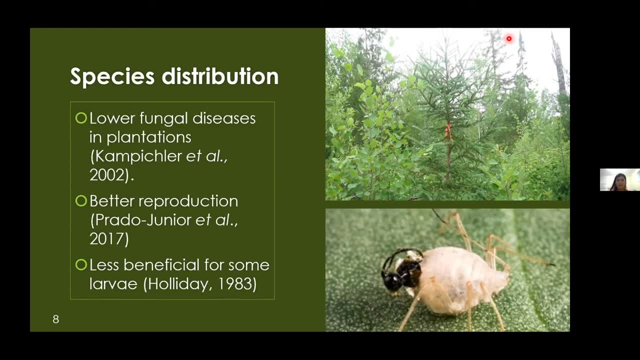 range that there is a really low quantity of like these, like wasp larvae and butterfly moth larvae in open areas. it could be two other factors. so we want to understand more about this system. so we're: what we're going to do in the summer is we're going to go look at the predators that are. 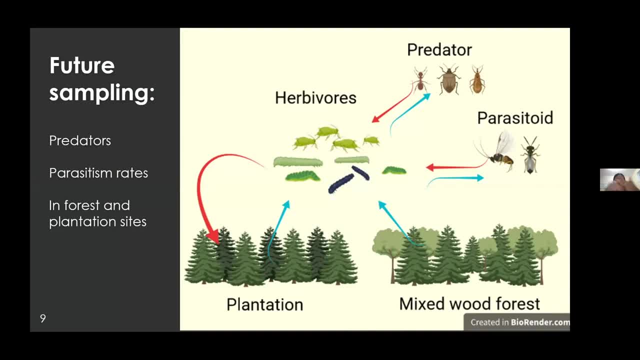 within both of these areas. like i mentioned, ants, there's like a bunch of stink bugs and other um bugs and we'll see if like there's any like uh differences between these two, like mixed food and plantations, and because of this kind of um threat of um the of the uh spruce butt worm, we're also 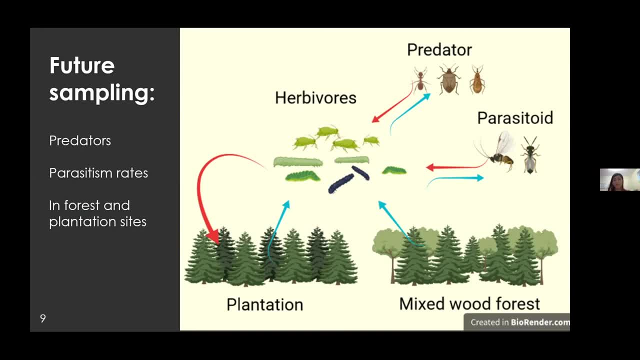 gonna be looking at levels of parasitism, so of wasps and flies. so flies and wasps tend to attack the insect larvae, while wasps are usually the ones that attack um the aphids, and see if there's correlation between these two locations. so, and yeah, it's also possible that, um, because there's higher levels of aphids, maybe that attracts. 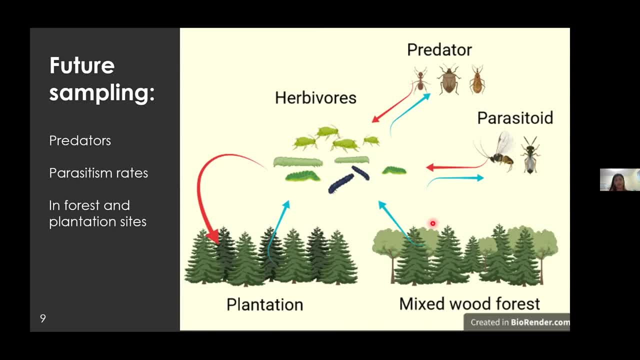 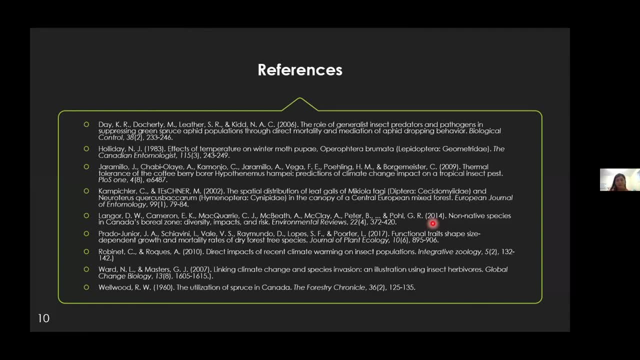 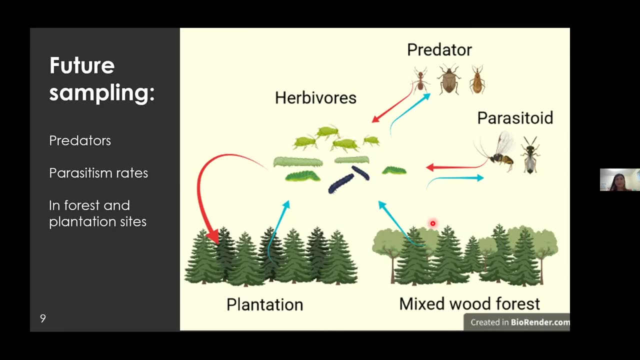 like more ants and that could also decrease other pesticides, but we'll see. so, um, i like to think, um, like, um. these are my references, but i'd like to thank everyone that helped me for this project. so i want to thank my colleagues and friends, and my colleagues in the lab as well, who helped me. 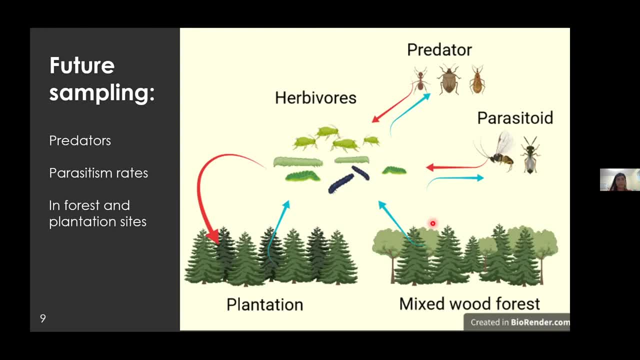 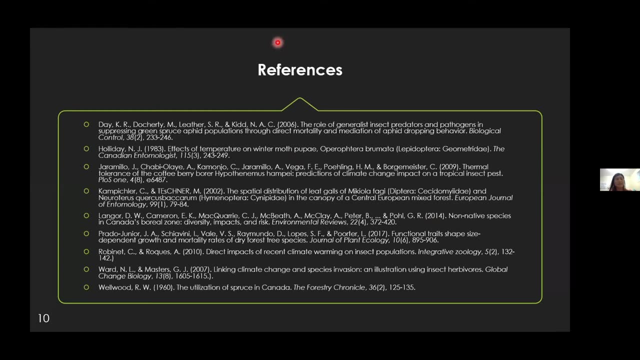 um, i so i want to thank everyone from eucat, um, my um, people from feralde that helped me a lot when i was up there and the people that helped me sampling as well when i was in up in the forest. so that's my presentation and hopefully this summer is gonna go well and less. uh negative, uh negative. 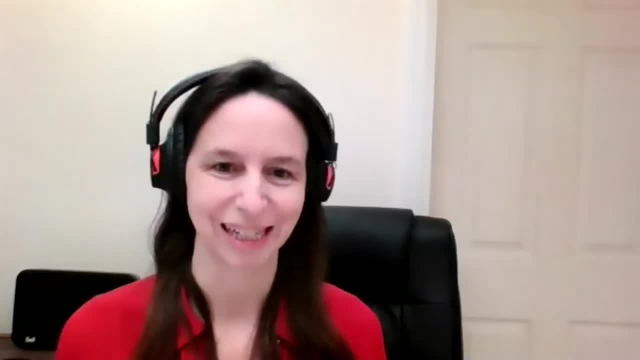 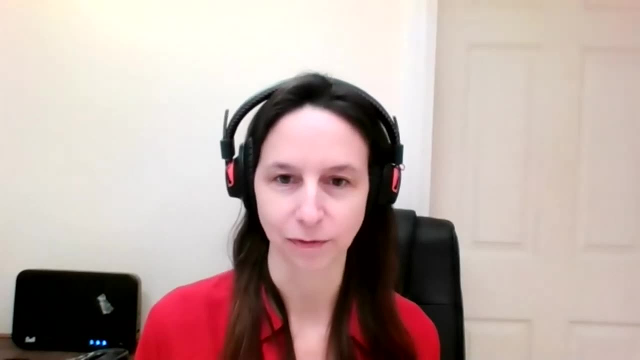 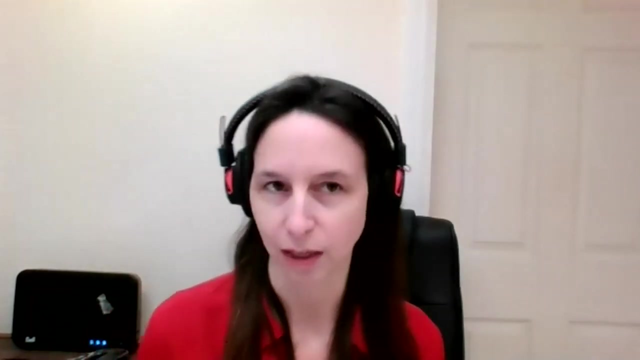 effects from covet. yeah, all right, thank you. thank you so much, pamela, for your wonderful presentation, specifically for Pamela. before we move on to more general questions, questions that were left over from the last talks, anybody okay? well, I have a question. are you thinking of doing anything? 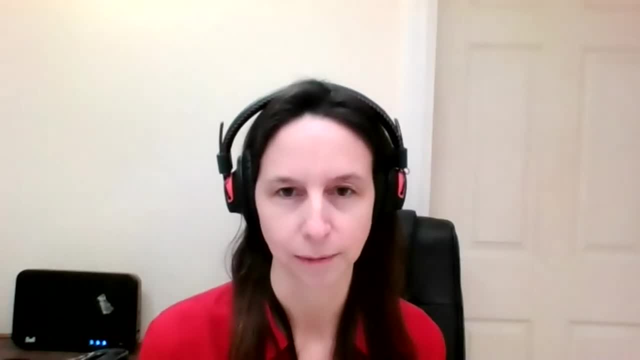 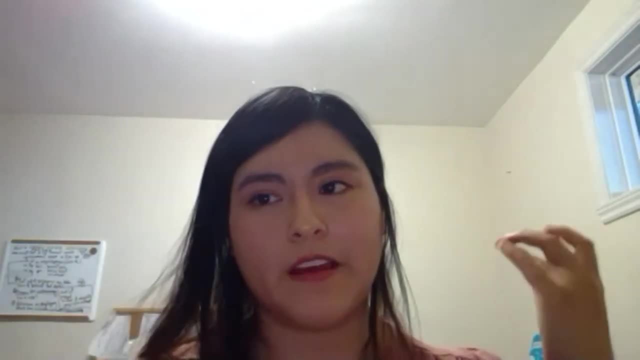 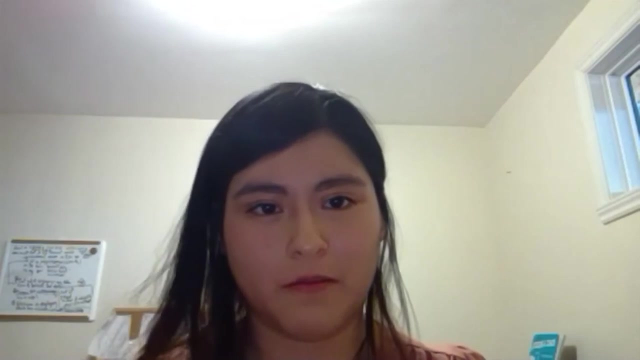 different this summer or just repeating to get more, more samples, yeah. so yeah, I mentioned I'm gonna get samples from like predators and parasitoids and yeah, I'm gonna, because I only managed to sample in like the late fall. I didn't get like the whole population early and and late. summer. so I'll try to get that as well this year. so you would expect to have greater diversity of species if you have a longer season gonna be different because depending on the year- not the year- depending on the month- you'll have different larvas emergence. so some of them emerge later on the year or they're very like early in the year. they might be very small and there's a lot of like more like bud worms. well, yeah, they're that sometimes will like take flight in June and July. we went like in July and August. so, yeah, I think, diversity, hopefully, and there to have something that isn't. 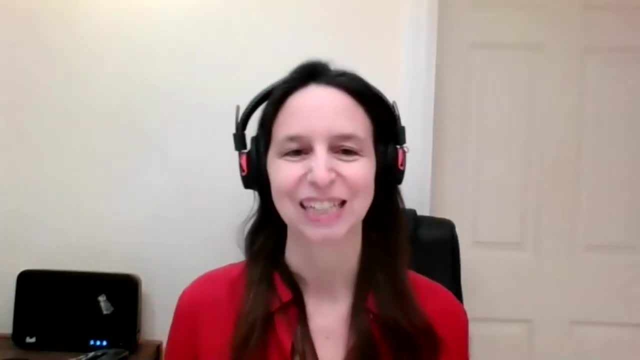 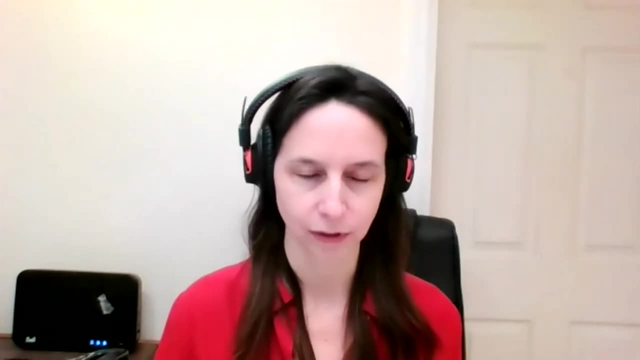 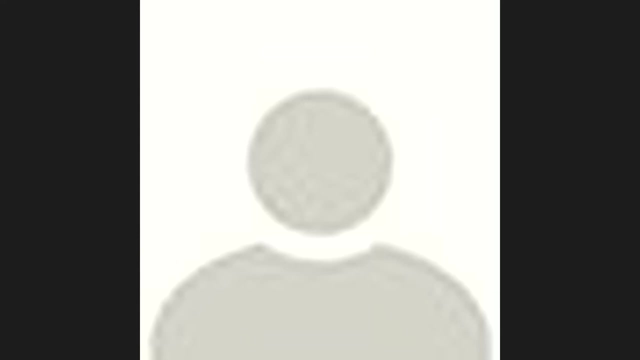 one. so, yes, absolutely good point. okay, I do have a hand raised in the audience, Kim. do you want to? I think you can unmute yourself. yes, yes, I did so go right ahead. thanks, Pamela, I think that's really intriguing. I'm sorry I'm asking so many questions, but I'm just curious about what is your hypothesis for if there's an 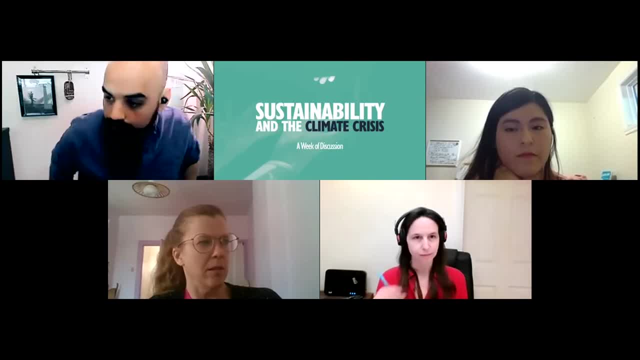 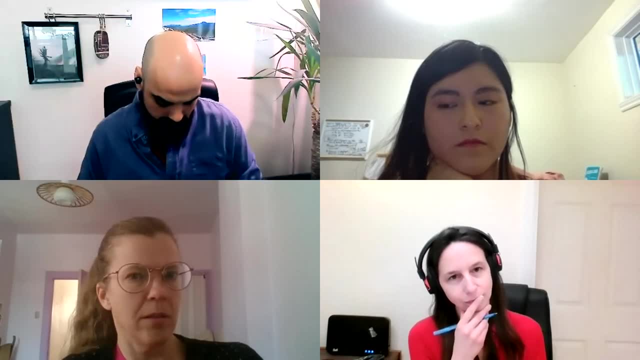 increase in aphids in the in the plantation area and yet no corresponding increase. that you would expect of their predators like that. so I'm just curious about what is your hypothesis about that? wasps is the? is the wasp itself somehow more fragile species? it's unable to adapt to the. 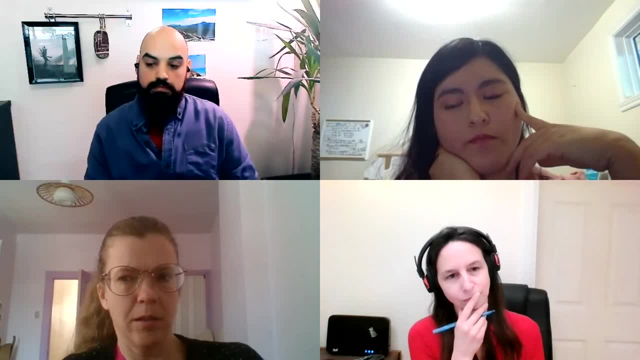 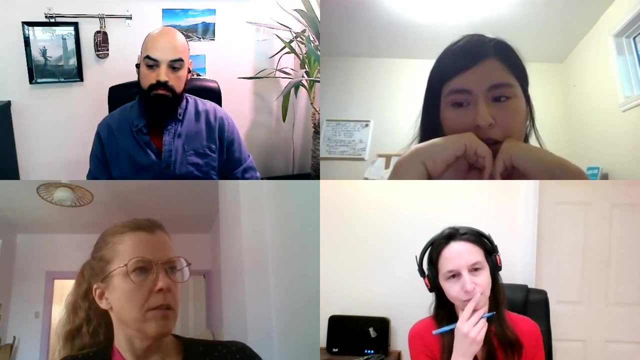 plantation environment or what's your, your theory about why there wouldn't be a corresponding increase in the in the predator insect populations to take care of that? like there's an imbalance somewhere. I'm just curious. yeah, it's possible that maybe, like these wasps, would be more colorly. 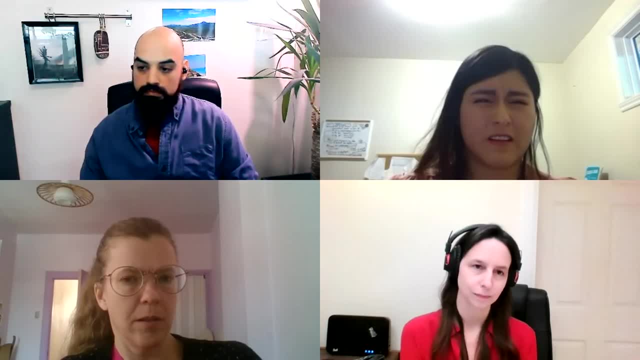 correlated with, like, their nesting areas, but the they do like kind of disperse, so it would be surprising to not find them. so I'm just curious about what is your hypothesis about that. so I'm just curious about what is your hypothesis about that. so I'm just curious about what is your hypothesis. 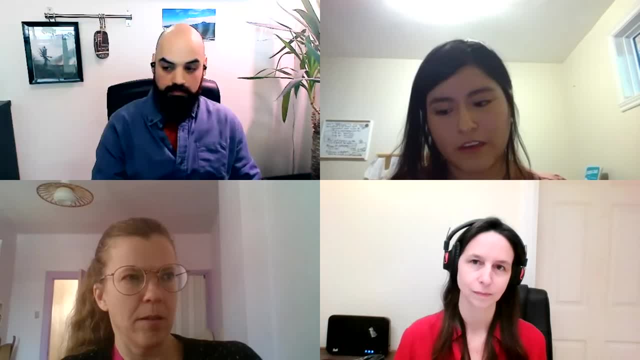 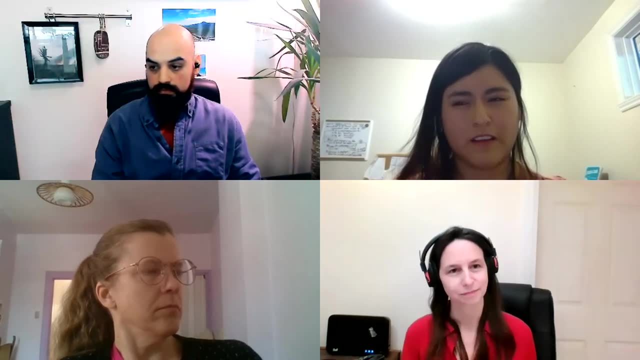 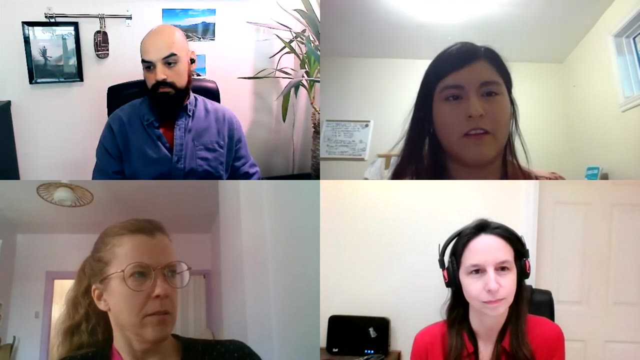 since it's also kind of an anthropogenic Lee disturbed location, like again it they just might not like right like dispersed there, but I know that like, for example, and this is the case a lot in like like cities or urban areas where there's less like parasitoids, but it would be surprising. 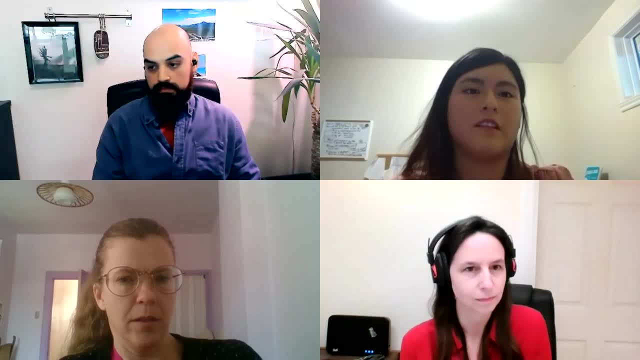 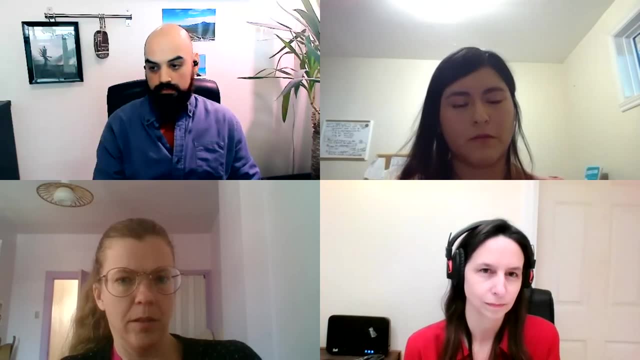 for me to see that in plantations, because, and like, if you're in a city, it's gonna- it's obviously it's a lot more fragmented and plantations is just an open area and they're not that super big. but yeah, we'll see. 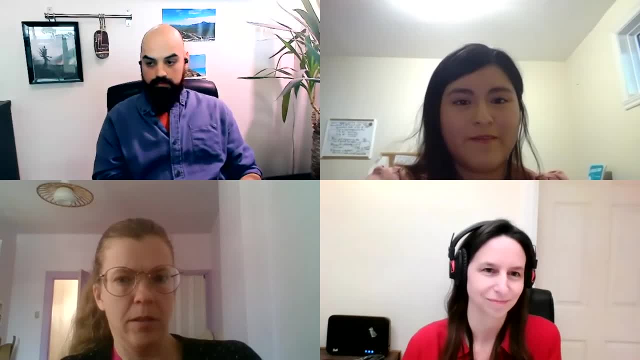 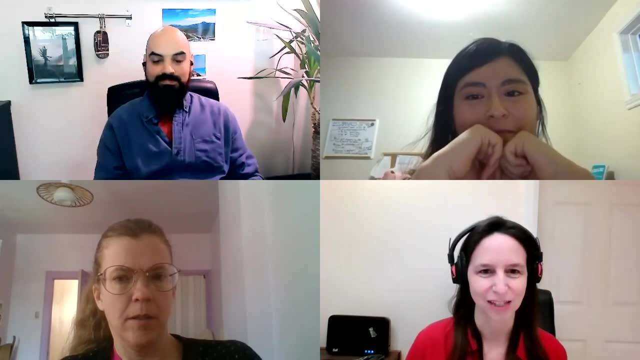 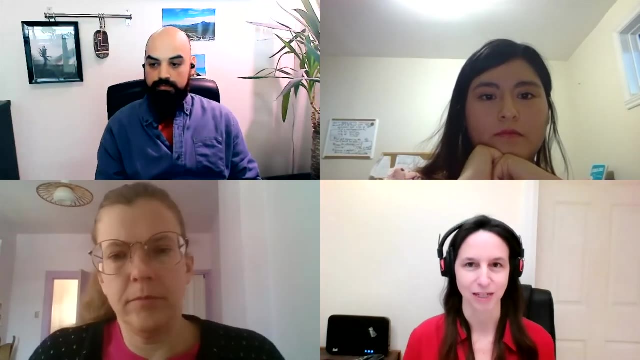 It would be very surprising. We'll have to listen to your next talk when you've done more sampling Just next year. Does anybody have any other questions specifically for Pamela? Otherwise, I'll move along. Okay, we did have a question left unanswered. 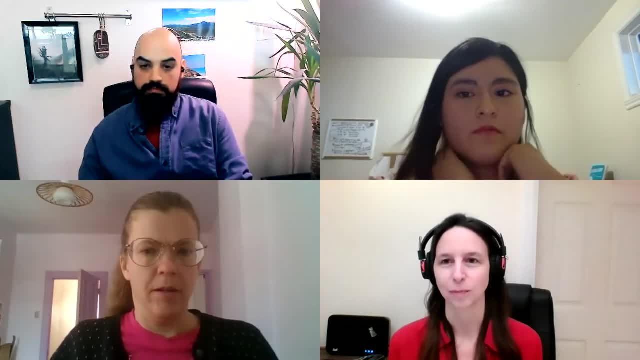 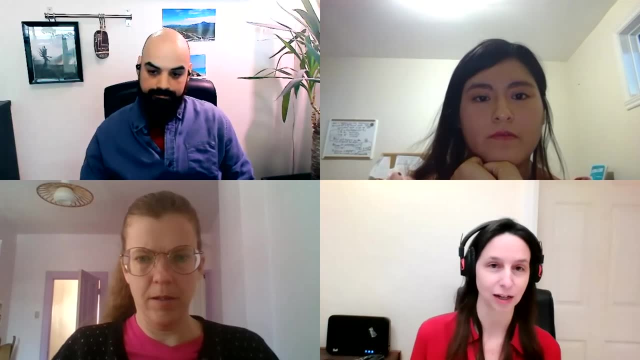 because we ran out of time at the end of Javier's talk from Carly. She has a question about scaling results With agriculture. we often think about land sparing versus land sharing at the landscape scale. I guess you can explain that if you'd like. 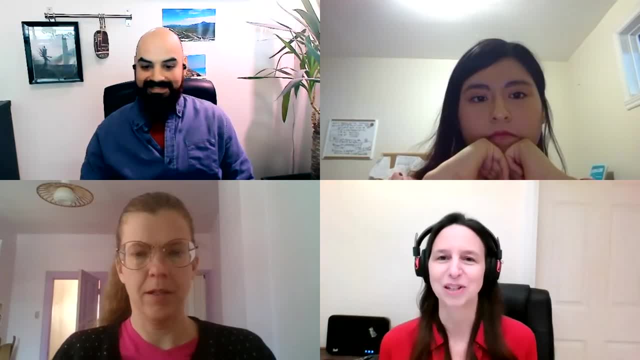 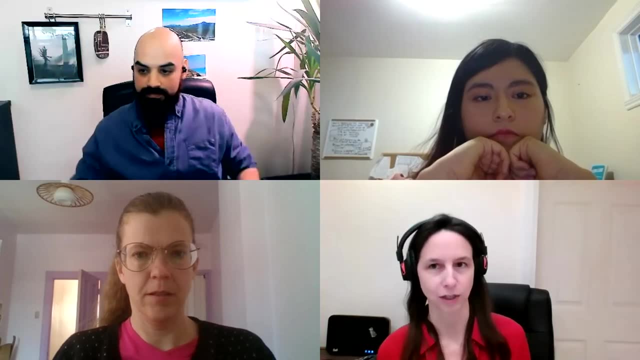 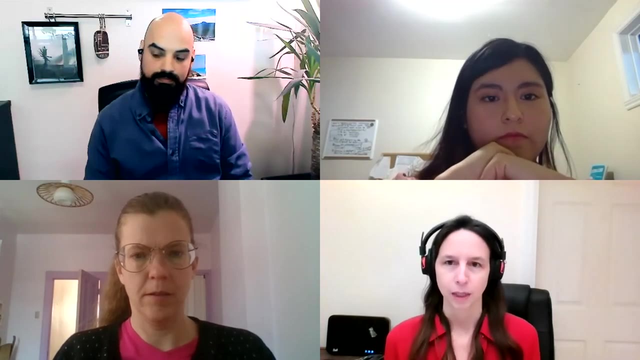 So let me go into my professor mode. You can do that. Do we focus on intensive agriculture and thus sparing more space for biodiversity, meaning that we would have conservation areas, or implying that we would have conservation areas to counterbalance that intensive agriculture Around these intensive fields? 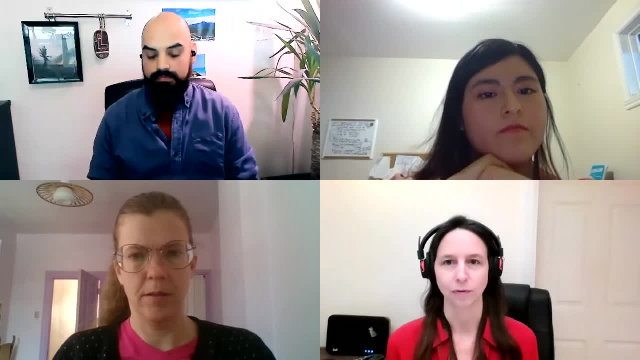 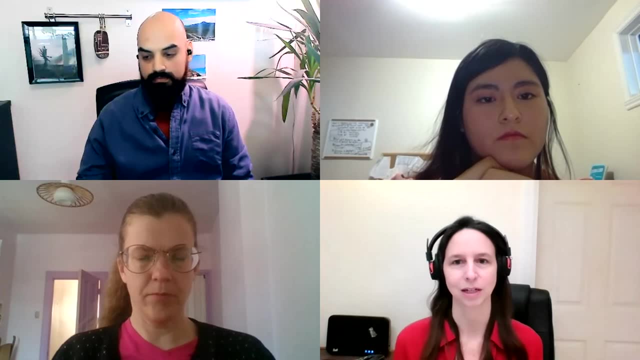 or do we share the space, like with shade grown coffee, where we aim for maintaining biodiversity within agricultural areas At the field scale? your work is showing that the sharing is good for any communities, but do you have any thoughts about whether your results would scale up? 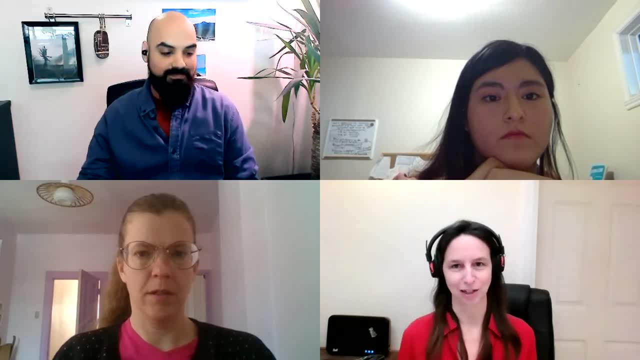 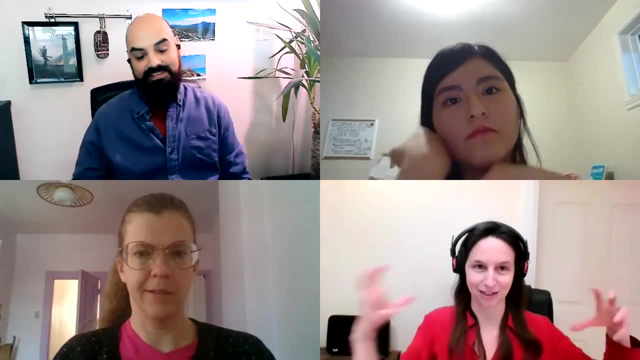 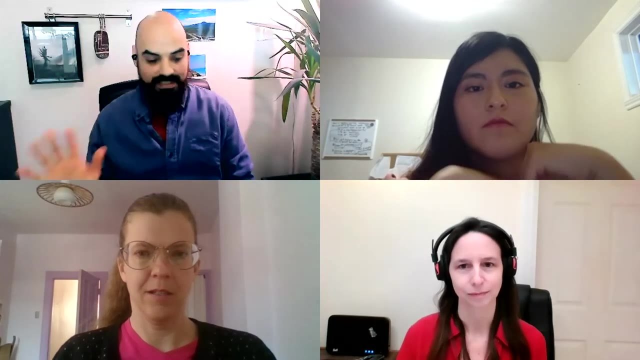 Great question, Carly: Is it feasible for all coffee plantations to be shade grown, in which case we might end up with the entire area in shade growing coffee plantations, as opposed to some coffee plantations and some natural habitat, Right? so this is absolutely a really great question, like it's very important because 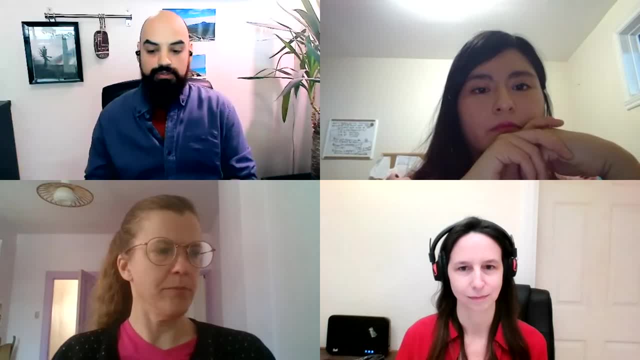 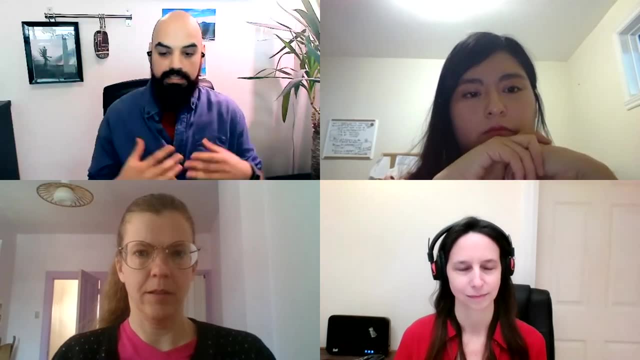 there are many things that you need to evaluate to be able to say this, because, yes, from the biodiversity point of view, it would seem that sharing it's the way to go to kind of like mitigate this biodiversity loss and other things. but you need to look at this from the perspective. of the farmers. because of shade growing, it may take some more resources to do in some cases, and not only that, it takes longer to grow, like the coffee can take a little bit longer, or rather the coffee berry. actually. you get a lot less yield, so there's a lot less production of. 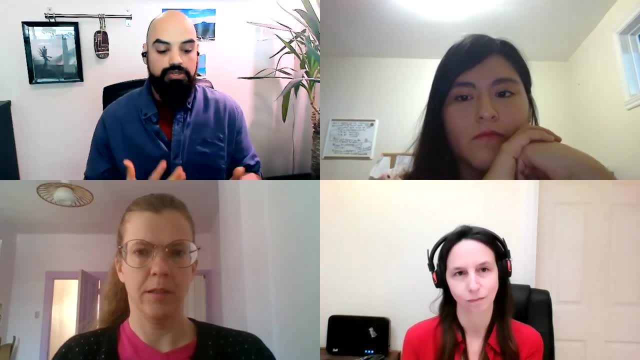 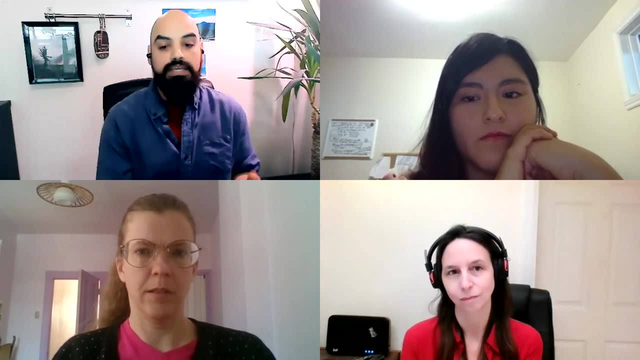 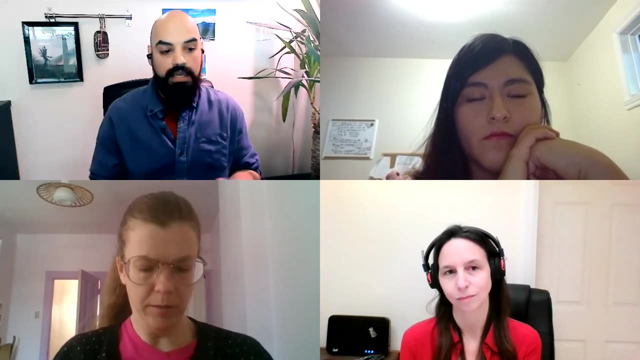 coffee, so the income for the. so you need to evaluate these: what type of trees you're going to use, what type of, in order to help them, because they see a more immediate, more immediate reward from doing intensive practices. so it's something that 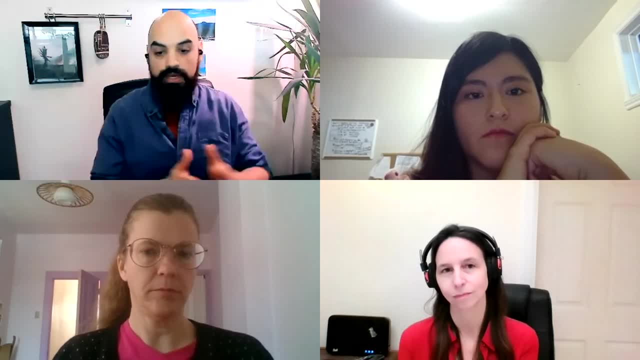 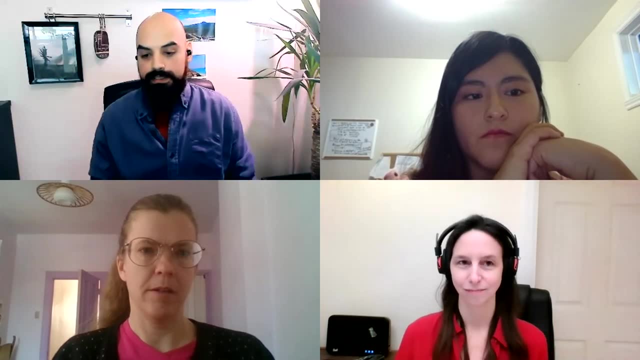 yes, from the biodiversity point of view, yes, sharing would be the way to go from at all scales. but then there's- there are other aspects that might be important as well. I just want to follow up with that. so are there species that only exist in in the forest? that? 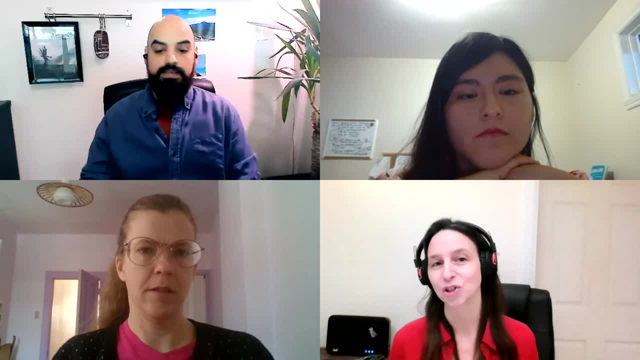 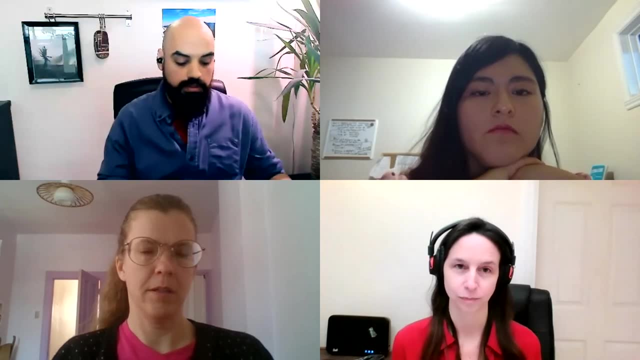 aren't in the forest, In the shade-grown coffee plantations? Yes, So wouldn't. wouldn't you lose those species if you went for an entire landscape of of sharing? So the thing is that you, you will lose a lot less than doing intensive practices, right? so 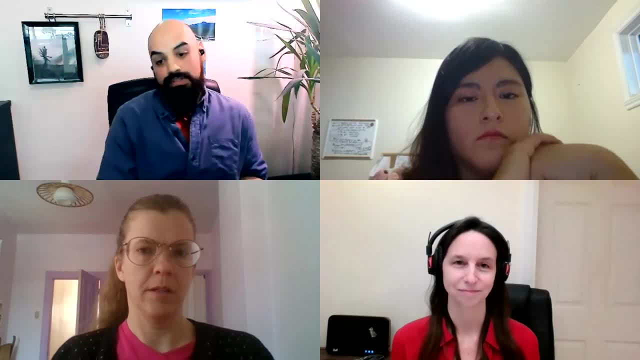 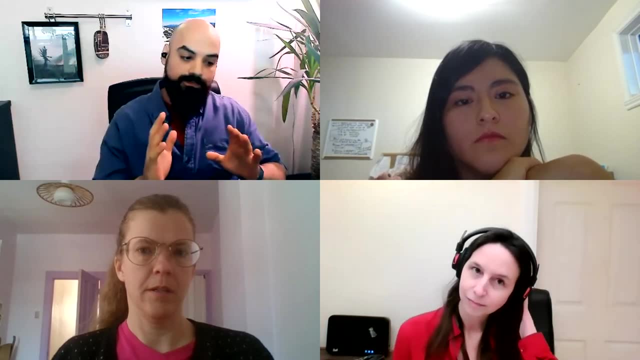 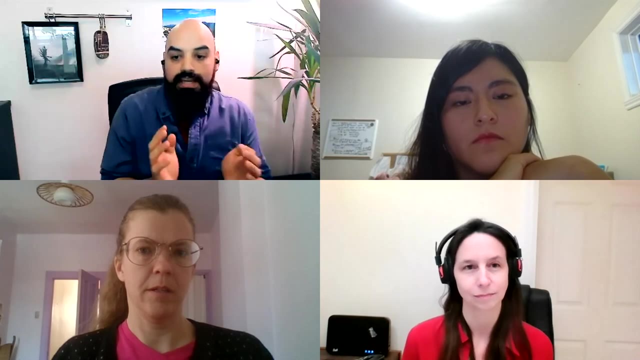 again, it's, it's a matter of evaluating the livelihoods of people still during these management practices, and so we would need to evaluate, integrate these, you know, biodiversity monitoring across multiple scales to see, you know, to mitigate as much as we can without impacting. 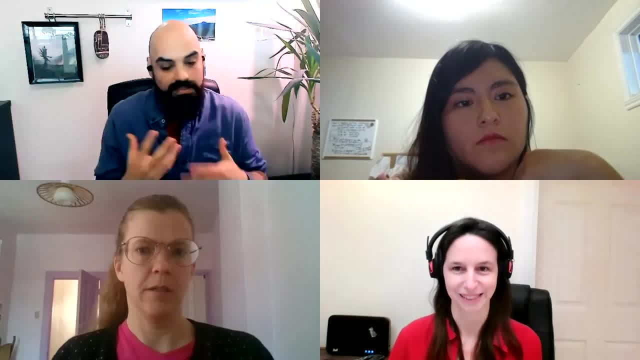 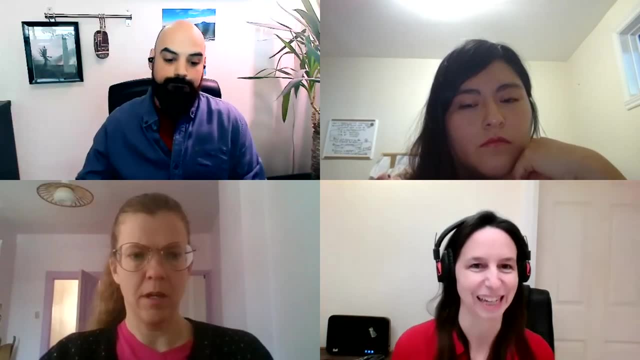 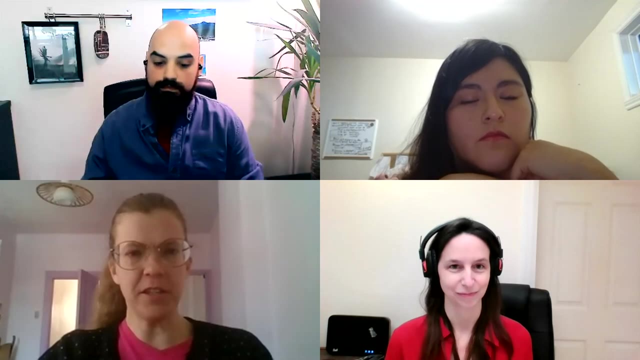 the livelihoods of people as much. so it's it's it's a very, you know, complex thing. Okay, thank you, I can. I can maybe add to that, just just to say that this debate happens in lots of different contexts. so I mean Forestry, Quebec. 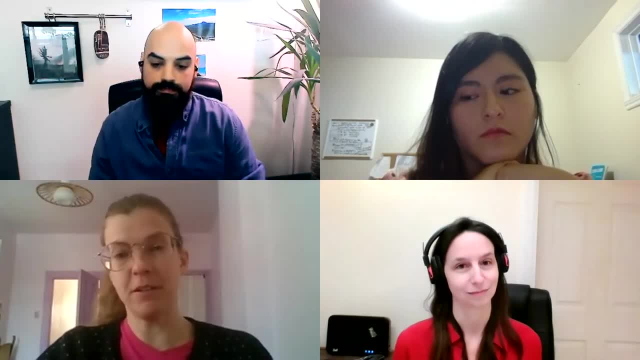 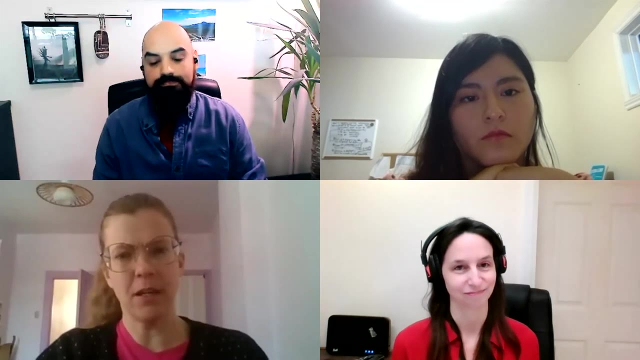 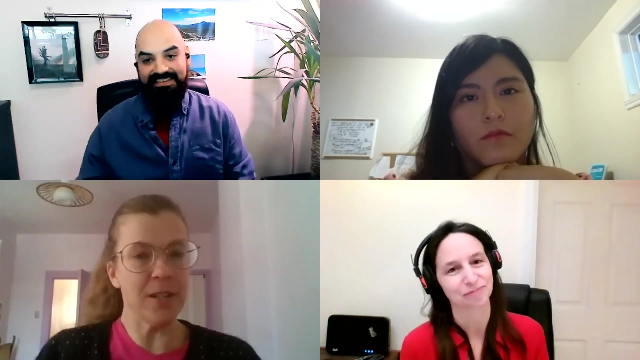 there's the same question of: do we go for small amounts of fast growing plantations or do we try and manage huge areas for maybe less wood production but more biodiversity conservation? so it's it's a huge debate and I think the answer probably is different for different systems. like, I don't think you can do shade-grown tomatoes. so you know, in terms of agriculture, some crops you can, some crops you can't, and yeah, 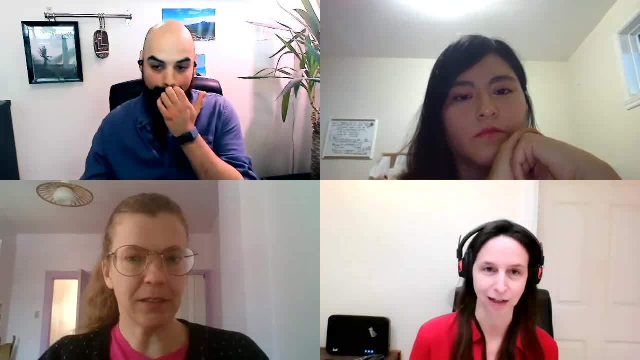 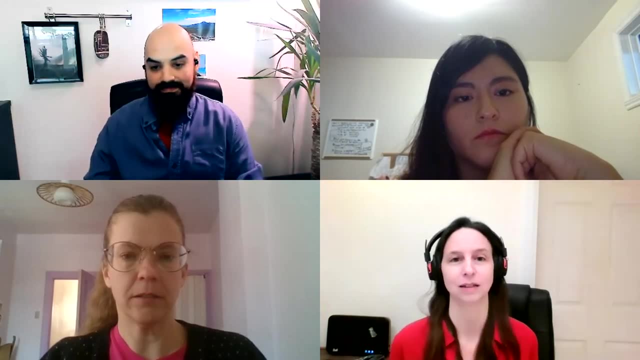 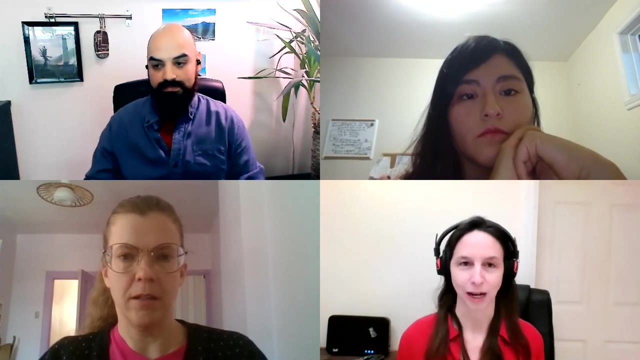 Right, But it's the same question as partial cutting for seeds. I think the answer to this is clear cutting, which was my master's thesis. right, and I concluded that clear cutting. you know that partial cutting didn't necessarily pay off, because it required twice as many roads and you would lose species of birds, in my case, from partial cuts that then you wouldn't have anywhere because you would have no in touch forest as a result of partial cutting everywhere. 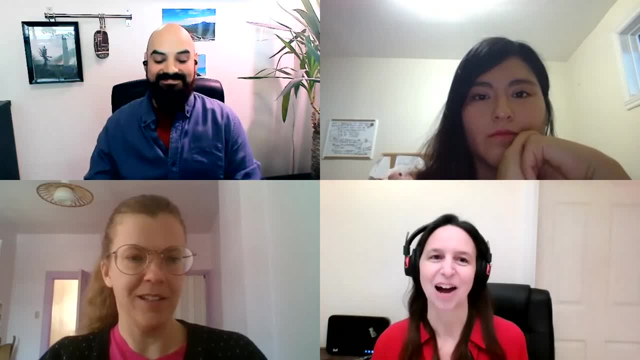 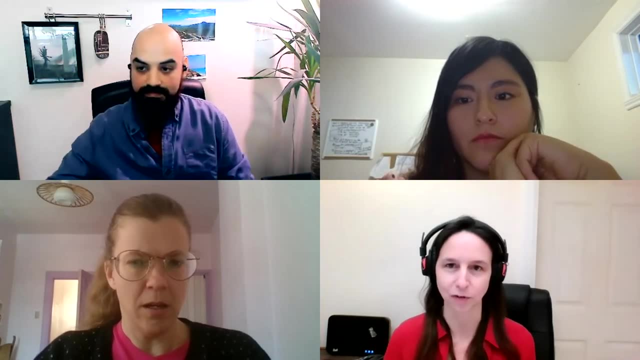 Anyways, that's my work. I have another question: What are some examples of mitigation for insect population control to prevent crossing the eruptive threshold? I think this one is more for you, Anna Wait, could you read that again, sorry? 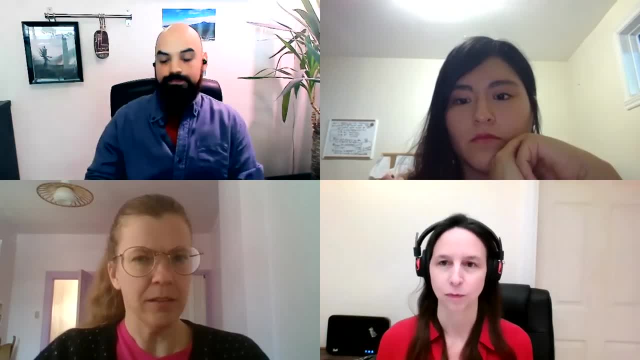 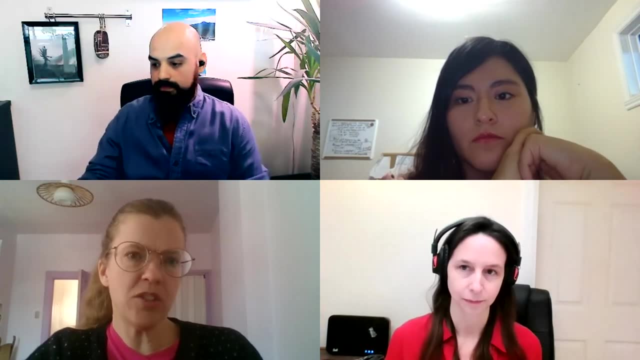 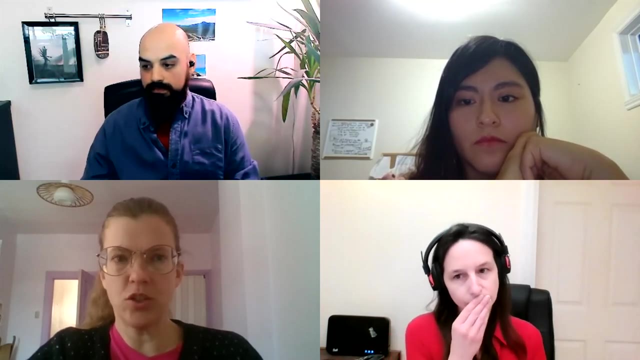 What are some examples of mitigation for insect population control to prevent crossing the eruptive thresholds? What should we be doing? Yeah, so so one question there, one big one, has to do with forest composition and the extent to which which trees you have on the landscape influences what insects to get. 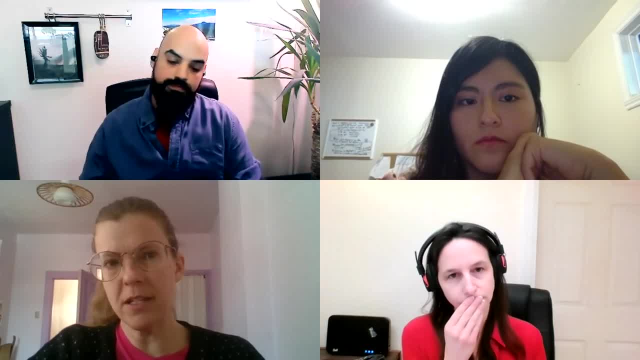 So, for example, for the mountain pine beetle, one of the things that has been brought up is: okay, the last you know. in the past you know it's been really popularly that the tree has to be cut off, Right. 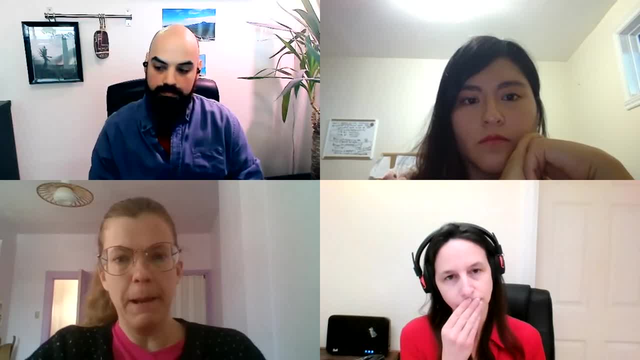 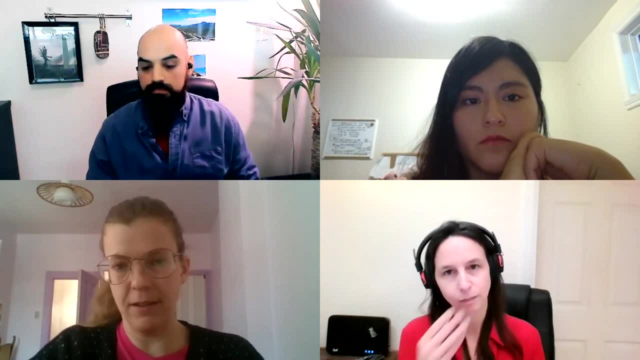 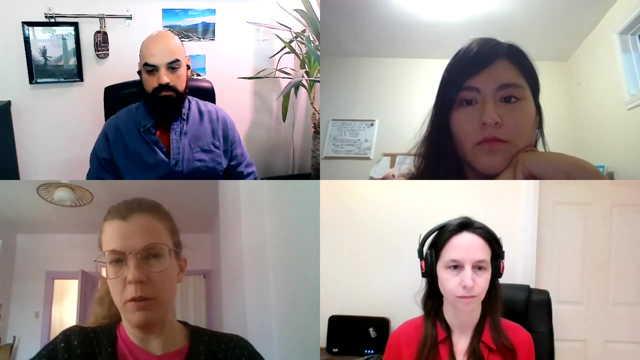 our lifetimes, lodgepole pine has been the dominant tree, but lodgepole pine is also very economically valuable and it has been planted. if we had maybe planted different trees on the landscape, we would have had less mountain pine beetle um so. so the mix of forest composition is is one. 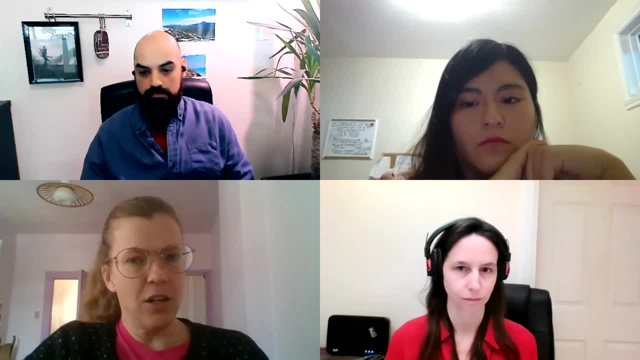 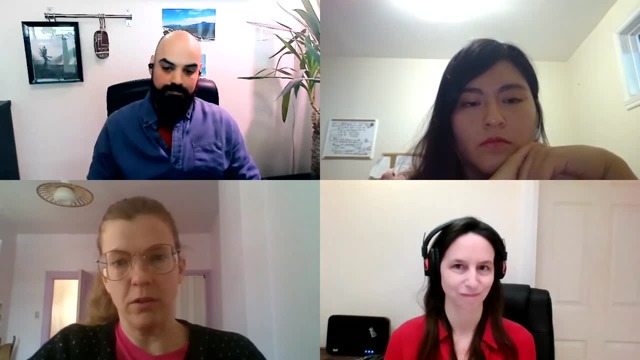 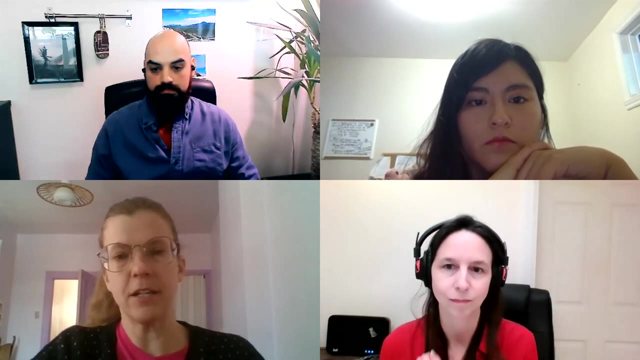 big question, of course, that's, you know, if we're going to put that as a management practice. that's very slow, um. and then the other one is just direct control of basically using insecticides, usually, um, to kill insects and to hope to bring the outbreak under control, and that too is debatable. because some, if you do it early it might work, if you do it late, it's. it's not going to work and you're just going to be, you know, poisoning the landscape and wasting your money for nothing. yes, absolutely okay. i have another question, uh, from yakin: what if those ants provide beneficial ecosystem services like pest control? 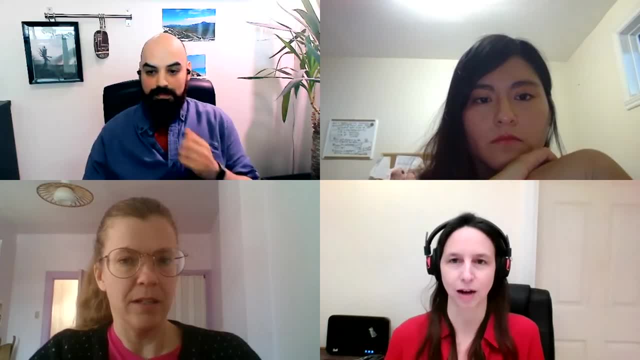 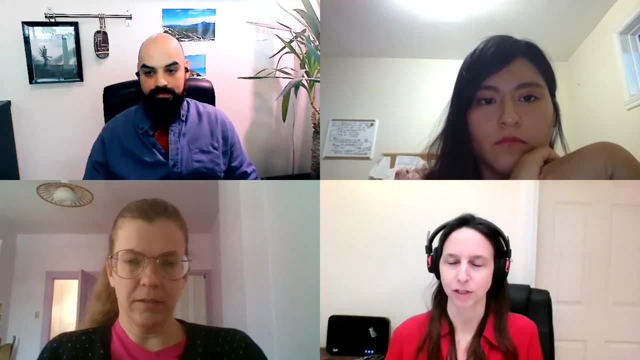 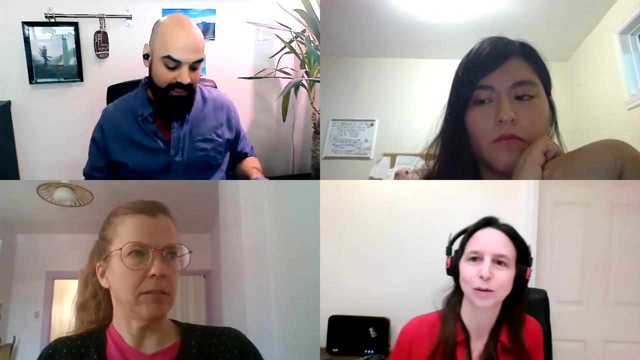 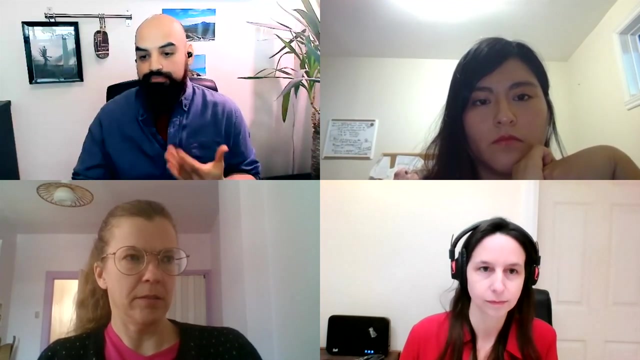 why would coffee farmers not want to grow coffee in the shade? how can they get to sufficient profits in the sunny areas? do they use pesticides then? but what will? but that will have additional effects, now, right, so so definitely, um, uh, you're gonna lose the these, uh, predatory ants that can help, um, you know, in the sun-grown coffee, you definitely lose. 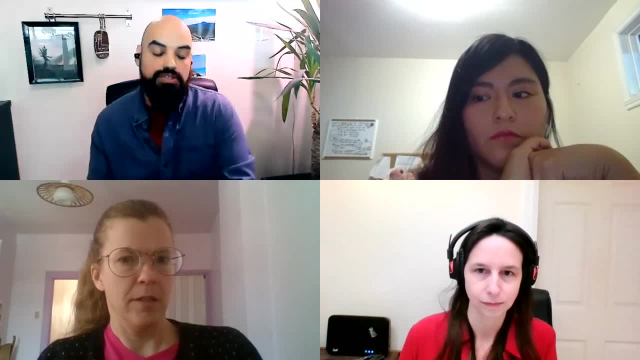 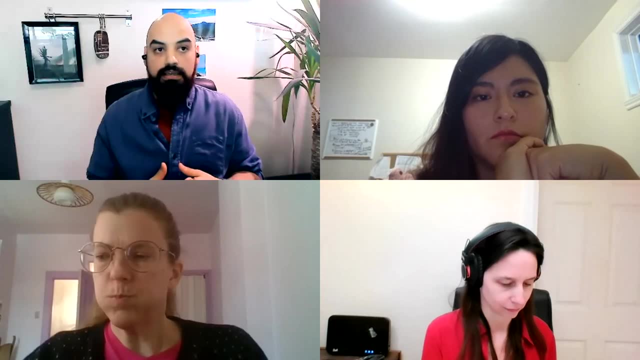 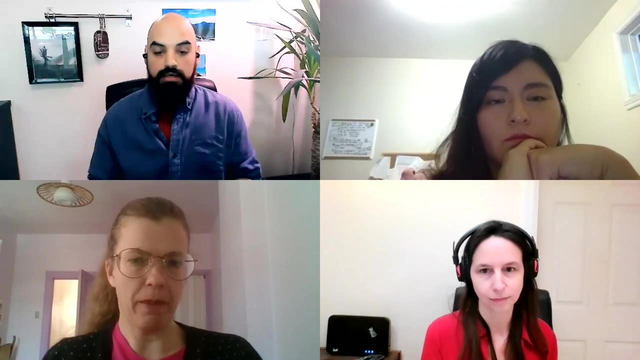 that's the major. one of the major uh portions of ants that you lose is the, the predatory ants, um, but the thing is that a lot of coffee farmers they don't see ants as beneficial at all. so we first need to work on educating uh farmers that ants can be beneficial and to show 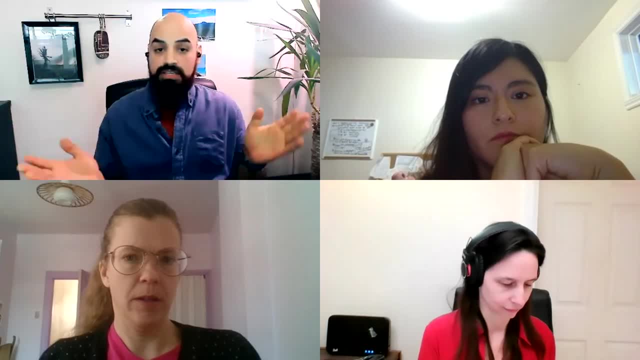 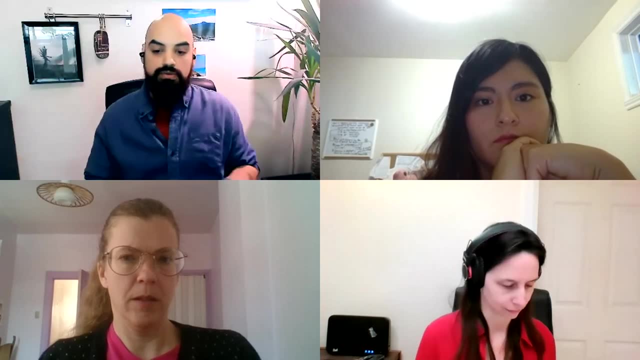 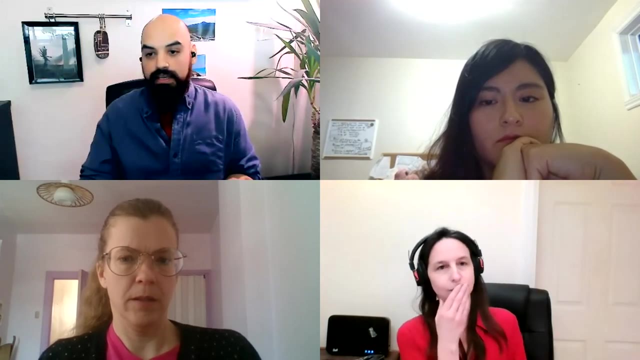 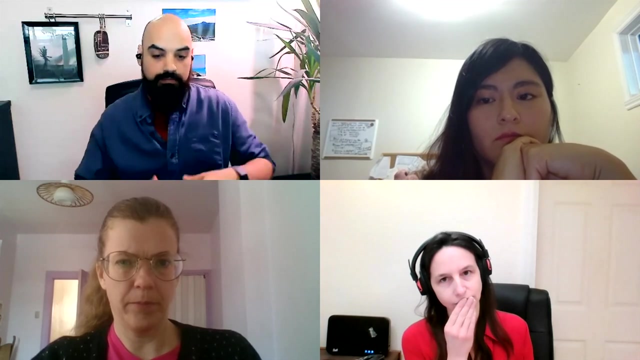 them how that they're beneficial. um, so we first need to work on educating afterwards. bento, humans can do the work. uh, potatoes can have weer smart phones, uh, that are. you know that they can be beneficial because they see them as pests, so they're gonna remove them anyways. and then, uh, in sun-grown coffees you turn sufficient profits because you get- uh, you get- more yield. um, it's a lower quality coffee, like some people can even taste the difference, um, and so it's. it's something that you get that profit out of, just the yield that you get from difference. and the pesticides, yes, you might net is the best one. you are a group who is currently ones that really need to cannot say just. 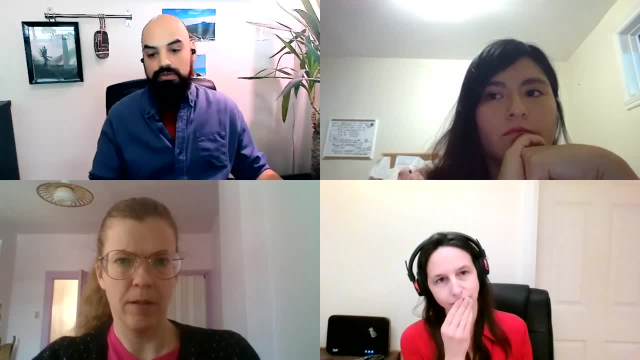 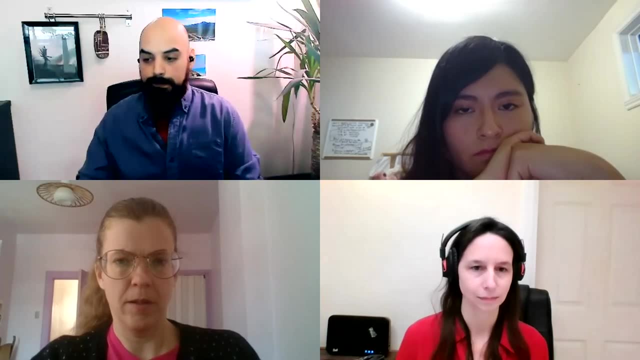 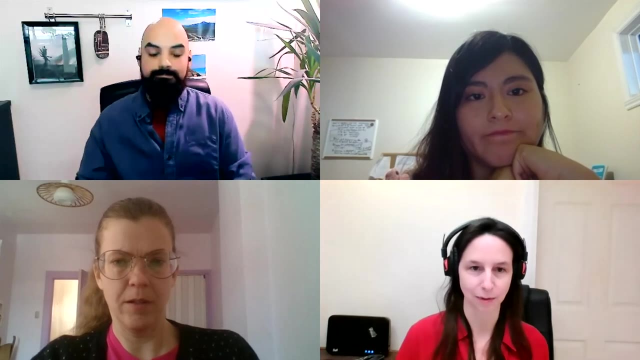 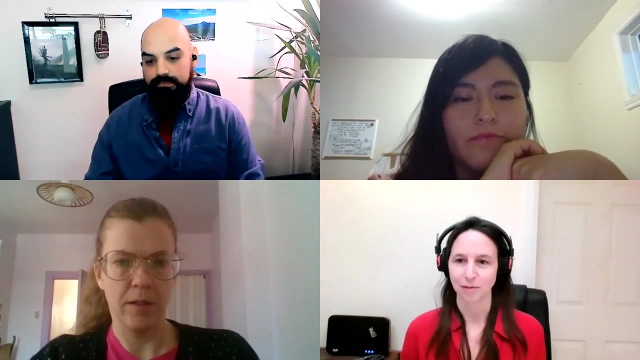 but do you get that? definitely use. some people use more in intensive practices, way more pesticides. everything under control. so, yeah, thank you, javier. we have gone over time already, for space has been very kind to host us for this long. we do have another panel starting at 2: 30 um. we will host, uh, damon matthews. 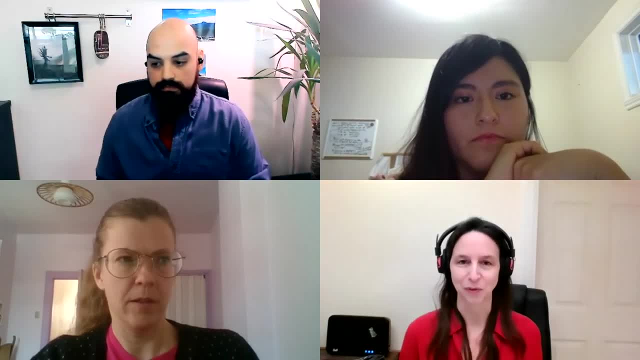 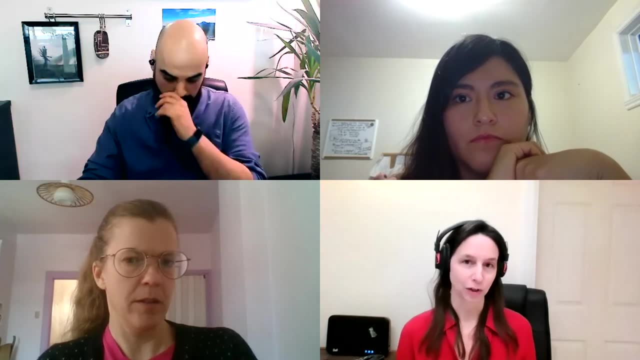 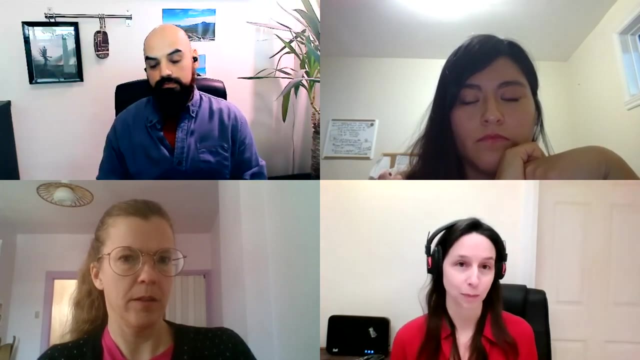 who will talk about the carbon budget, um, so that will be really interesting. and we also have later on today at 4: 15. we have anders bjorn and daniel horan greenford, who will talk about capitalism and science-based targets, so that will be another interesting one. we have event perfecto coming on. 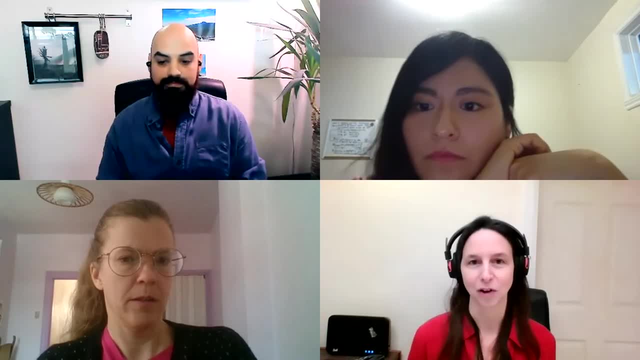 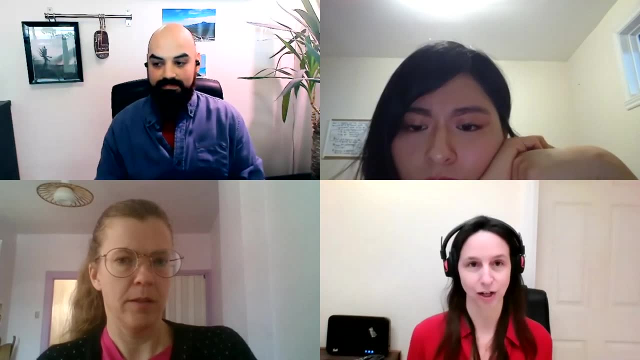 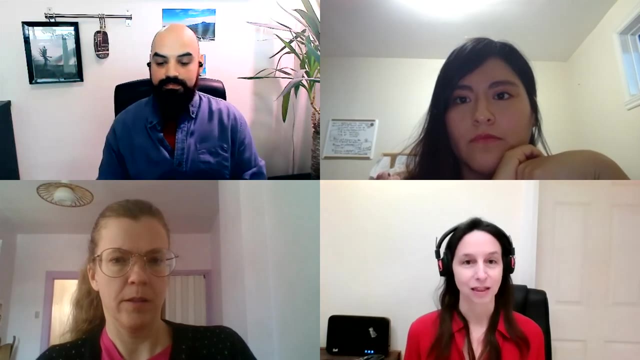 thursday afternoon. who will revisit? uh, the question of coffee, um, and so i welcome you back to discuss more at that time. we have events all week, so do check out the schedule where you found this event. there are four events every day, and with that, i would like to thank our